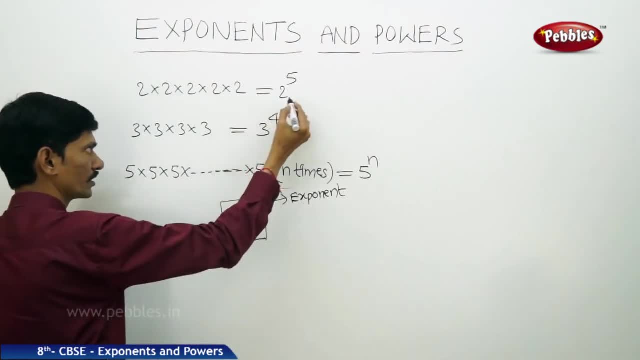 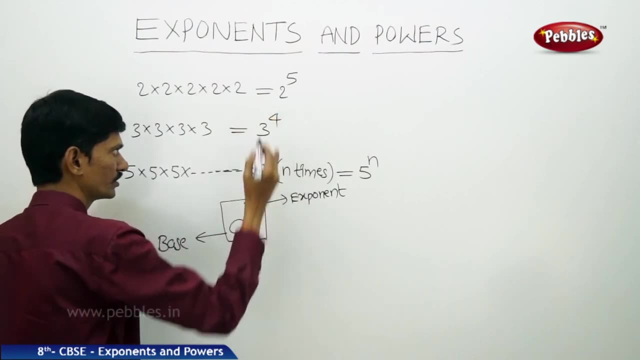 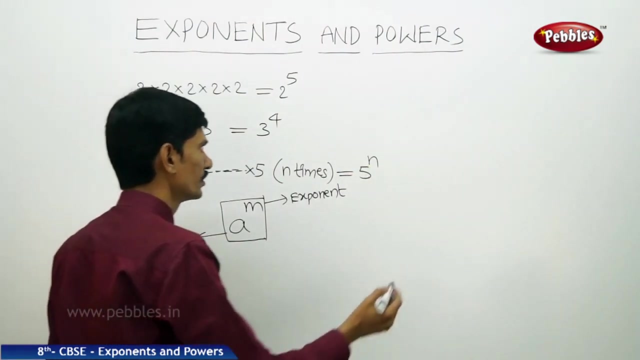 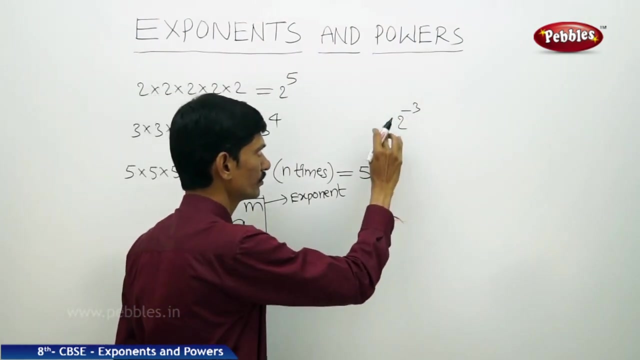 called the power. Now, in the first case here the base is 2 and the exponent is 5.. In the second case, 3 is the base and 4 is the exponent. In the third case, 5 is the base and n is the exponent. Now what is 2 power minus 3?? Means here base is 2 and the 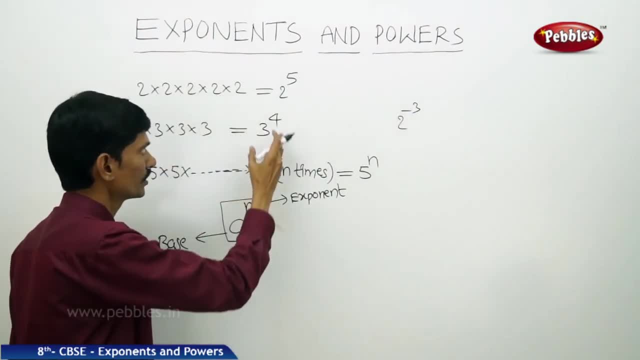 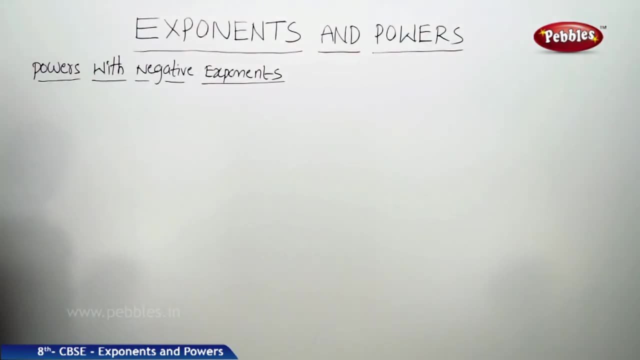 exponent is minus 3.. But here we have not seen the negative power. So if the negative power is given, then how to find its value? Now we will discuss powers with negative exponents. First we will take 10 power 3.. So 10 power 3 equals 10 into 10, into 10.. 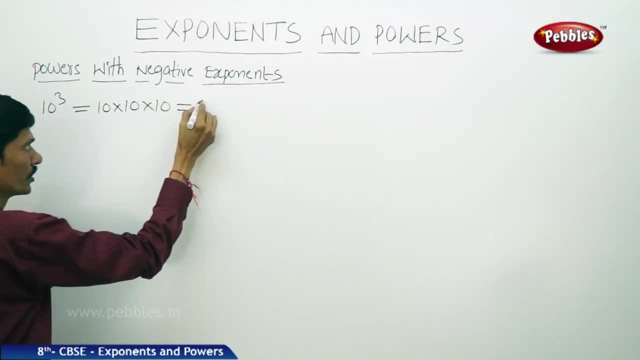 This equals to 10 times 100, 100 times 1000.. Now we will decrease the exponent by 1.. So will take 10 power 2, so this equals to 10 into 10, this equals to 100. so how you got. 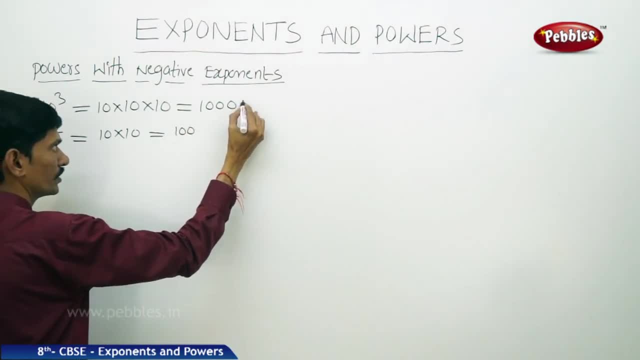 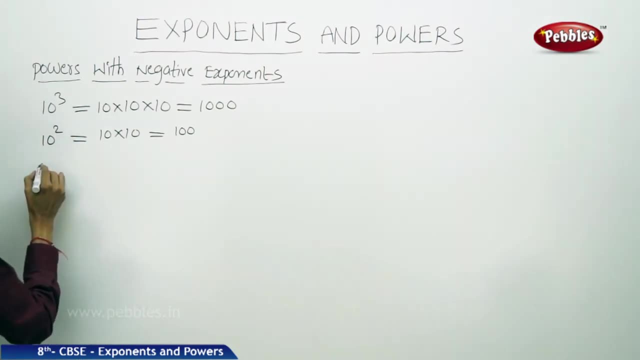 this 100 dividing the 1000 previous power, 1000 by 10. so if 1000 is divided by 10, we are getting 100. next you will find 10 to the power of 1. this equals to 10 itself. and next, 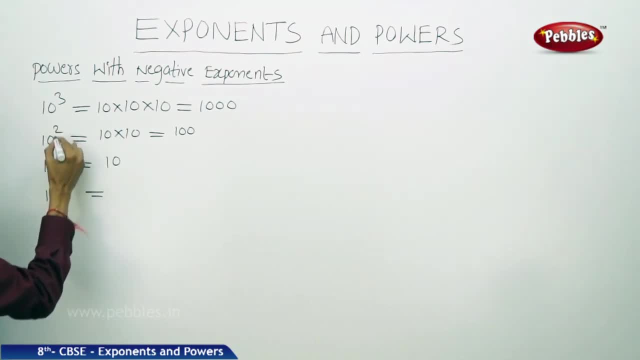 10 power 0, so we are decreasing the exponent by 1. so how we are getting the value of the 10 power 2? by dividing 1000 divided by 10. and again we are getting 10 here dividing its previous value by 10. so this, divided by 1000 divided by 10, is 100. 100 divided by 10. 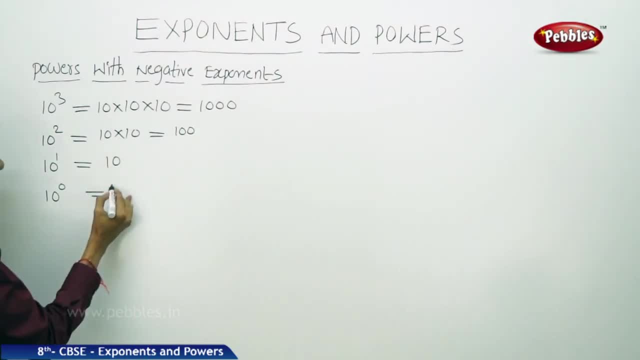 is 10. the next 10 power 0. again this 10 is divided by 10, this is 10.. equals to 1. next, when you decrease the exponents 3, 2, 1, 0, then next you have to take 10 to the. 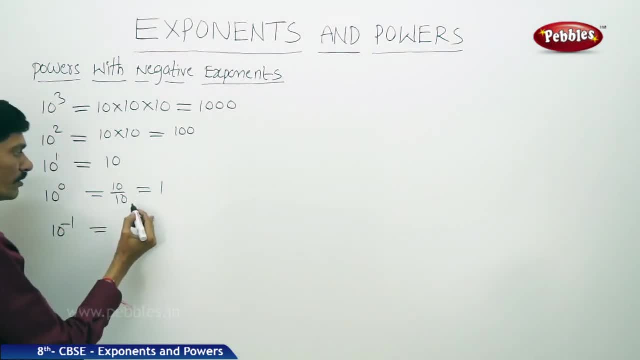 power of minus 1. this equals to, and divide the previous result by 10. so here, 1 divided by 10, this equals to 1 by 10. next 10 to the power of minus 2. this equals to, so 1 by 10. 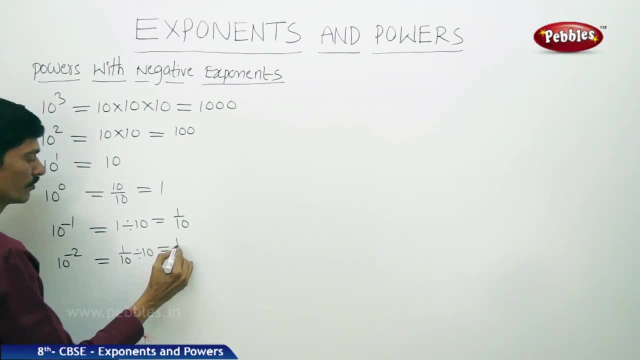 is divided by 10, this equals to 1 by 10. into again 1 by 10, this equals to 1. 1's are 1 by 10, 10, 10 square. now we will take 10 to the power of minus 3, so this equals to the previous. 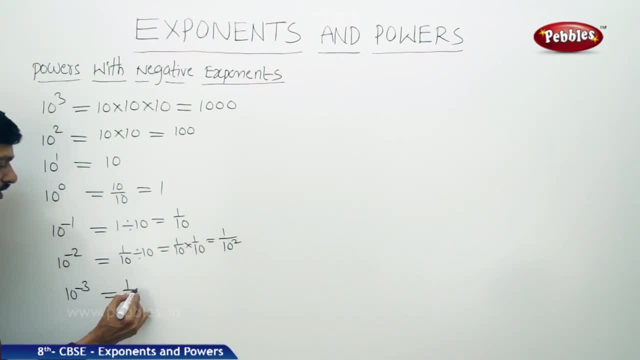 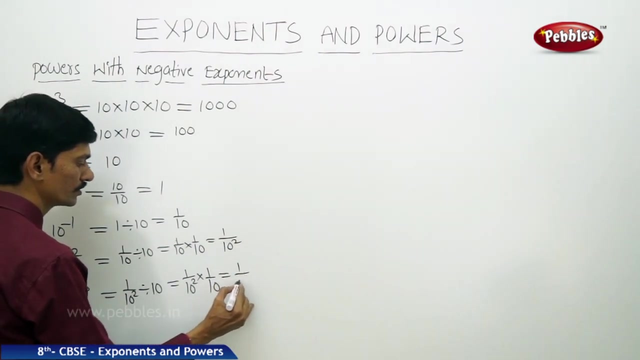 result is 1 by 10 square, so this must be divided by 10. so this equals to 1 by 10 square into the reciprocal of 10 to the power of minus 1.. is 1 by 10.. So this equals to 1. 1s are 1 by 10 square into 10, 10 cube. So when you 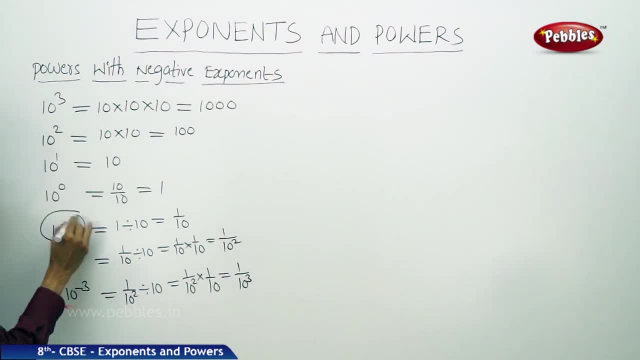 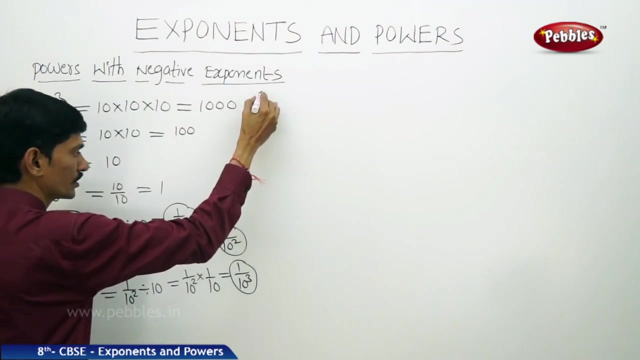 observe the negative powers: 10 power minus 1 is 1 by 10 power 1, and 10 power minus 2 is equals to 1 by 10 power 2, and 10 power minus 3 equals to 1 by 10 power 3.. Now let 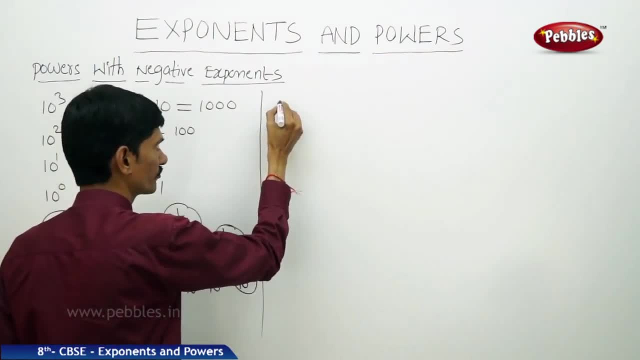 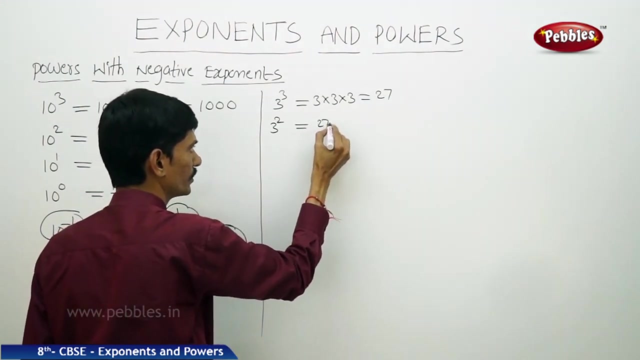 us take another example. When you take 3 cube, it is 3 into 3 into 3 equals to 27.. Next, 3 square is obtained by dividing the previous result by 3.. So 27 divided by 3, this equals. 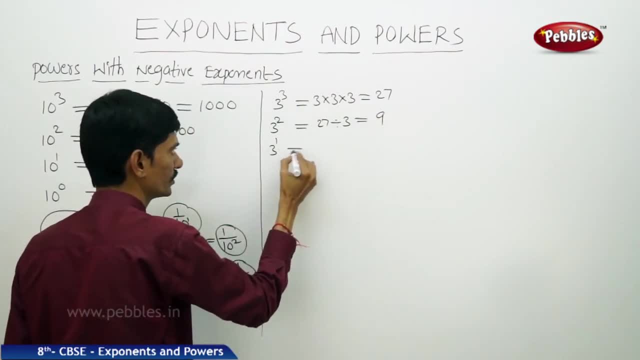 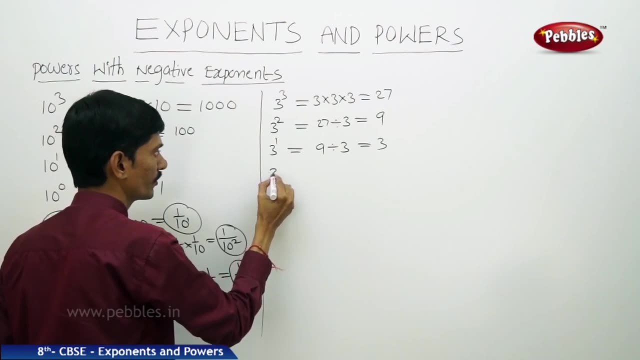 to 9.. Next, 3 to the power of 1,. this equals to, again, 9 divided by 3.. So this equals to 3.. Next 3, power 0. So in this case also, we are dividing, we are taking all the exponents by decreasing. 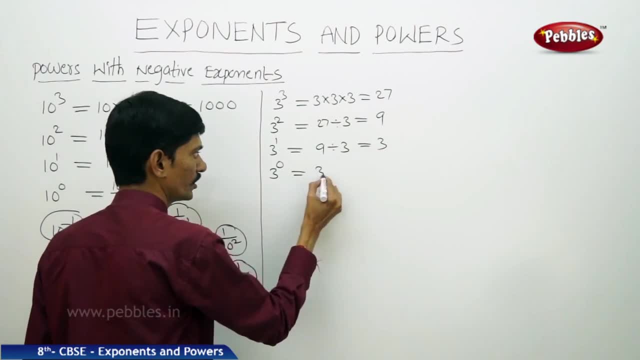 1.. So 3 power 0 equals to 3 divided by 3. This equals to 1.. Next, 3 power minus 1. So this equals to here the previous result: 1 divided by 3.. This equals to 1 by 3.. Next, 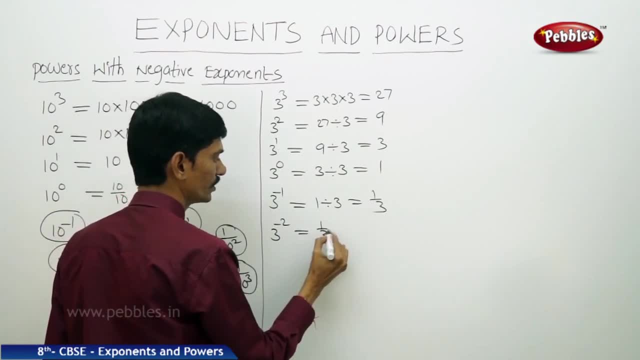 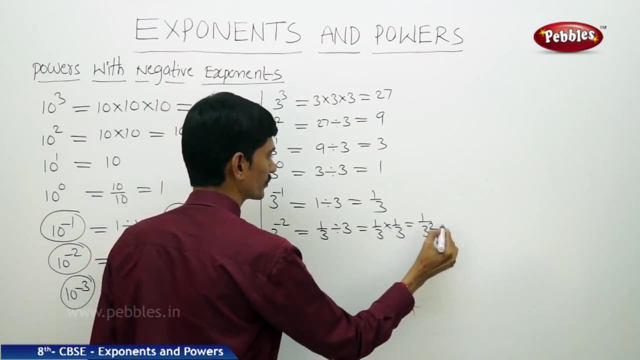 3 power minus 2 equals to 1 by 3 divided by 3.. equals to 1 by 3 into 1 by 3.. This equals to 1 by 3 square Now: 3 power minus 3 equals. 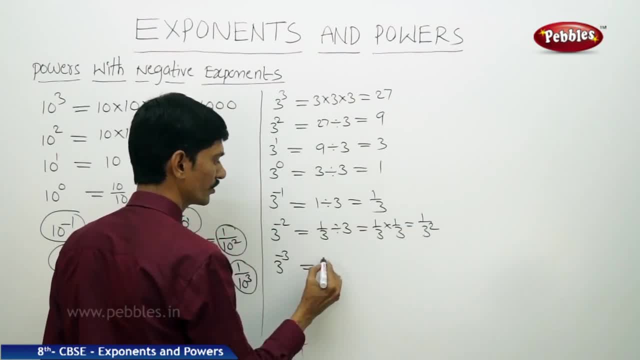 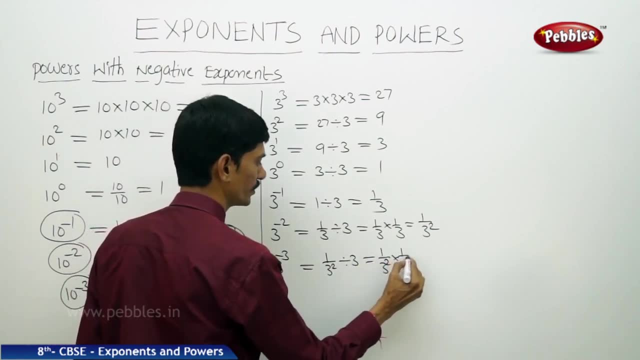 to the previous result is 1 by 3 square divided by 3.. So this equals to 1 by 3 square into 1 by 3.. So this equals to 1 by 3 cube. So here also we can observe that 3 to the power. 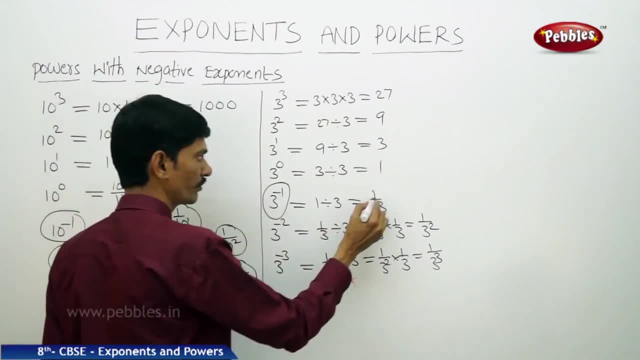 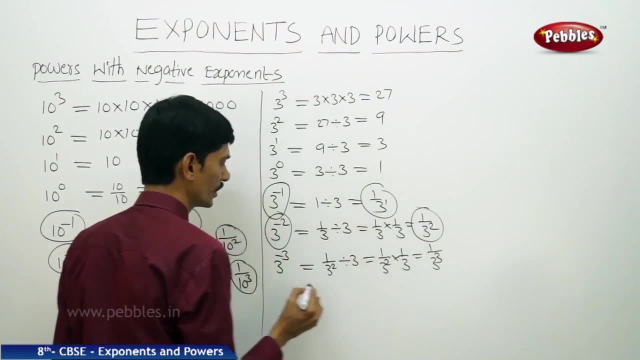 of negative power means: 3 to the power of minus 1 equals to 1 by 3 to the power of 1, and 3 to the power of minus 2 equals to 1 by 3 to the power of 2, and 3 to the power. 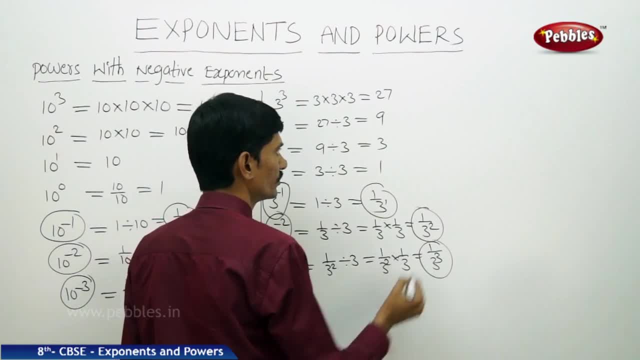 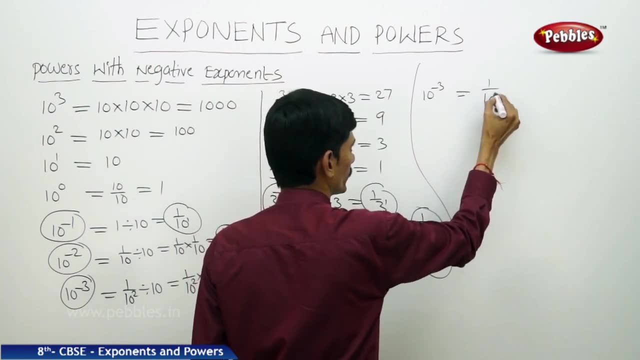 of minus 3 equals to 1 by 3 to the power of 3.. So in general, see here, 10 power minus 3 equals to 1 by 10 power 3 and 3 power minus 2, we got 1 by 3 to the power of 2.. So in 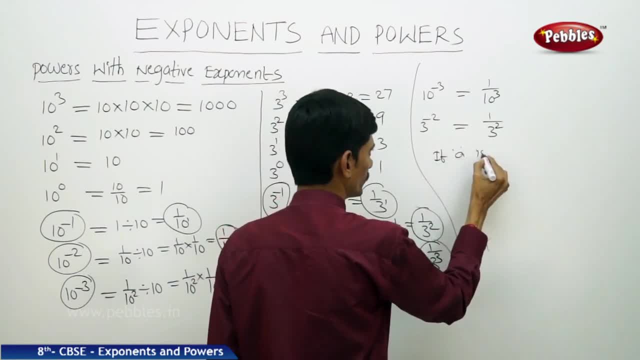 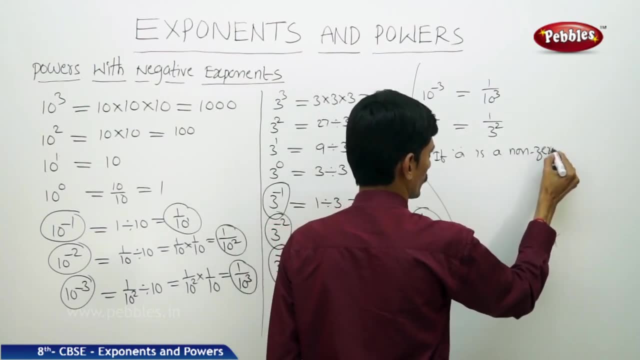 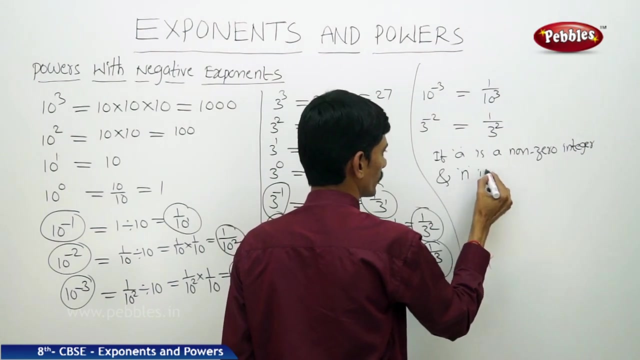 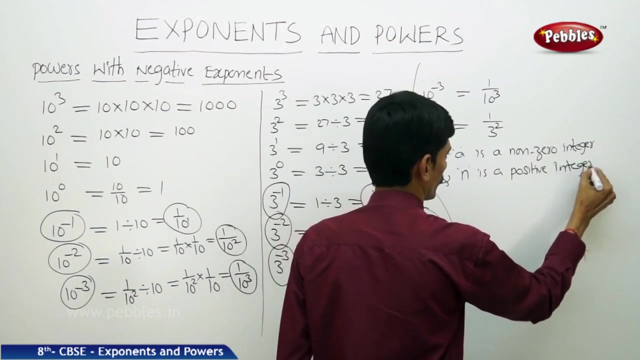 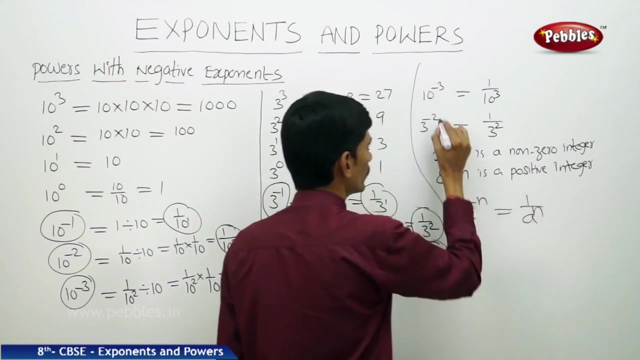 general, if a is a non zero integer and n is a positive integer, then we can write a to the power of minus n as 1 by a to the power of n. see 10 power minus 3 means 1 by 10 power 3, so here: 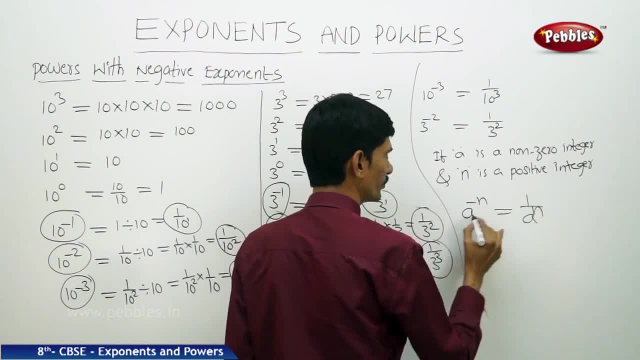 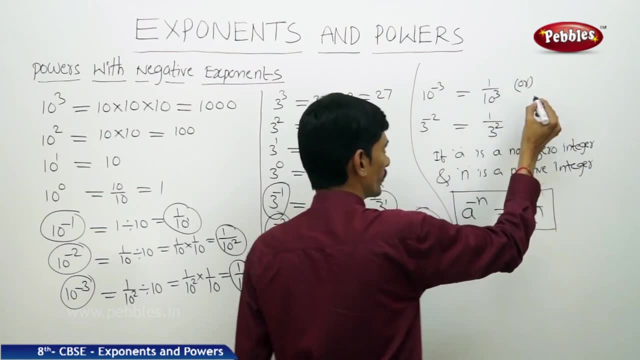 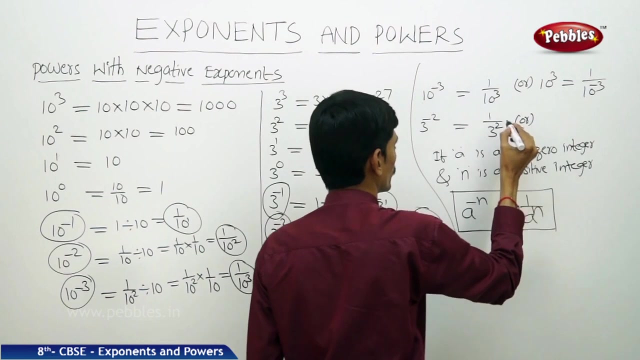 a to the power of minus n can be written as 1 by a to the power of n. or here, 10 power 3 can be written as 1 by 10 to the power of minus 3. here also, 3 power 2 can be written. 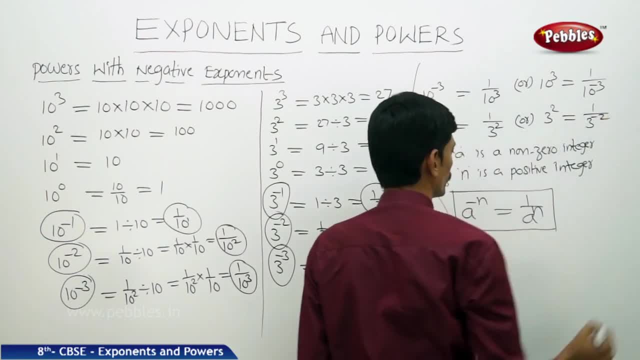 as 1 by 10 to the power of minus 3, so here also 3 power 2 can be written as 1 by 10 to 3 to the power of minus 2. so this formula can be written as a to the power of n equals to: 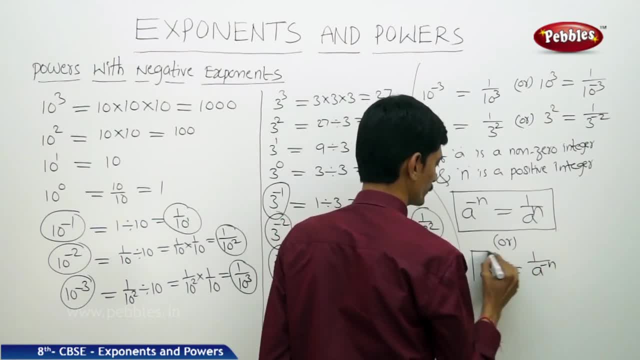 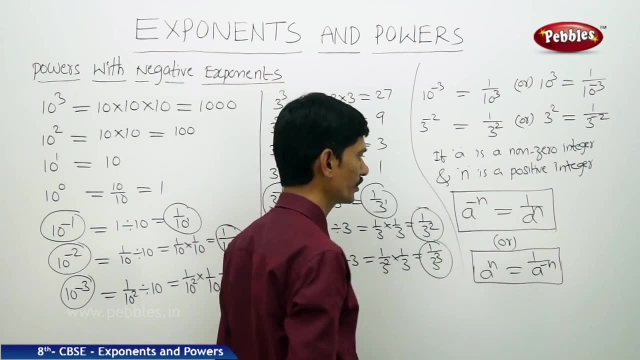 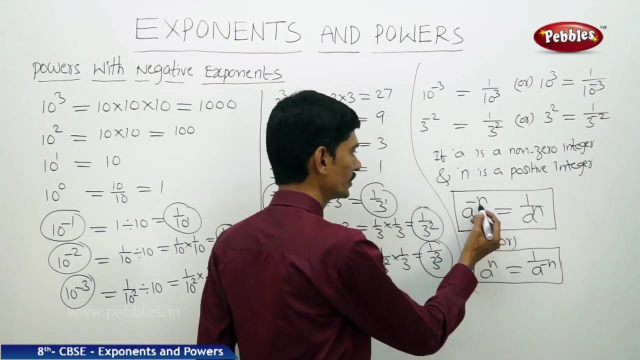 1 by a to the power of minus n. so if a is any non-zero integer and n is a positive integer, then we can write: a to the power of minus n equals to 1 by a to the power of n, or a to the power of n equals to 1 by a to the power of minus n. here a power minus n is the multiplicative. 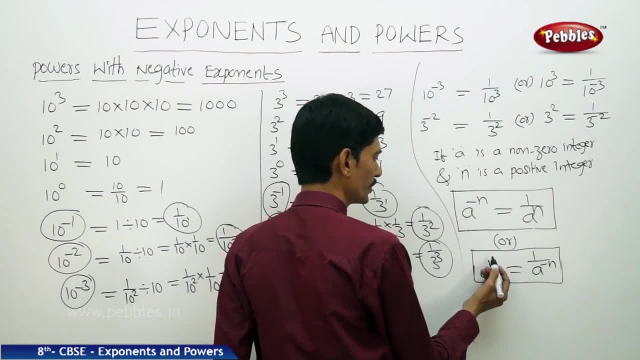 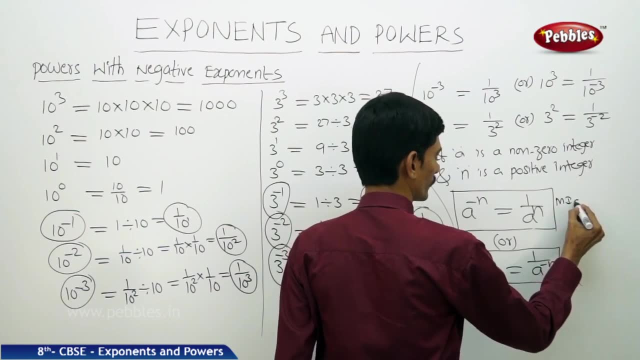 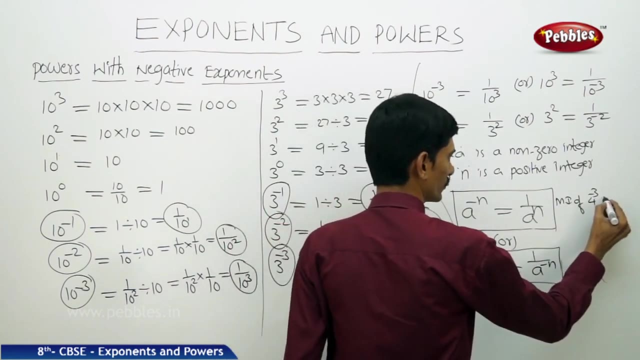 inverse of a power n, or here, a power n is the multiplicative inverse of a to the power of minus n. now, what is the multiplicative inverse of 4 power minus 3? so the multiplicative inverse of 4 power minus 3 is 4 to the power of 3. and what is the multiplicative? 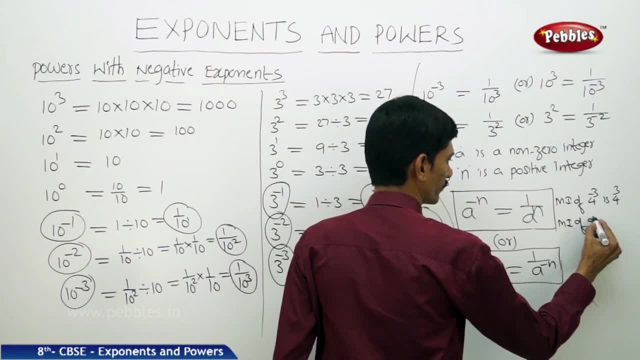 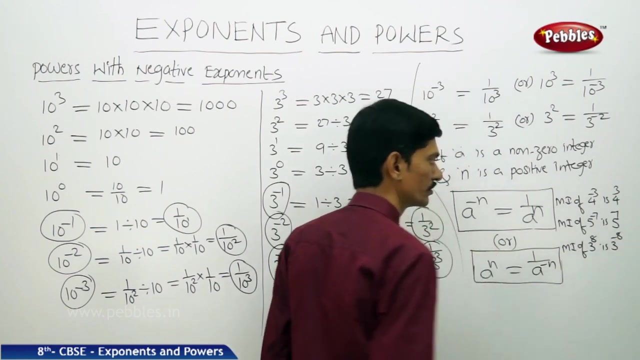 inverse of 5 power minus 7.. The multiplicative inverse of 5 power minus 7 is 5 to the power of 7.. And what is the multiplicative inverse of 3 power 8?? The multiplicative inverse of 3 power 8 is 3 to the power of minus 8.. Now let us see the question. now Write the. 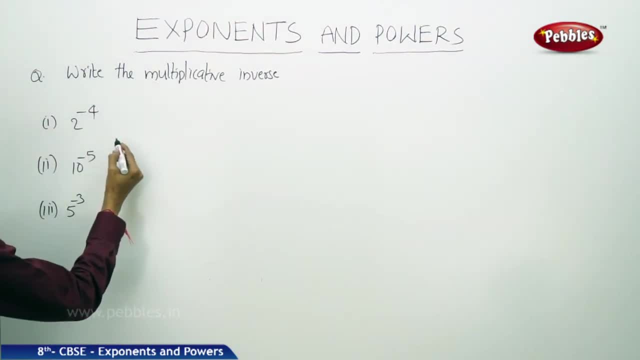 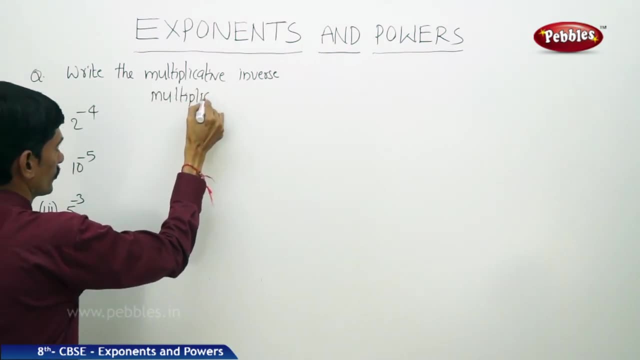 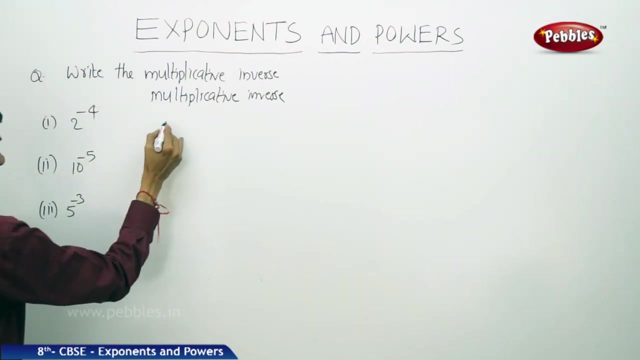 multiplicative inverse of the following: So what is the multiplicative inverse of 2 power minus 4?? So the multiplicative inverse of 2 to the power of minus 4 is 2 to the power of 4.. And the multiplicative inverse of 10 to the power of minus 5 is 10 to the power. 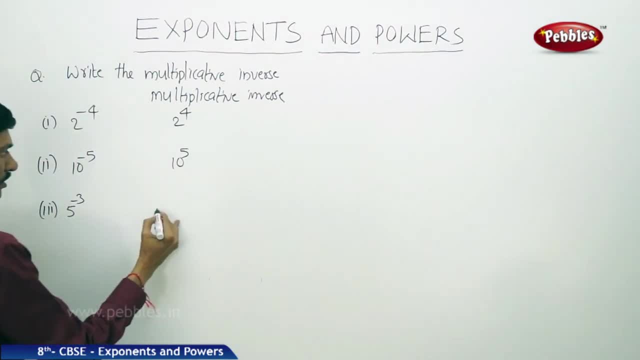 of 5.. And the multiplicative inverse of 5 to the power of minus 3 is 5 to the power of 3.. because the product of these two numbers is 1.. If the product of the two numbers is 1,, 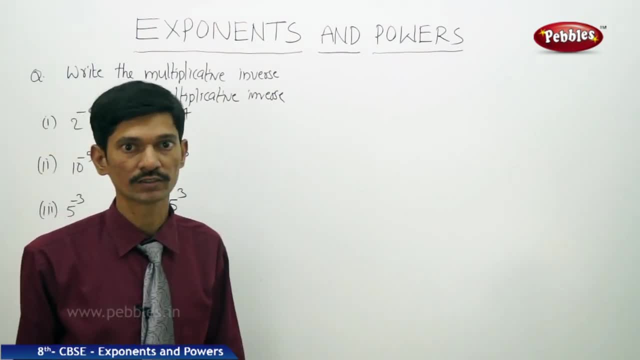 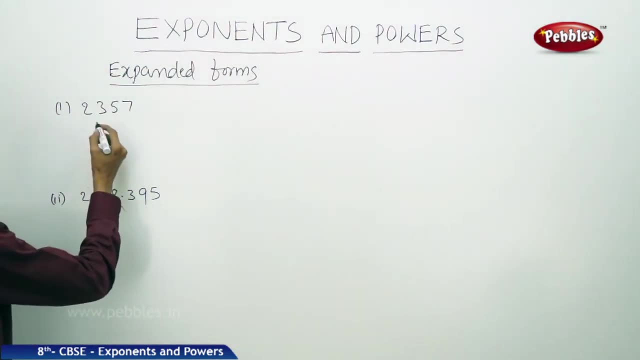 then each one is called the multiplicative inverse of the other. Now let us write the expanded forms of the following numbers using exponents. Now, the first question is 2357.. Now this can be written as now here: 2000 means its place value is 2000.. 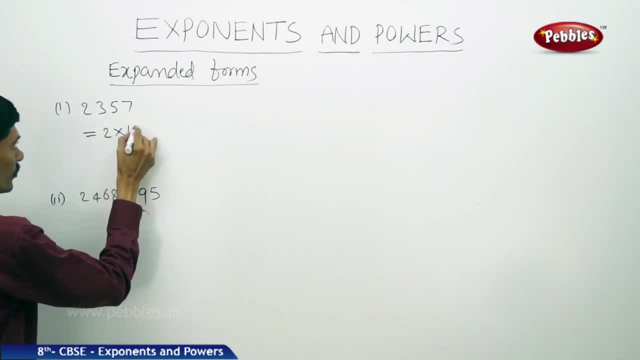 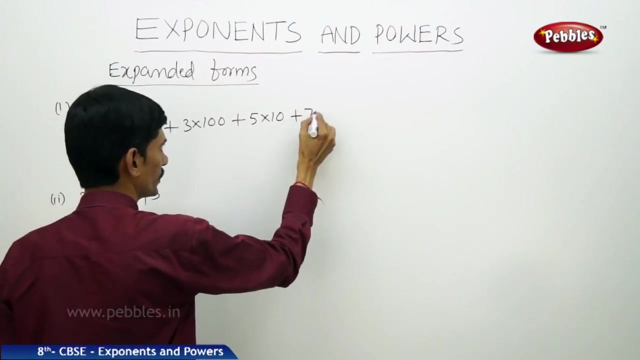 So we can write that 2 into 1000 plus 300.. So 3 into 100 plus 50.. So we can write 5 into 10 plus 7 in units plus, So we can write 7 into 1.. 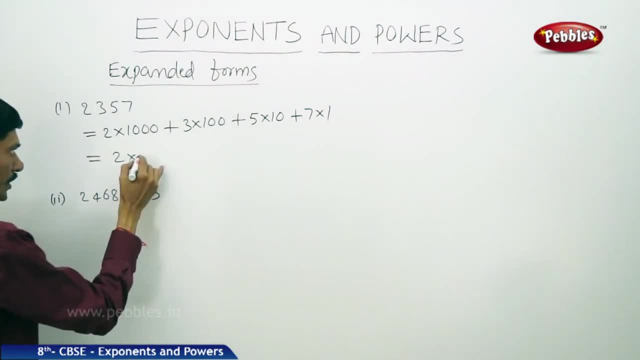 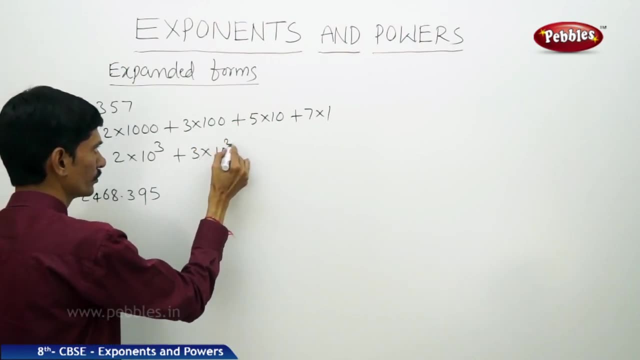 Now this equals to 2 into 1000. can be written as 10 to the power of 3. plus 3 into 100 can be written as 10 to the power of 2.. Plus 5 into 10 can be written as 10 to the power of 1.. 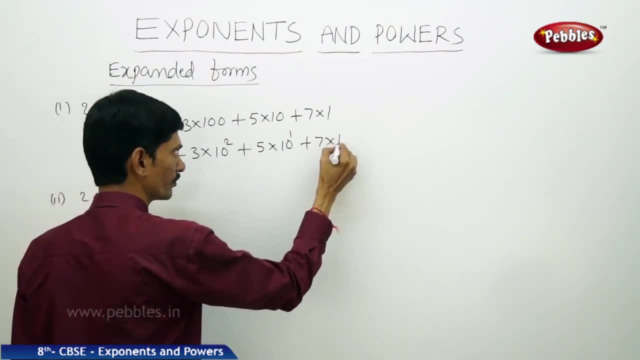 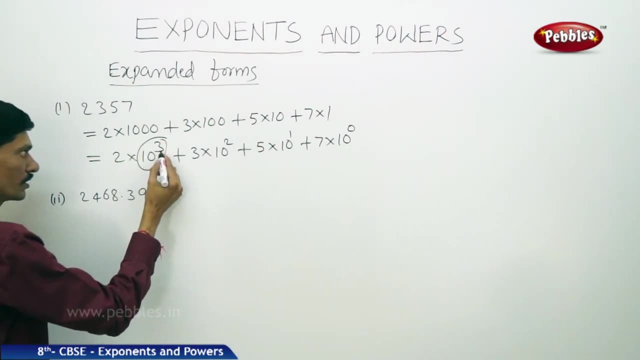 Plus 7 into 1 can be written as 10 to the power of 0.. So here we have taken the exponents and powers. here 10 raised to the power 3.. And here 10 square: 10 to the power of 1 and 10 to the power of 0.. 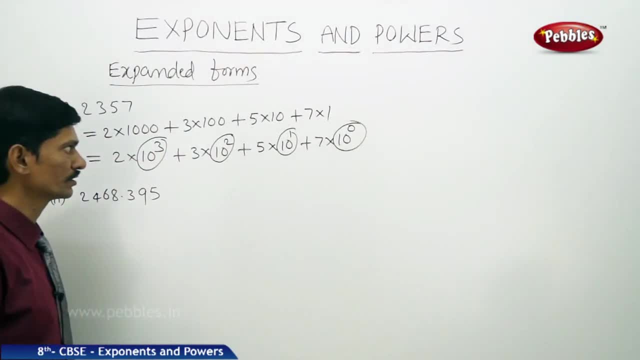 But we can write even the negative exponents while expanding a number. Now let us do that In second problem. So it is 2468.395.. Here 3 in 10th place means 1 by 10.. 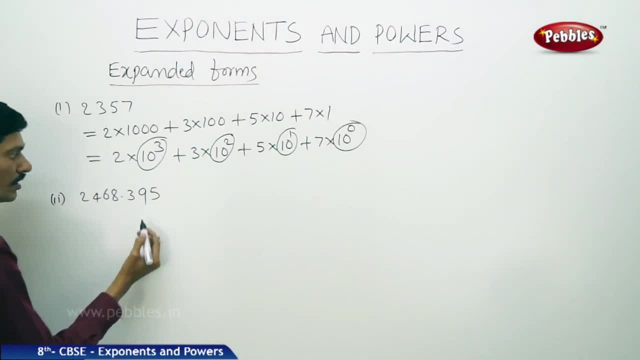 And 9 in 100th place means 1 by 100.. And 5 in 1000th place means 1 by 1000. So this can be expanded like this: 2000.. So 2 into 1000 plus 400.. 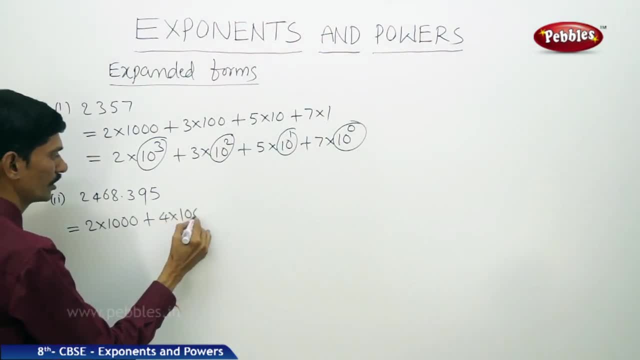 So we can write 4 into 100 plus 60.. 60 can be written as 6 into 10.. Plus 8. 8 in the units place, So we can write 8 into 1.. Plus 3 in the 10th place. 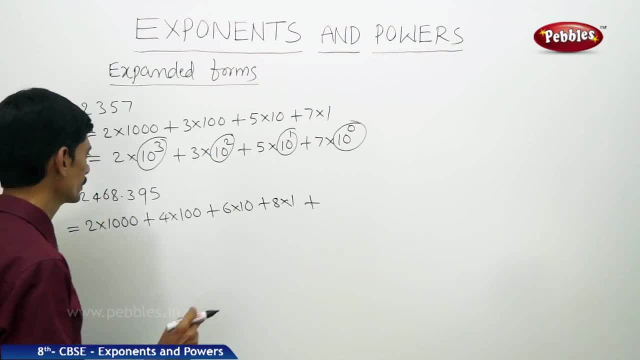 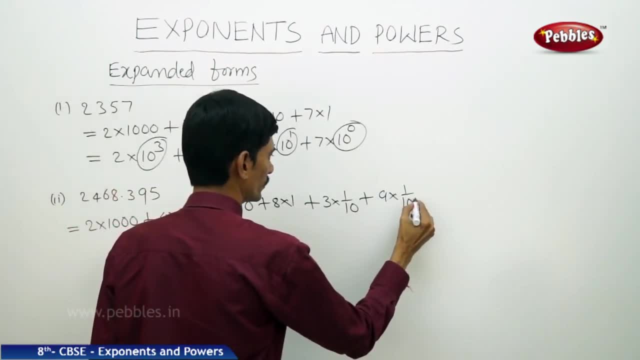 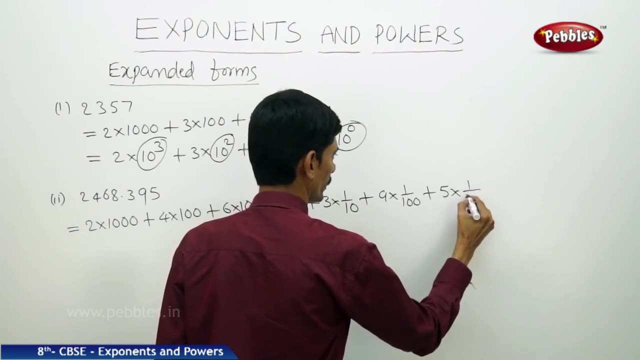 So we can write 9 in the 100th place. So we can write 9 in the 100th place. So we can write 9 in the 100th place. write 9 into 1 by 100 plus 5 in the 1000th place, So 5 into 1 by 1000.. Now this equals: 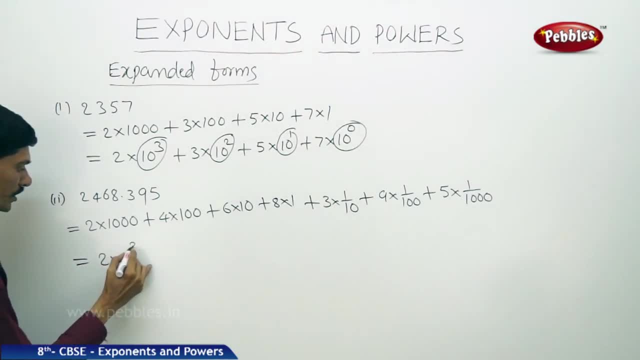 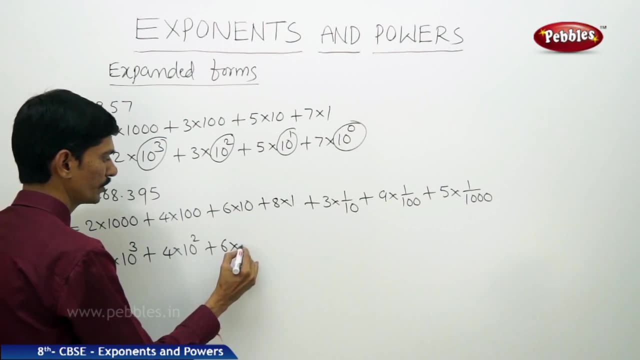 to 2 into 1000. can be written as 10 to the power of 3 plus 4 into 100. can be written as 10 to the power of 2 plus 6 into 10. can be written as 10 to the power of 1 plus 8. 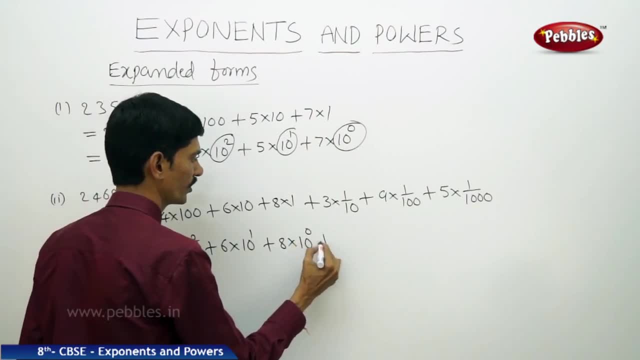 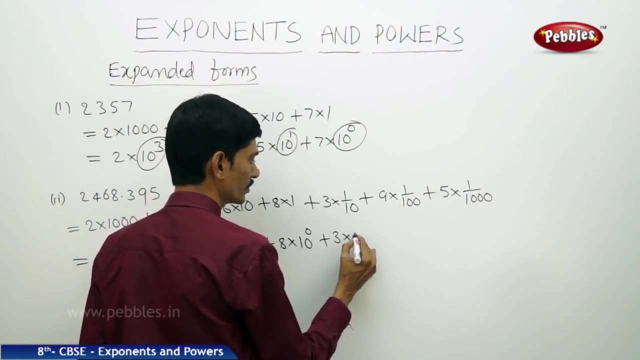 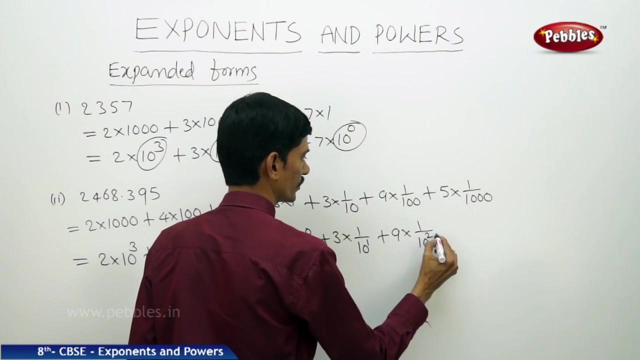 into 1 can be written as 10 to the power of 0 plus 3 into 1 by 10.. So this can be written as 1 by 10 to the power of 1 plus 9 into 1 by 10, to the power of 2 plus 5 into 1 by 10. 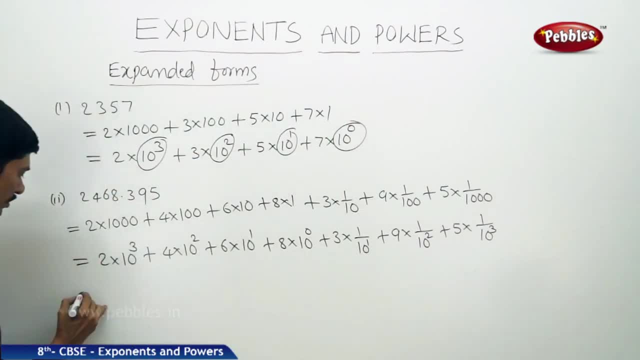 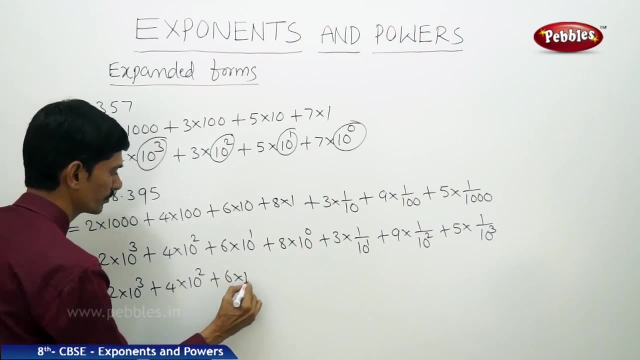 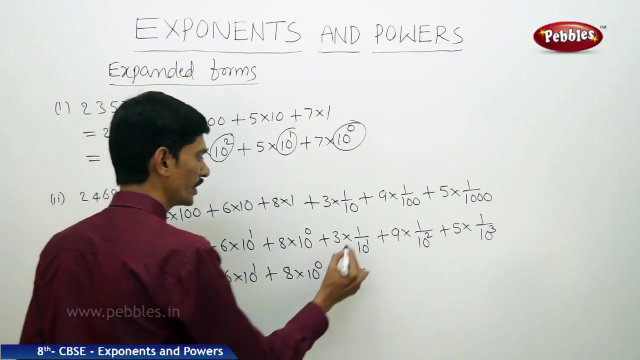 to the power of 3.. Now, this 2 into 10, to the power of 3 plus 4 into 10, to the power of 2 plus 6.. 6 into 10, to the power of 1 plus 8 into 10, to the power of 0 plus 3 into So, 1 by 10. 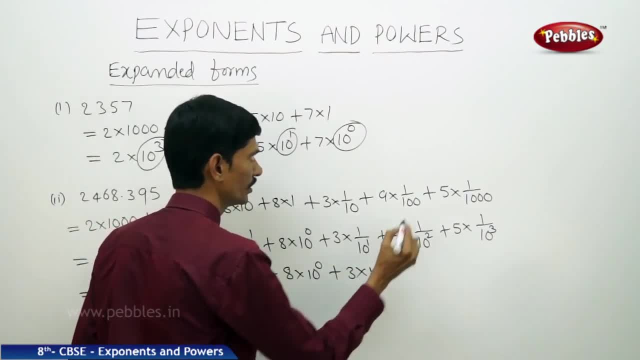 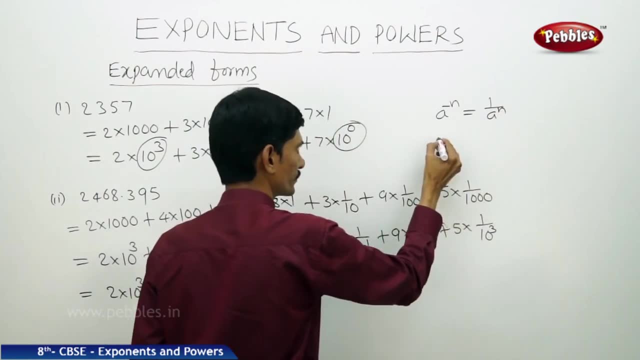 to the power of 1 can be written as: 10 to the power of minus 1, using 8 to the power of minus n equals to 1 by 8 to the power of n, or 8 to the power of n equals to 1 by 8. 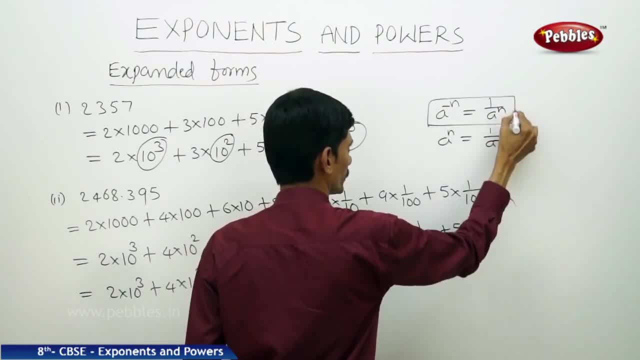 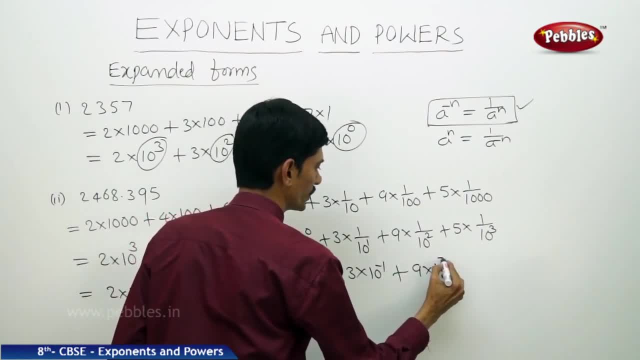 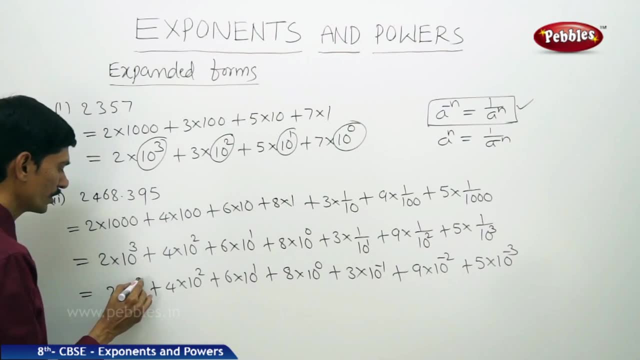 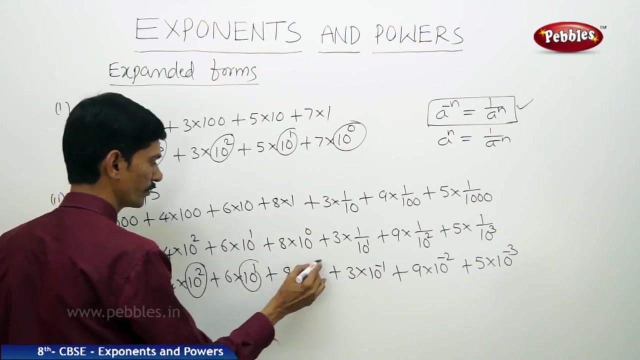 plus 9 into 10 to the power of minus 2, plus 5 into 10 to the power of minus 3.. So here we are using even the positive exponents and also the negative exponents. So 10 power 3, 10 power 2, 10 power 0. So these three are positive exponents. This is to the power. 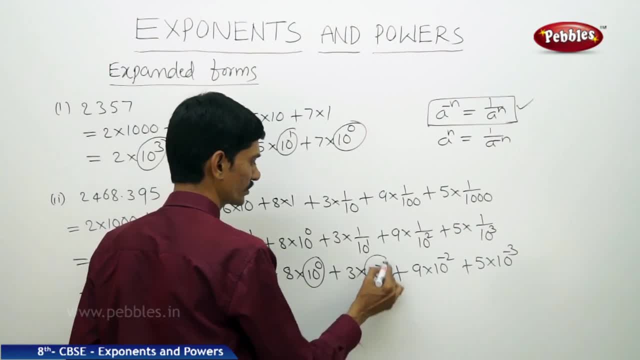 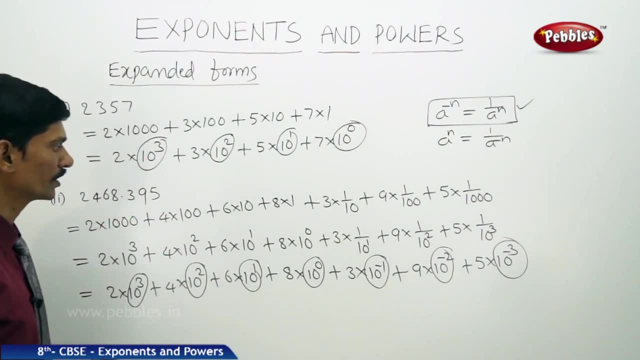 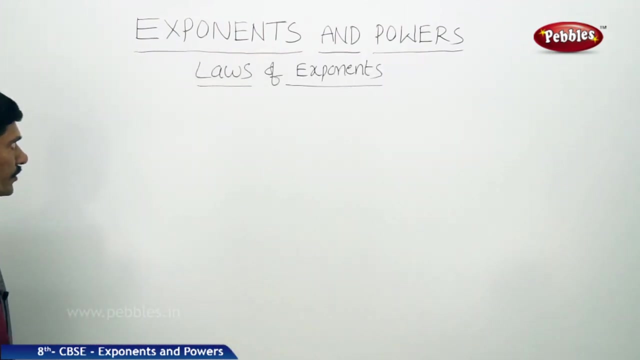 0 and the negative exponents are 10 to the power of minus 1,, 10 to the power of minus 2, 10 power minus 3.. So while expanding a number or a decimal number, we use even the negative powers. Now the next topic: laws of exponents. So in 7th standard we 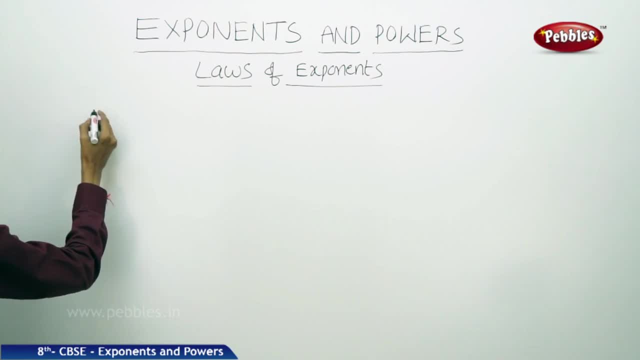 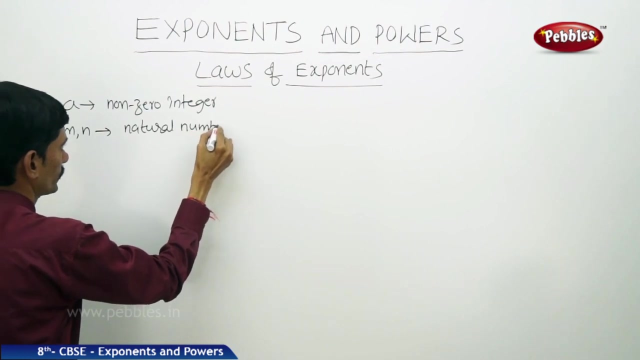 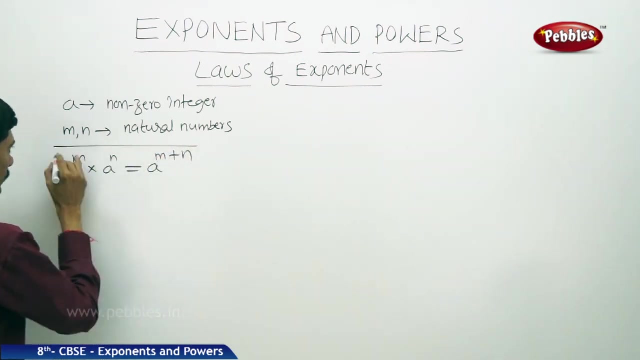 have already learnt one law of exponents: that if a is a non-zero integer and m, n are natural numbers, It means only positive integers- Then a to the power of m into a to the power of n equals to a to the power of m plus n. So this formula is: 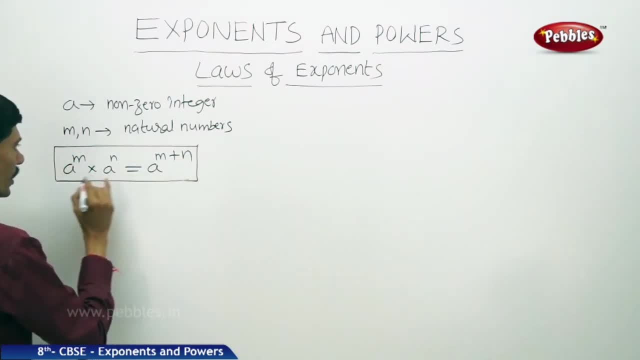 only if a is any non-zero integer and m, n are natural numbers. means that we can take a value is any integer like minus 5 or plus 5, but the exponents must be taken only the positive numbers. means natural numbers, means only positive numbers. so m value. 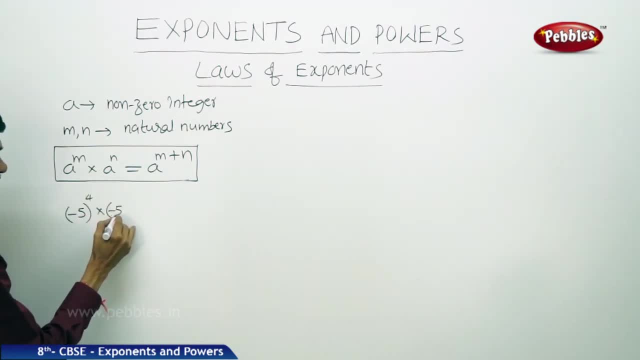 if it is 4 into minus 5 to the power of 3, equals to minus 5 to the power of 4 plus 3, this equals to minus 5 to the power of 4 plus 3 is 7. so here the exponents are only the. 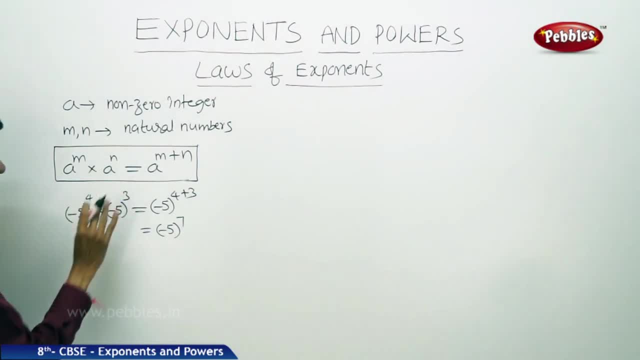 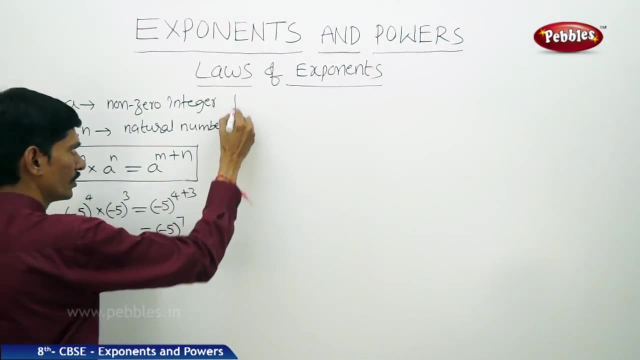 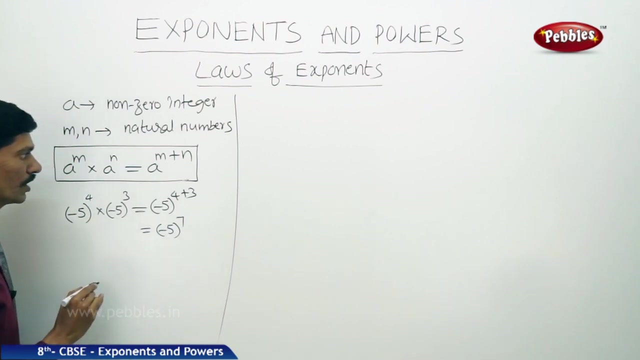 positive numbers if you take the negative exponents. so even though, does the law hold the same? again? now let us see with an example. so in place of m and m, if you take the negative numbers, means any integers, either positive or negative integers, then the formula will: 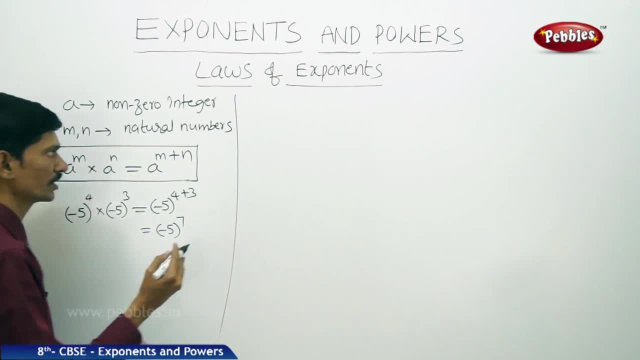 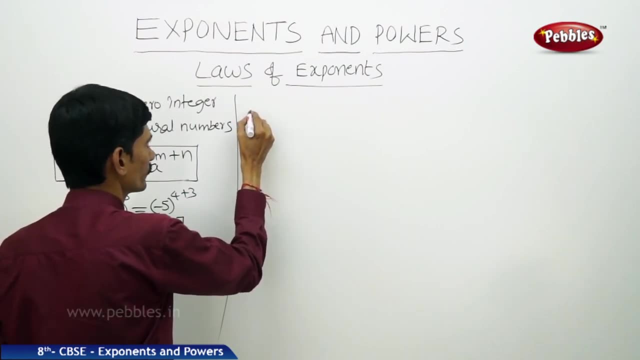 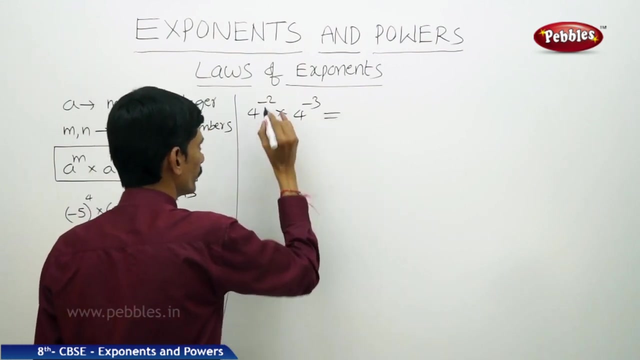 be the same means the law will be the same or not. let us check with an example. now take a values. any integer like 4 and the powers means exponents. i am taking the negative exponents. so 4 power minus 2 into 4, to the power of minus 3. now this equals to 4 power minus 2 can be written as 1 by. 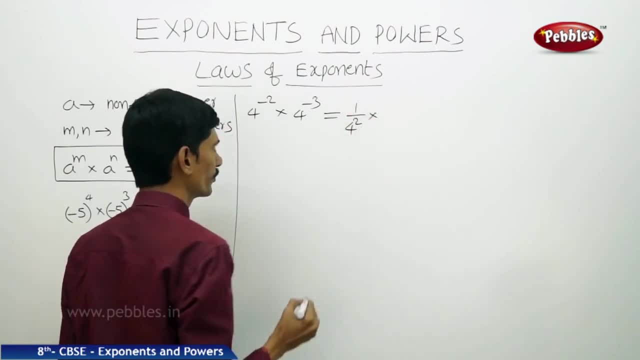 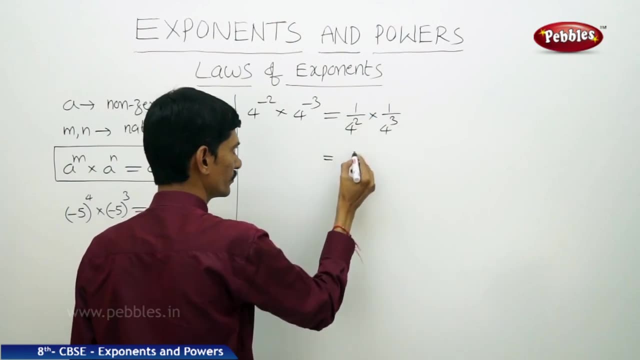 4 to the power of 2 into 4. power minus 2 minus 3 can be written as 1 by 4 to the power of 3.. Now this equals to 1 into 1, 1 by. So here, according to this law, 4 power 2 into 4 power 3 can be written as 4 power 2 plus. 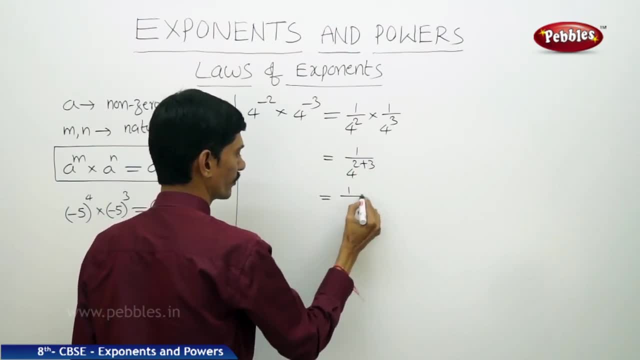 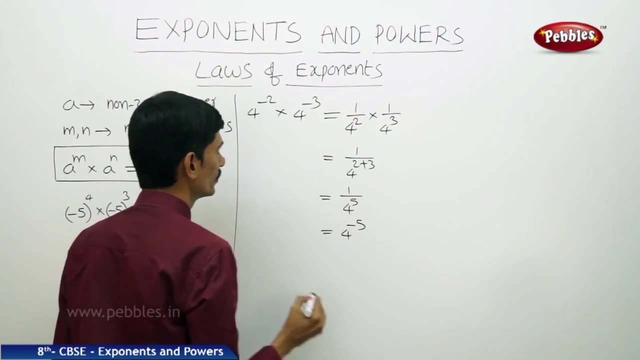 3. This equals to 1 by 4 to the power of 5.. Now this can be written as 4 to the power of minus 5.. So here we observe that 4 power minus 2 into 4 to the power of minus 3 equals. 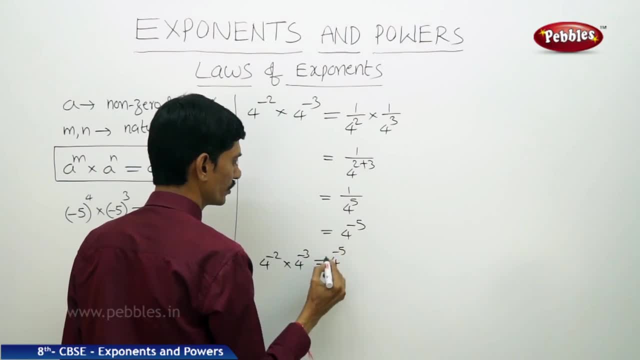 to 4 to the power of minus 5.. Now this is same as so 4 to the power of minus 2 plus of minus 3.. So here, a to the power of m into a to the power of n equals to a to the power. 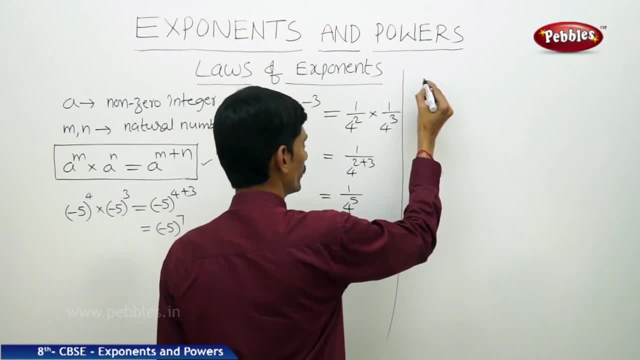 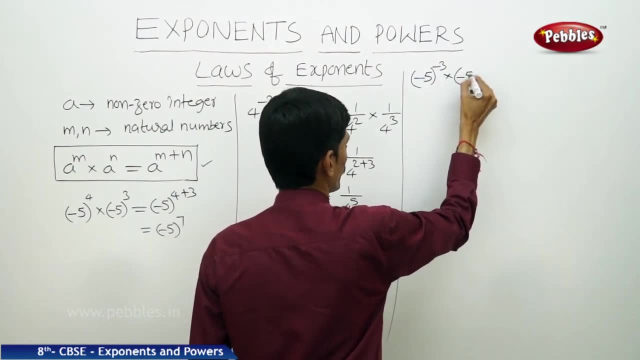 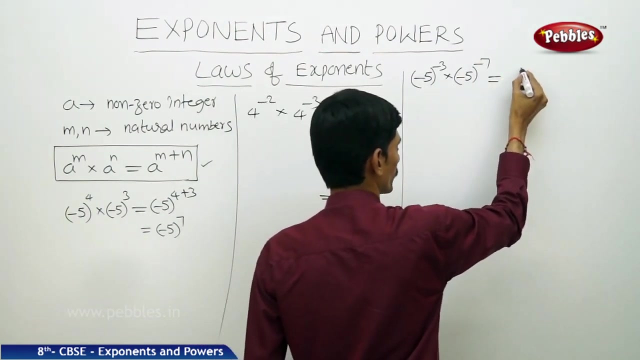 of m plus n. Now let us take another example: minus 5, minus 5.. 1 to the power of minus 3 into minus 5, 1 to the power of minus 7.. Now this equals to minus 5, 1 to the power of minus 3. can be written as 1 by minus 5, 1 to the power. 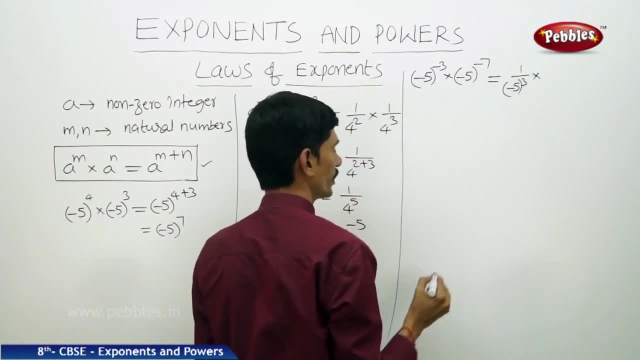 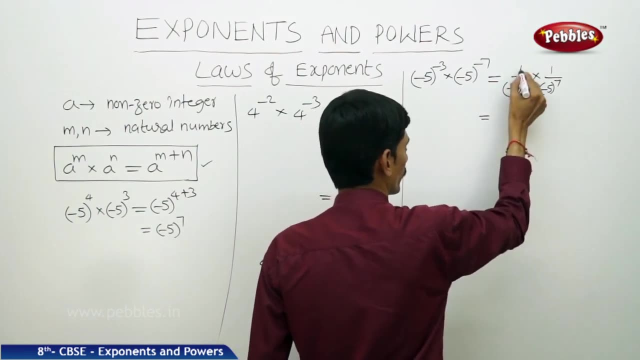 of 3 into minus 5, 1 to the power of minus 7 can be written as 1 by minus 5, 1 to the power of 7.. Now this equals to 1, 1's are 1 by minus 5, 1 to the power of 3 into minus. 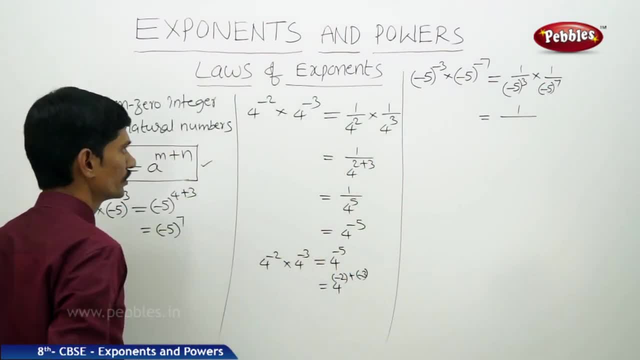 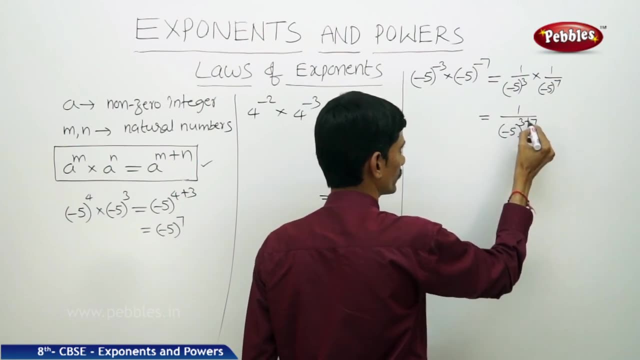 5, 1 to the power of 7.. So now, according to this law, here 3 and 7 are natural numbers, So we can write minus 5 over the power of 3 plus 7.. This equals to 1 by minus 5 over the power of 3 plus 7 is 10.. 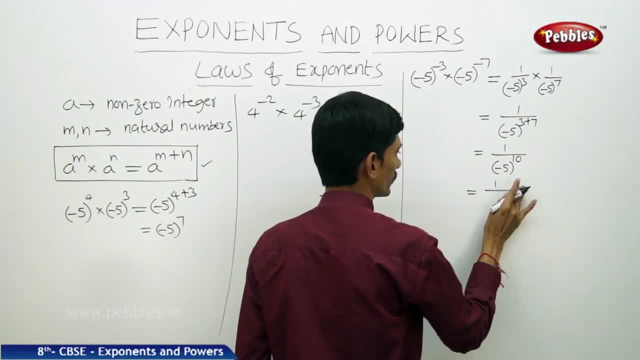 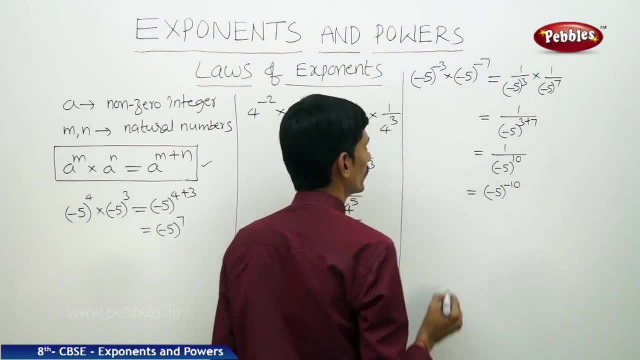 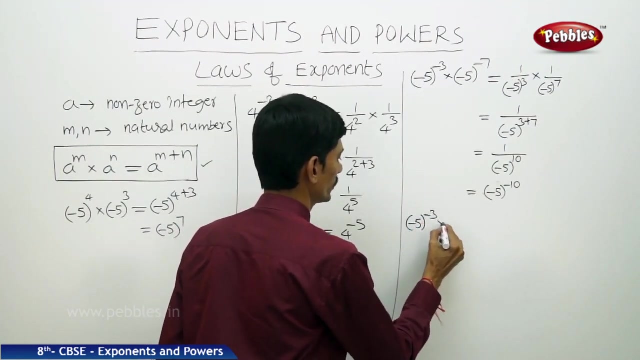 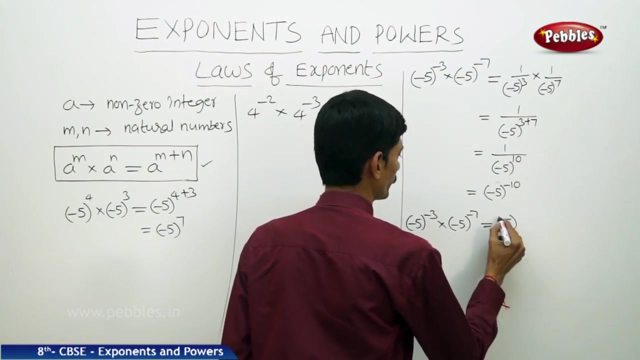 Now this can be written as 1 by minus 5 over the power of minus 10.. Now we observe that minus 5 over the power of minus 3 into minus 5 over the power of minus 7 equals to minus 5 over the power of minus 10.. 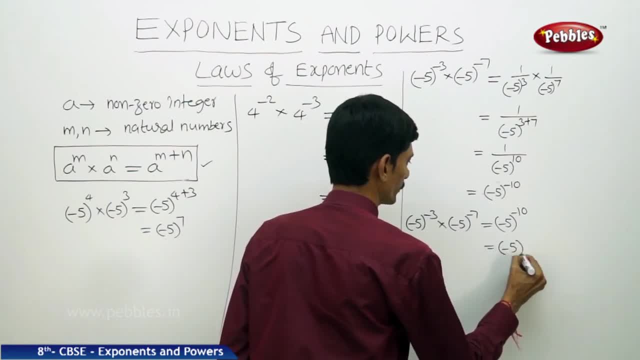 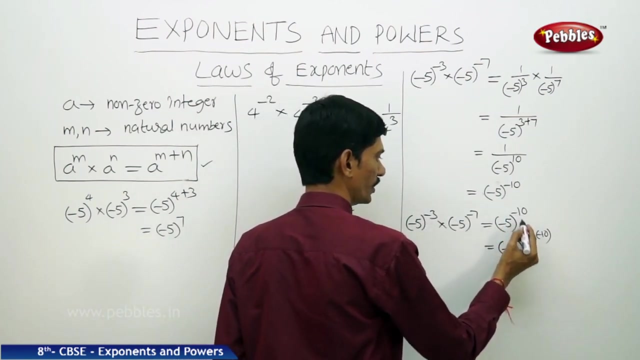 So, which is equals to minus 5, over the power of These exponents are added So minus 3 plus half, minus 10.. So, even though the exponents are negative, the exponent of the result is same as the sum of the two negative exponents. 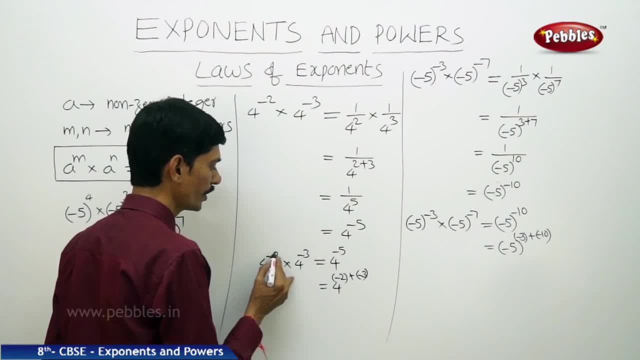 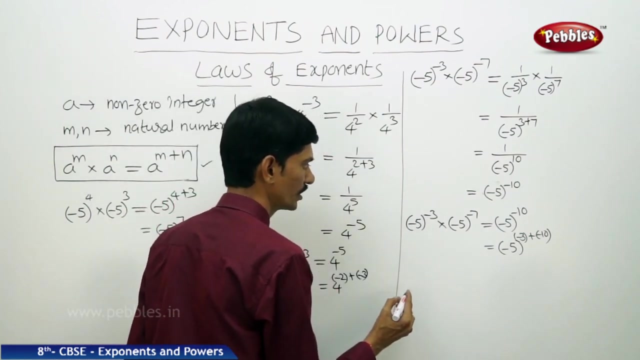 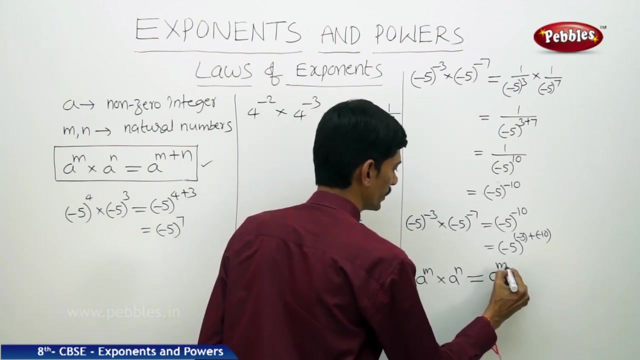 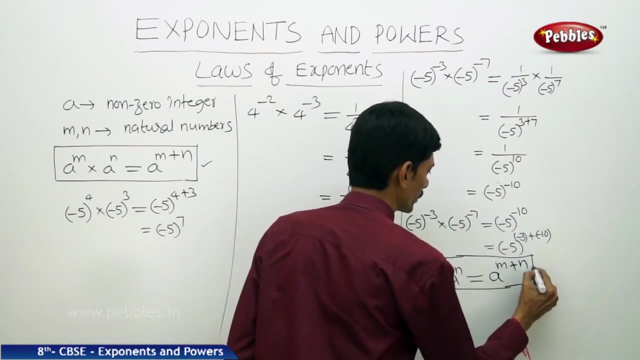 So even in this example also, when 4 power minus 2 into 4 power minus 3, this equals to. We observe that 4 power minus 5 means the negative exponents are added. So these two examples, The negative exponents, are added. So then we can write in general that a to the power of m into a to the power of n equals to a to the power of m plus n. where a is any integer, means non-zero integer and m comma n are any integers. 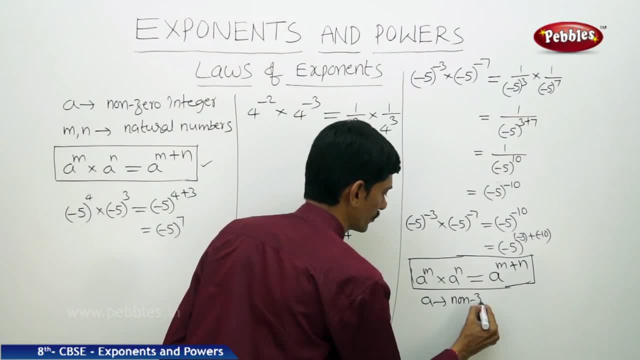 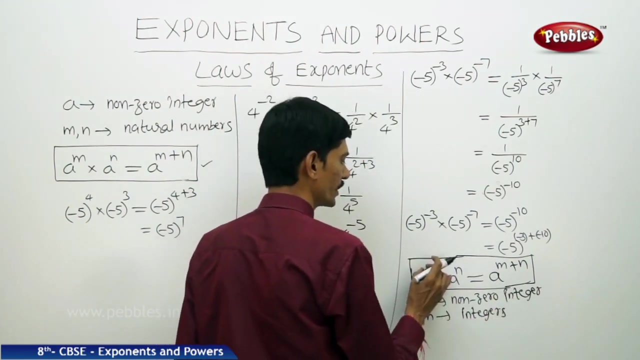 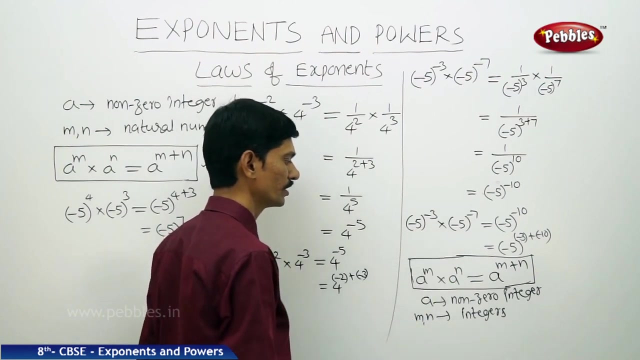 So here a is non-zero integer And m comma n are integers. means here we can take the exponents. even the negative means not only m and n are positive. if you take the negative exponents the law holds the same. 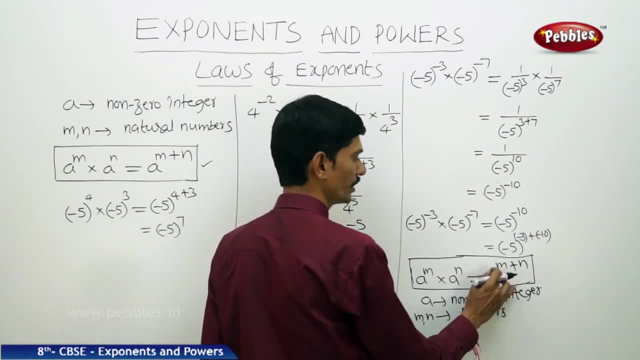 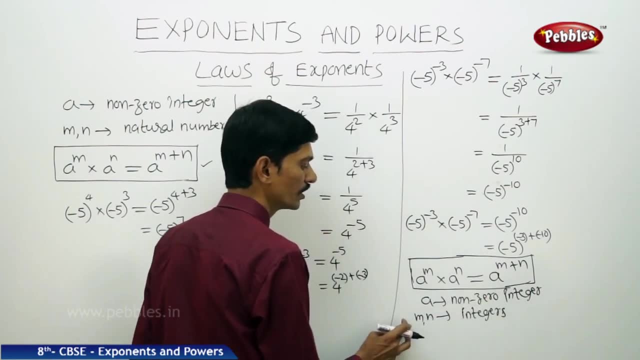 So a power m into a power n equals to a to the power of m plus n. So this is true for a value, any non-zero integer, And for m comma n, any integers. So now we can indeed, with a to the power of n plus n plus a to the power of description, we can do that. 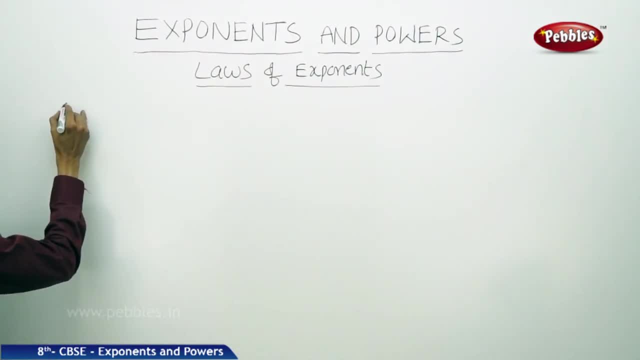 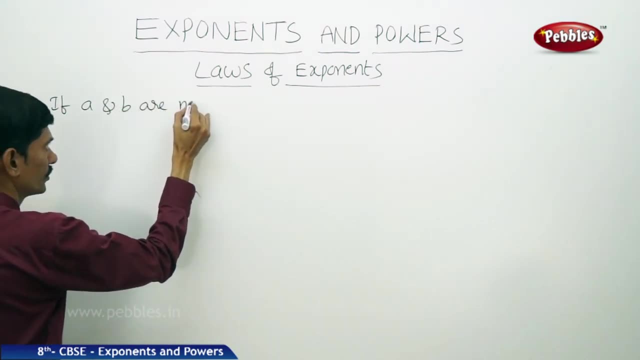 we can list out all the laws of exponents. so if a and b are non-zero integers, m and n are integers. k to the power of n is dash over n squared right. k to the power of n plus n minus a to the power of m plus n squared. 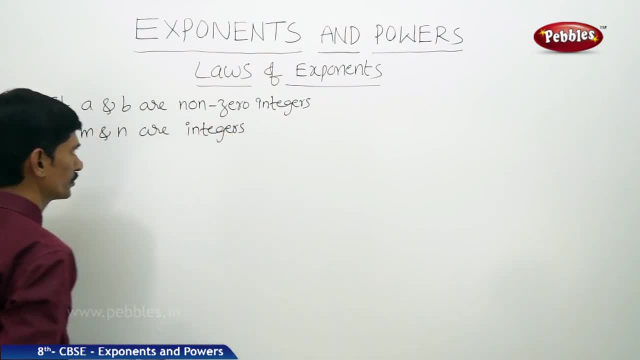 k times, flow times, zero gain. we can calculate that t to the power of free weight, then that z to the power of 10. things is zero. take over, gave k and b are non-zero. integers may be positive or negative integers. then we can write the loss of exponents. The first: 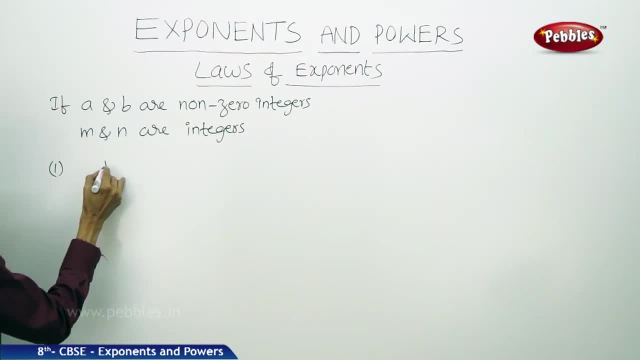 one we have proved just now. so that is a to the power of m into a to the power of n equals to a to the power of m plus n. Now the second one is a to the power of m divided by a to the power of n equals to a to the power of m minus n. The third one is a to 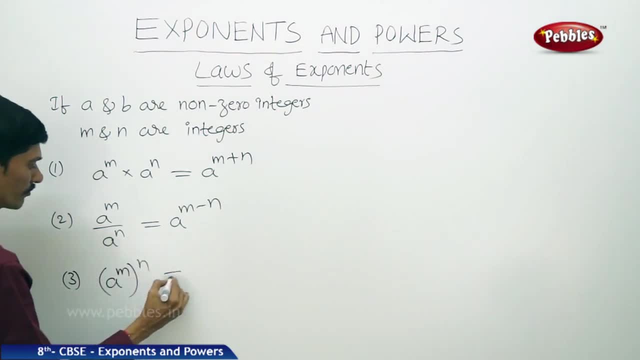 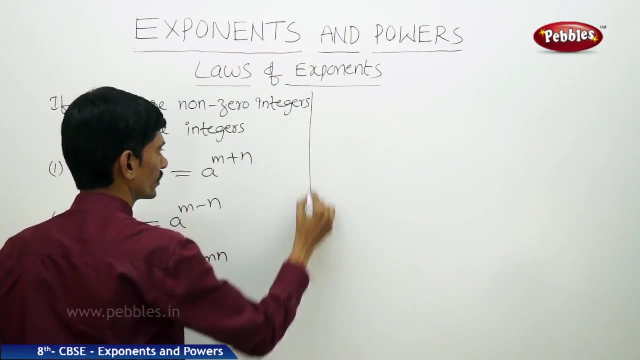 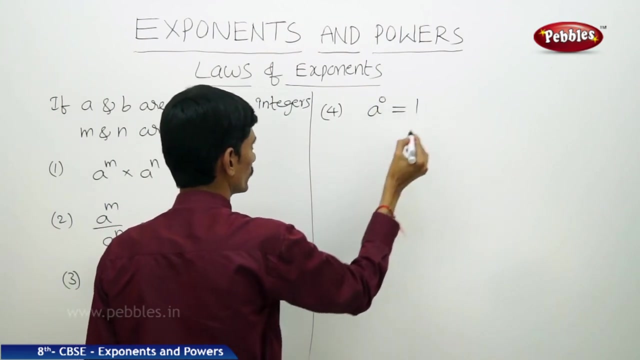 the power of m whole to the power of n equals to a. to the power of m into n. Next fourth one: a to the power of 0 equals to 1.. Next fifth one: a to the power of 0 equals to 1.. 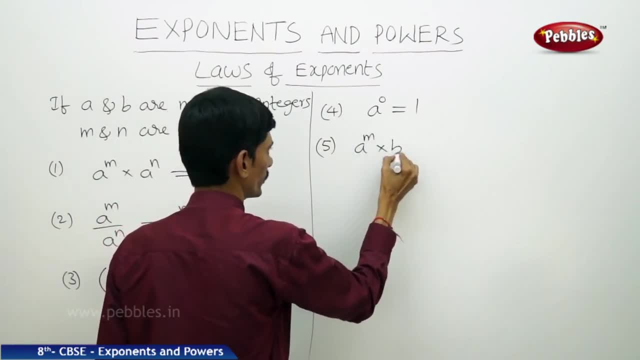 Next fifth one: a to the power of 0 equals to 1.. Next fifth one: a to the power of 0. a to the power of m into b to the power of m equals to a into b whole to the power of. 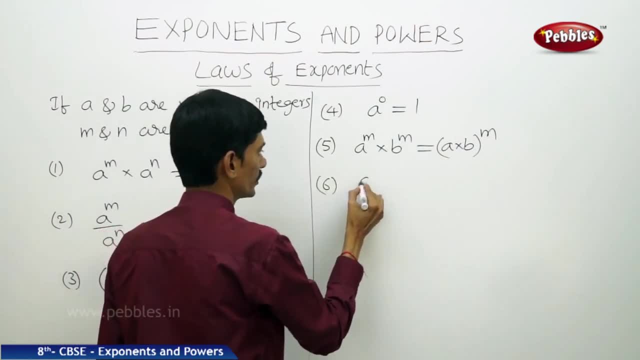 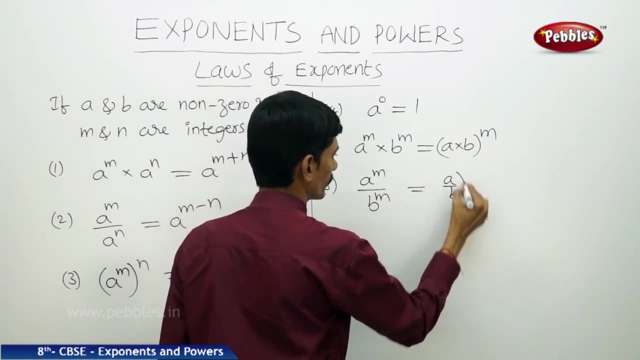 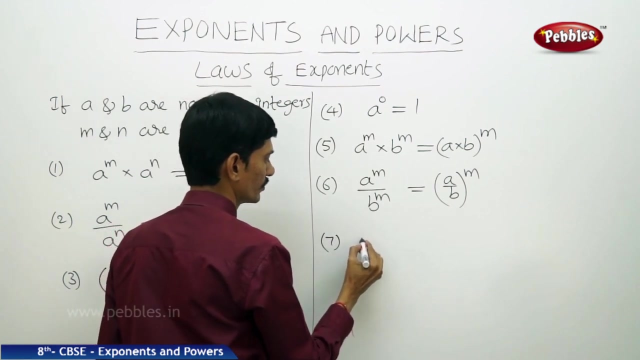 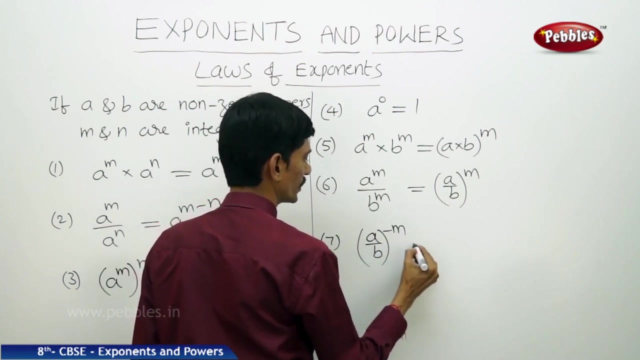 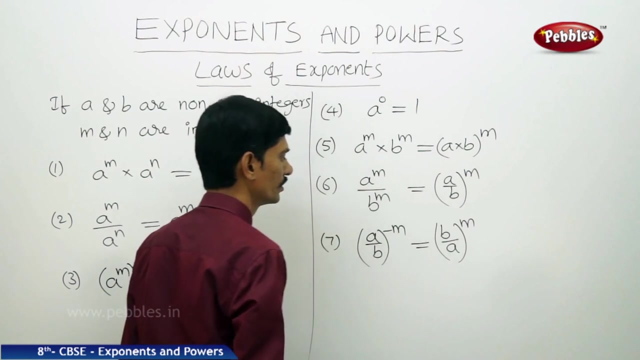 m. sixth one: a to the power of m divided by b to the power of m. this equals to a by b whole to the power of m. now the seventh one: a by b whole to the power of negative exponent. like minus m equals to. this can be written as b by a whole to the power of plus m. so 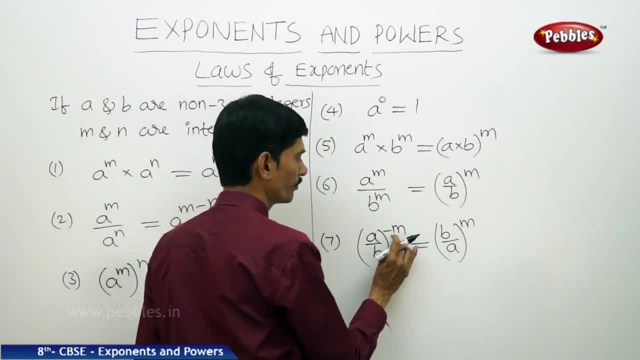 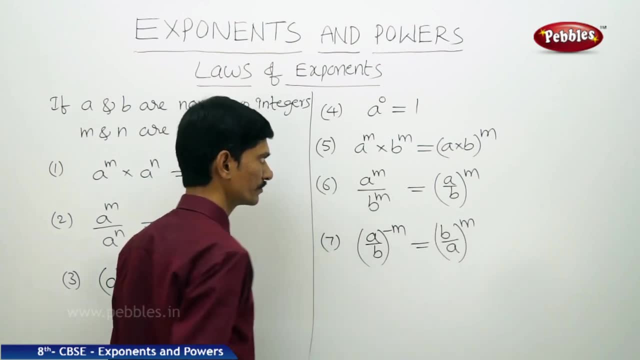 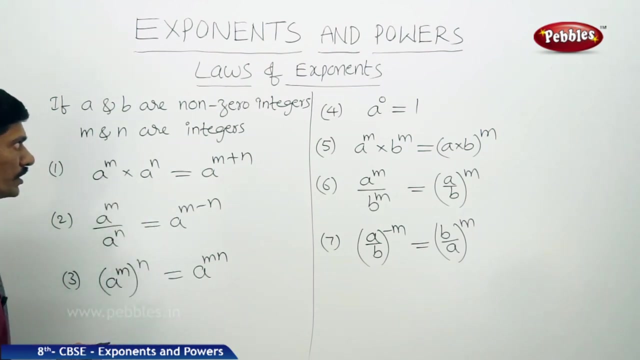 when you change the power exponent minus m as the positive exponent, then we should write the reciprocal of b to the power of m into b, to the power of m into b to the power of a by b means b by a. so these all laws are true for a and b, any nonzero integers and 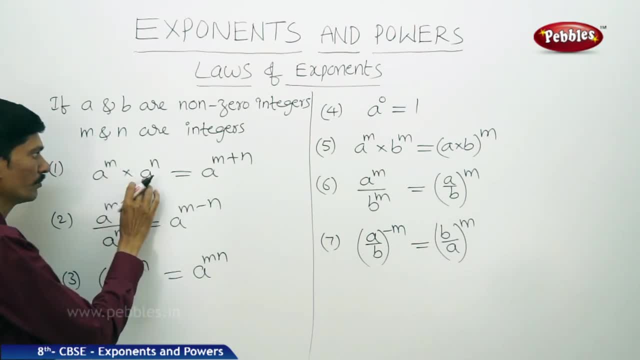 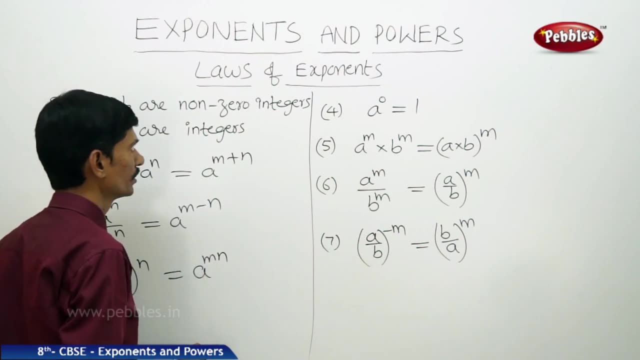 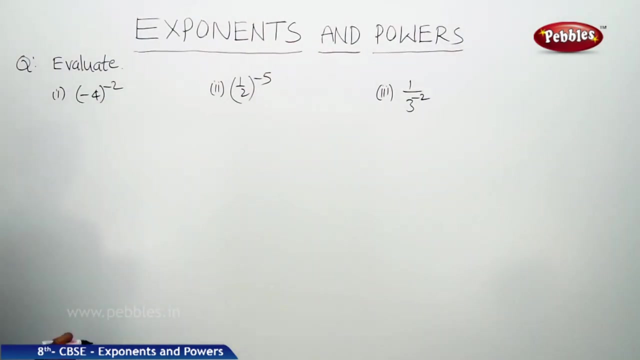 m and n are any integers. so here a value must be a and b values must be nonzero integers and the exponents m and n may be any integers. now let us solve few problems. the first question: evaluate minus four whole power minus two. now we can. this is according to the law, minus a to the 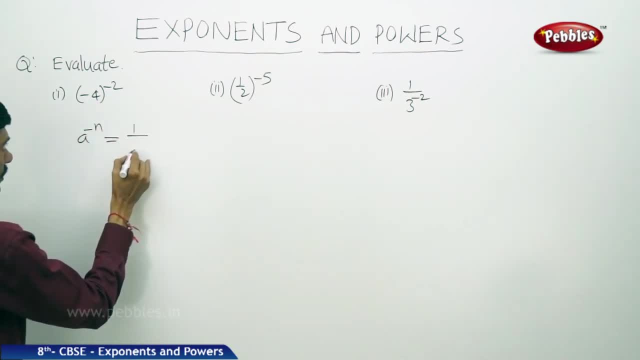 power of minus n equals to one by a to the power of n. so, according to this law, minus four whole to the power of minus two equals to one by minus four whole to the power of plus two. when this comes to the denominator, the negative power will become negative power. minus n, minus n, minus e. All right, then x would nuestra denommeinator of negativevector, of negative tails, would be negative tails forever, and then any other exponent would be negative. he would have minus n from all the deff e squared when e payments to the denominator negative six. this is some random y a and e to the number of organize n, so let us Aub serite y. would not al tab agree to this during the damitur is balanced by their argument besides the others, and y is equal to the complexity. 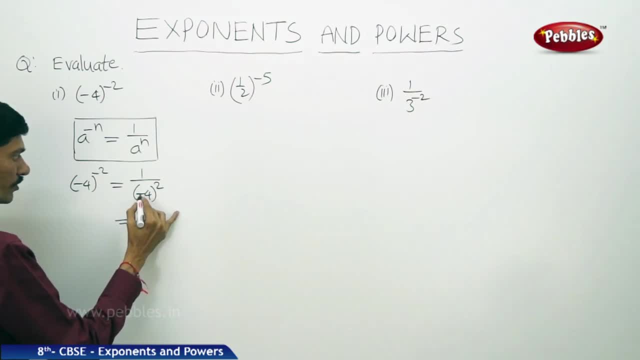 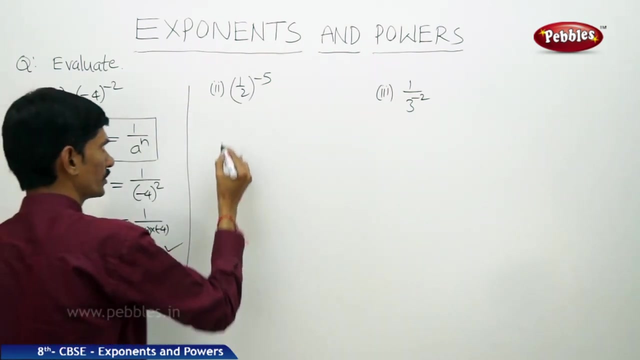 the positive power. So this 1 by minus 4 whole square means minus 4 into minus 4.. Now this equals to 1 by minus into minus plus 4. 4's are 16. So this is 1 by 16.. Now 1 by 2 over. 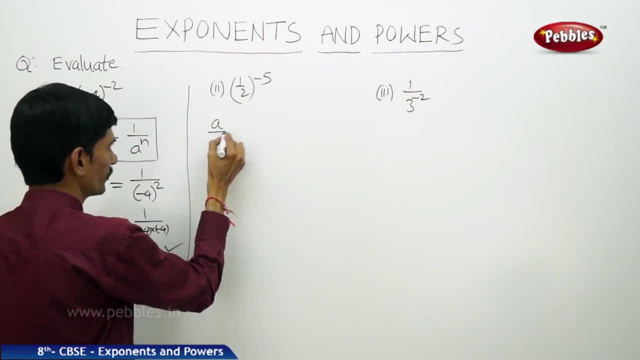 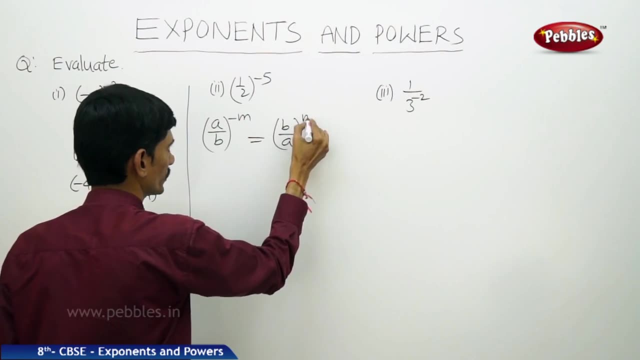 to the power of minus 5.. So this is: according to the law: a by b over to the power of minus m equals to b by a over to the power of m. Now I can write 1 by 2 over to the power of. 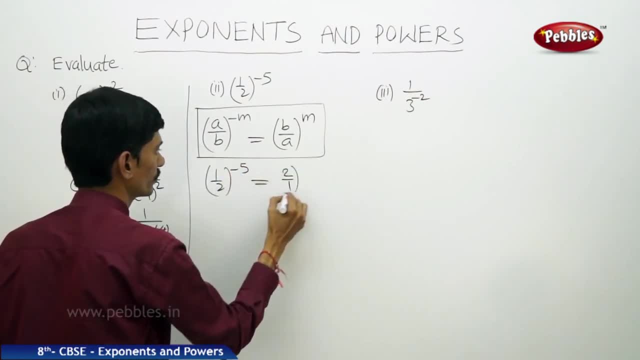 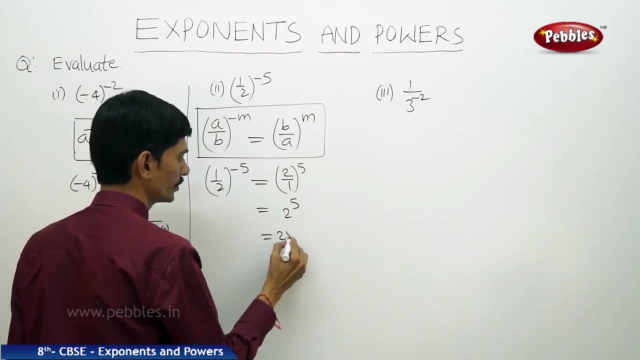 minus 5 equals to 2 by 1 over to the power of 5.. So 2 by 1 means 2 to the power of 5.. So 2 power 5 means 2 into 2, into 2, into 2.. 2 is multiplied 5 times 2, 2's are 4, 4- 2's. 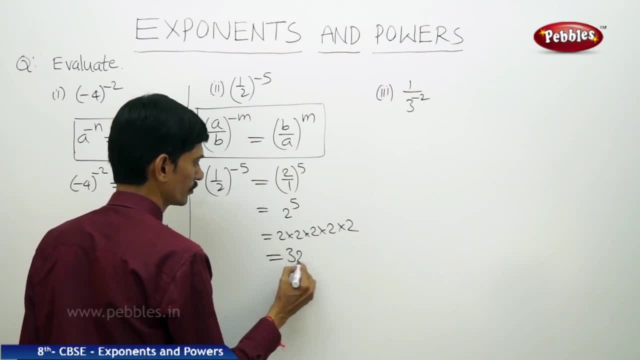 are 8,, 8 2's are 16, 16 2's are 3.. So this is 1 by 2 over to the power of minus 5.. So this is 1 by 2 over to the power of 32.. Now the next question: 1 by 3 power minus 2.. So 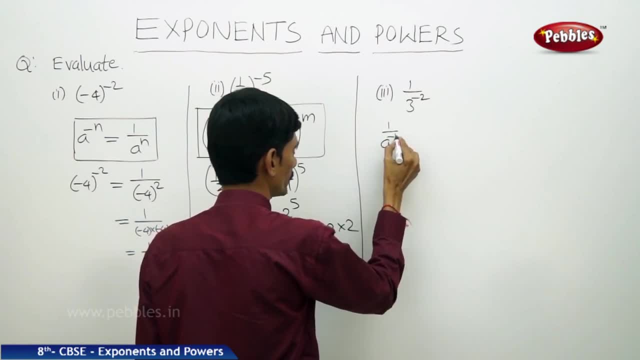 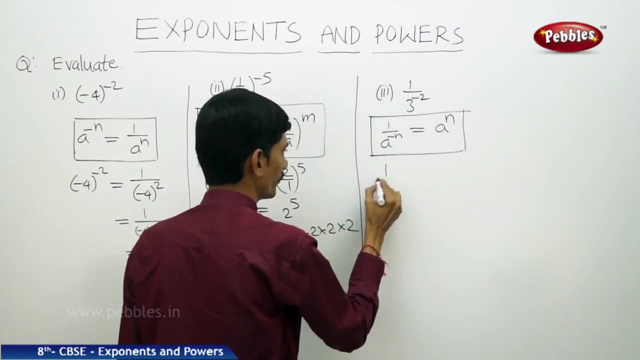 this is according to the formula: 1 by a to the power of minus n equals to a to the power of n. Now, 1 by 3 to the power of minus 2 equals to 3 to the power of plus 2.. So this equals: 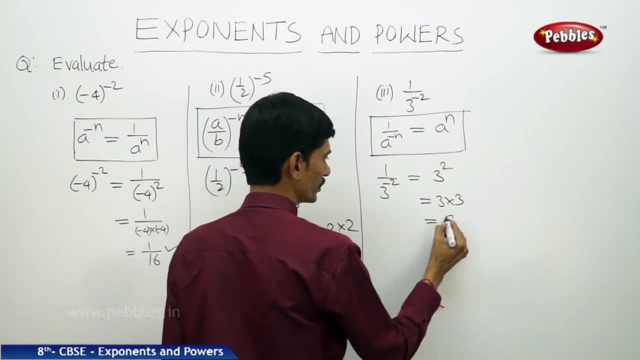 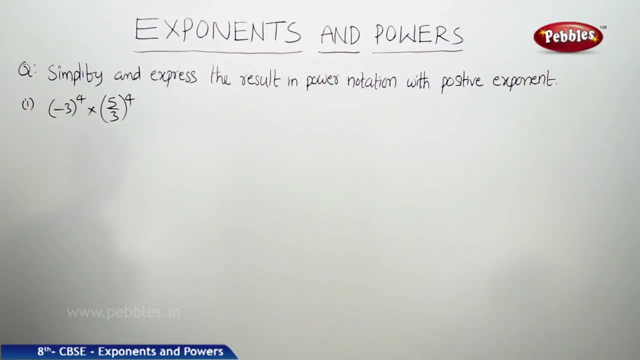 to 3 into 3.. 3 is multiplied 2 times 3, these are 9.. Now let us solve the next question. Simplify and express the result in power notation with positive exponent. Now the first question is: minus 3 over to the power of 4 into 5, by 3 over to the power of 4.. So we should express: 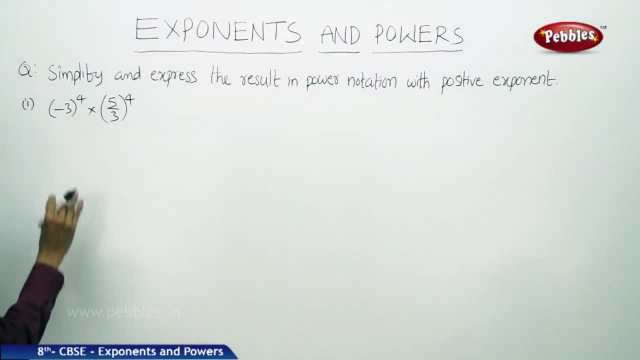 the result in the power notation with positive exponent. So the negative exponent should be changed as positive exponent. So this equals to: minus 3 over to the power of 4 is same minus 3.. So minus 3 over to the power of 4 can be written as minus. 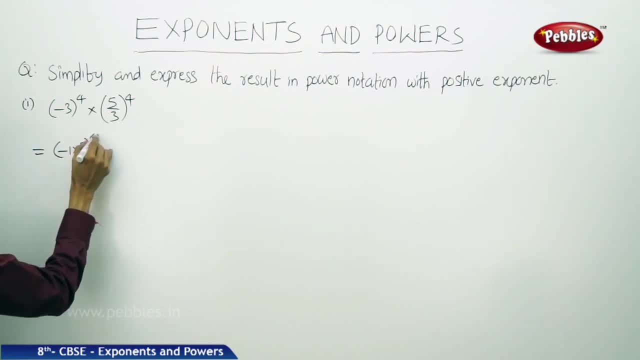 1 into 3 over to the power of 4, into Now 5 by 3 over to the power of 4 is same. Now this is according to a into b over to the power of m. So this is a power, m into b power. 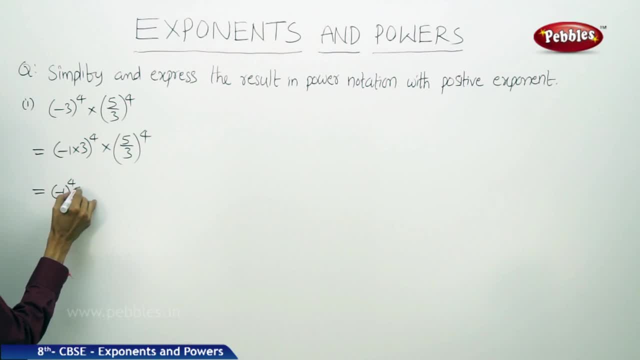 m. So we can write that minus 1 over to the power of 4 into 3 over to the power of 4 into Now. this is according to the formula a into b over to the power m, equal to a power m by b power m. So we can write that 5 power. 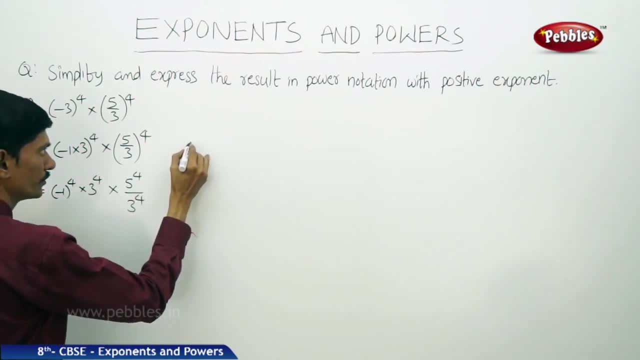 4 by 3 power 4.. So that 2 laws used here are: a into b over to the power. m equals to a power, m into b power m And a by b over to the power m equals to e to the power of m, by b to the. 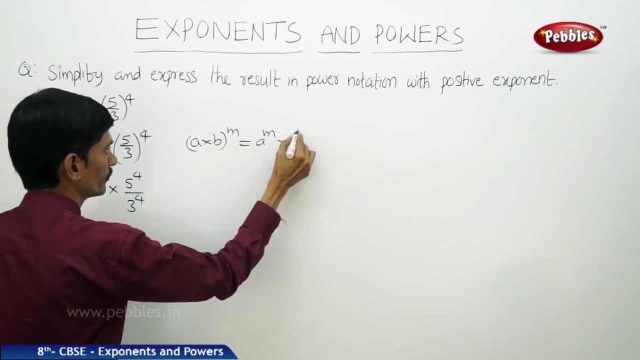 power m Now minus 1 over to the power of 4 into 8, over to the power m by m at the power m can be written as minus that. So that is has something else. So already, when you write that, then you have to do the same thing. Awesome, Well, this is an expression. 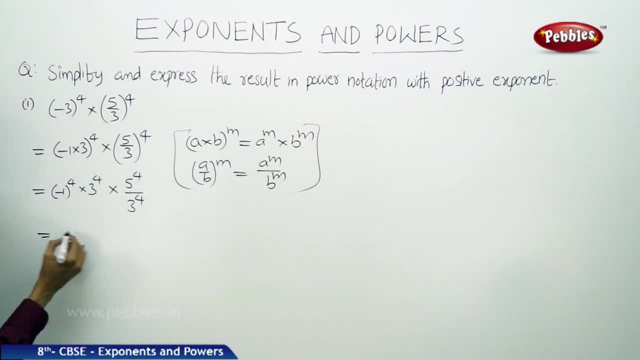 4,. if minus 1 is multiplied 4 times, so then we will get 1 into 3, power 4 is 81, when 3 is multiplied 4 times, we get 81 into 5. power 4 by 3, power 4 also 81, so 3 power 4 equals. 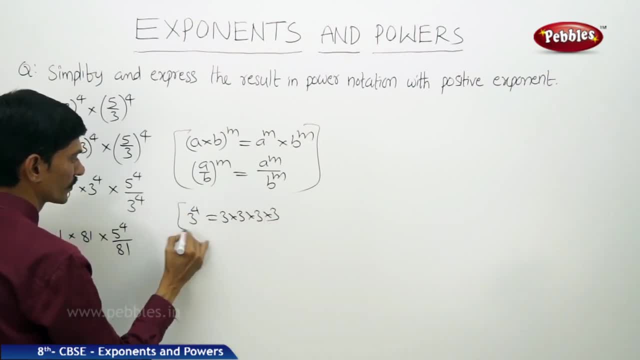 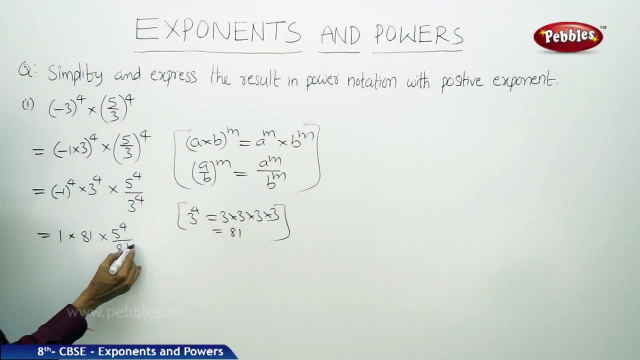 to 3 into 3, into 3 into 3, so this equals to 3, 3 is 9, 9, 3 is 27, 27, 3 is 81, now here 81, 81 get cancelled. this equals to 5, to the power of 4, now here 5 power 4, here the. 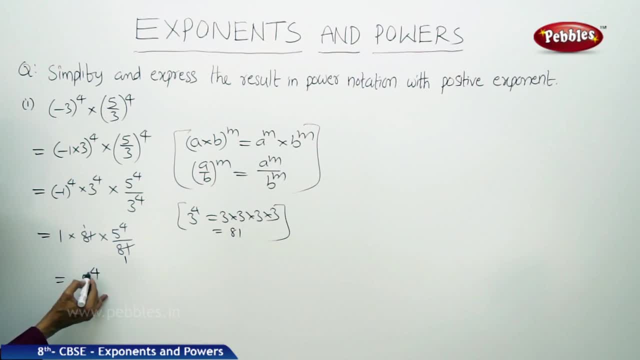 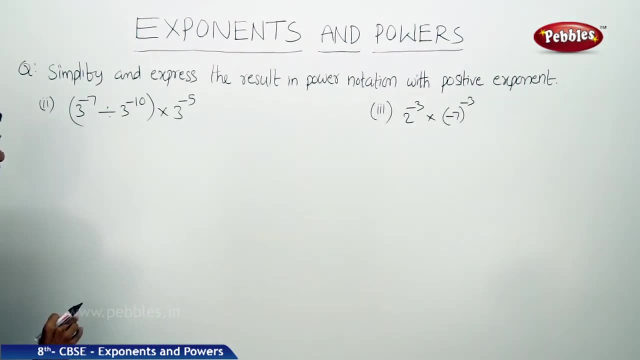 power is positive exponent. the power exponent 4 is the positive exponent. now the second question: 3 power minus 7 divided by 3.. Now 3 power minus 7 into 3 to the power of minus 5, now this equals to 3 power minus. 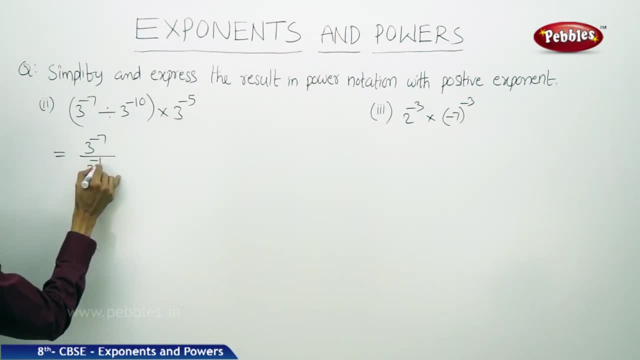 7 divided by 3 power minus 10, and which is multiplied by 3 power minus 5, now this equals to a power m by a power n. so this equals to a, to the power of m minus n. now here we can write: 3 power minus 7.. 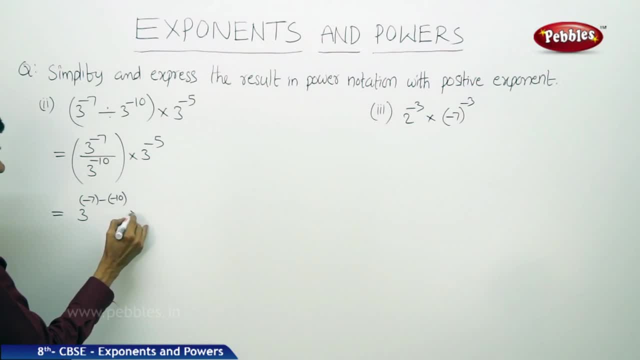 of minus 10 into 3 to the power of minus 5.. Now this equals to here: 8 to the power of m, by 8 to the power of n. equals to 8 to the power of m minus n. Now 3 to the power of. 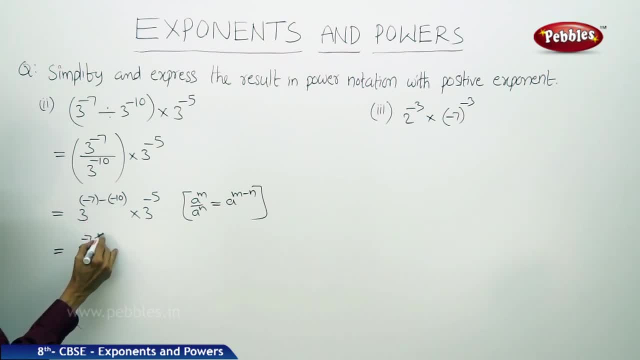 minus 7 minus into minus plus 10 into 3 power minus 5 can be written as 1 by 3 to the power of 5.. Since 8 to the power of minus n equals to 1 by 8 to the power of n, Now this equals: 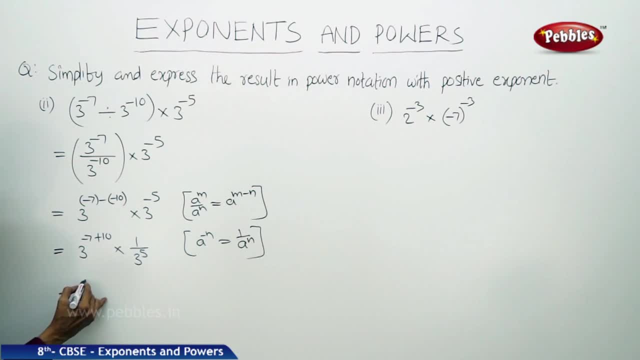 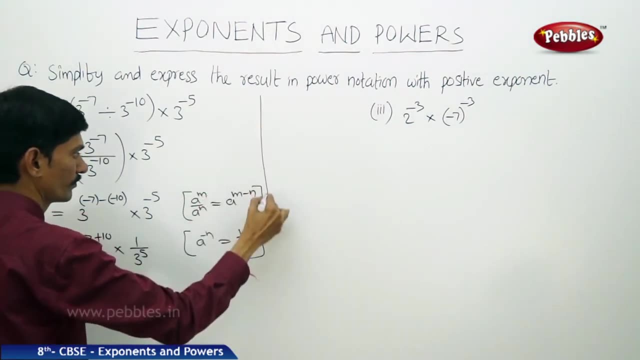 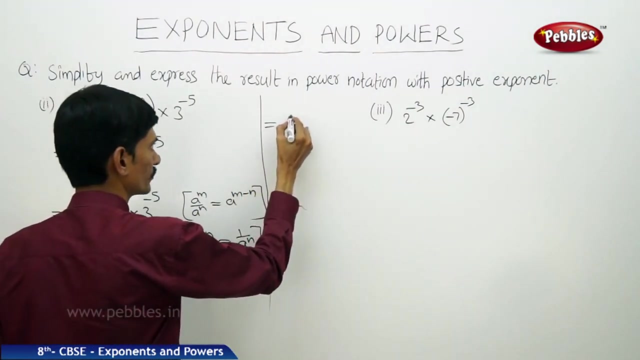 to 3 to the power of 10 minus 7 is 3 into 1 by 3 to the power of 5.. Now this equals to 3 power 3 into 1 is 3 power 3.. Again, we use the same formula. So 3 power 3 minus 5. a power m by a power n is a to the. 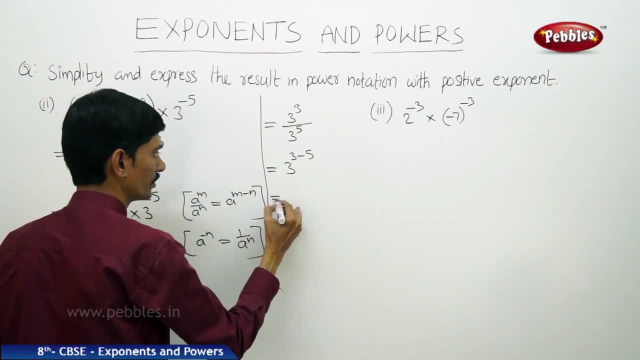 power of m minus n. So we use 3 power 3 minus 5.. This equals to 3 to the power of 3 minus 5 is minus 2.. Again, we use this formula: 3 power, a power minus n is a to the power of. 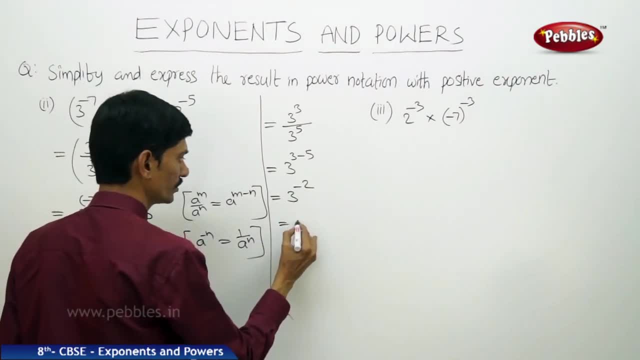 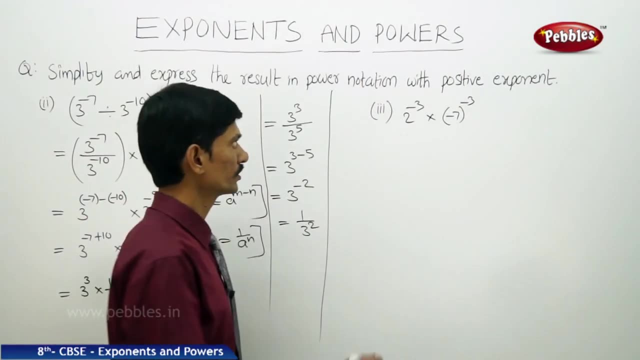 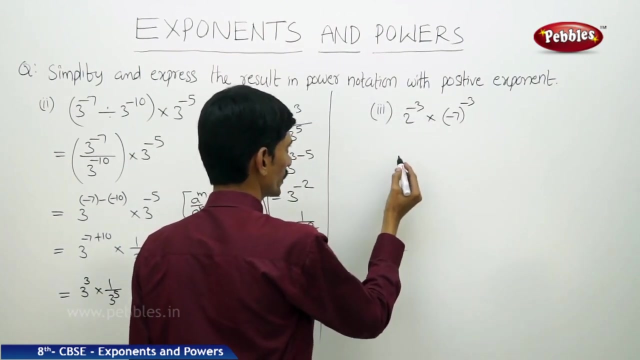 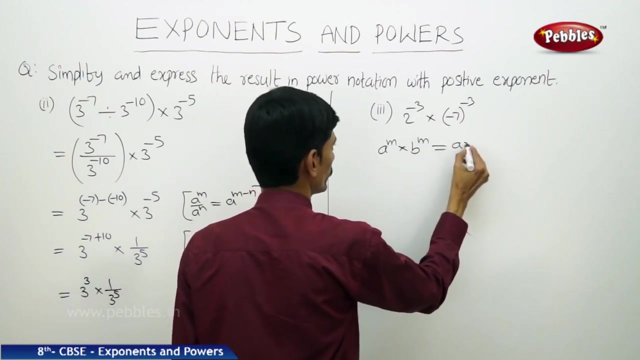 minus 7.. Now we will solve the third question. What is a to the power of m minus 7 minus 3.. Now this is according to the formula, a power m into b? power m equals to a into b. power of m. Now this equals to a to the power of m minus 3 into minus 7.. So we will solve the third question: a to the power minus 3 into minus 7, whole power minus 3.. Now this is according to the. 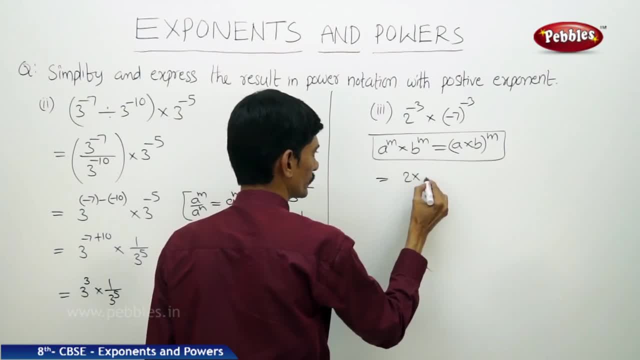 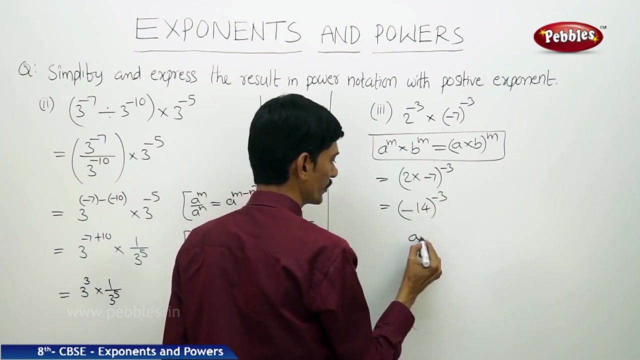 equals to 2 into minus 7, o to the power of minus 3.. So, plus into minus minus 2, 7 are 14, o to the power of minus 3.. Now this is, according to the formula, a power minus n. 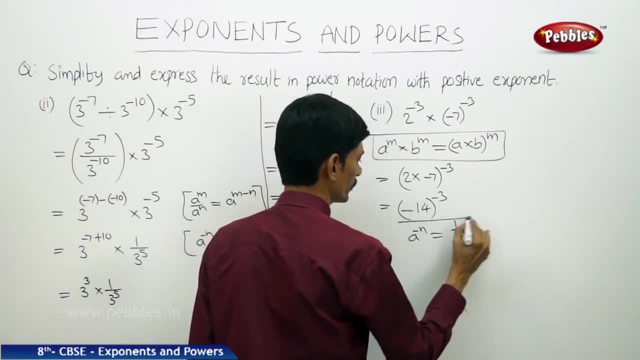 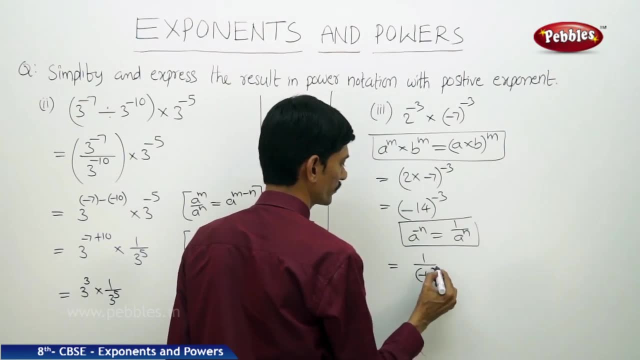 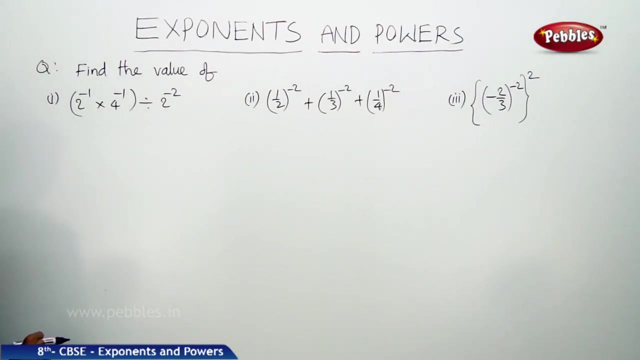 equals to 1 by a to the power of n. Now this equals to 1 by minus 14, o to the power of 3.. Now let us solve the next question. Find the value of 2 power minus 1 into 4 power. 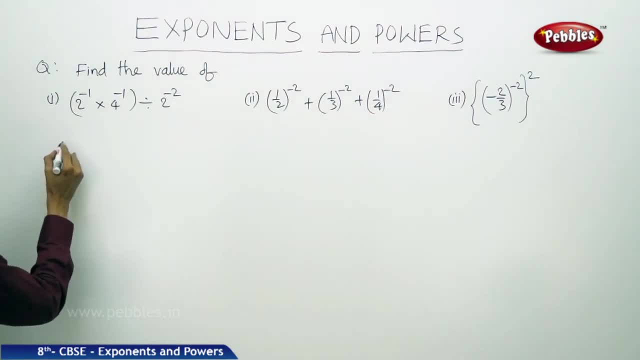 minus 1, divided by 2, to the power of minus 2.. Now this equals to: so we know that a power minus n is 1 by a to the power of n. So here we can write that 1 by 2 to the power. 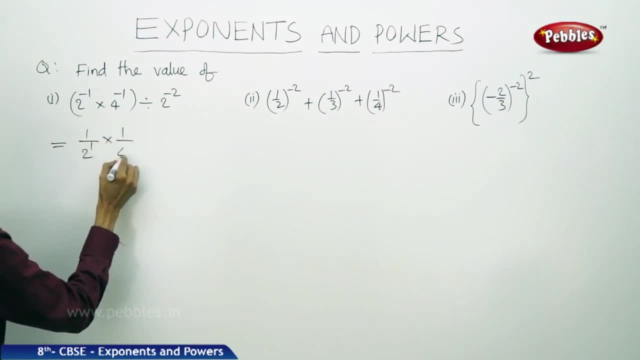 of 1 into 1 by 4 to the power of 1 divided by 1 by 2 to the power of 2.. Now this equals to 1 by 2 to the power of 1, means 2 into 1 by 4 divided by 1 by 4.. Now this: 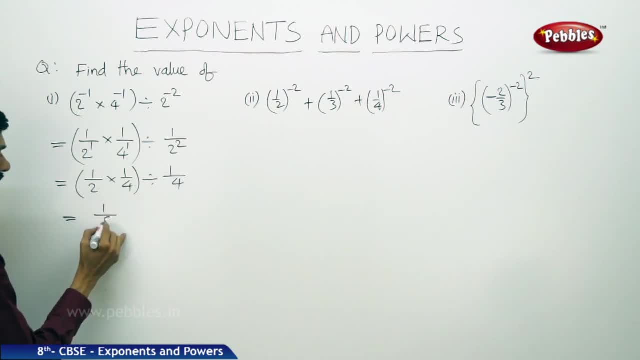 equals to 1. 1s are 1 by 2, 4s are 8 divided by 1 by 4.. This equals to 1 by 8.. Now we will take the reciprocal of 1 by 4. by multiplying into the reciprocal of 1 by 4 is 4 by 1.. 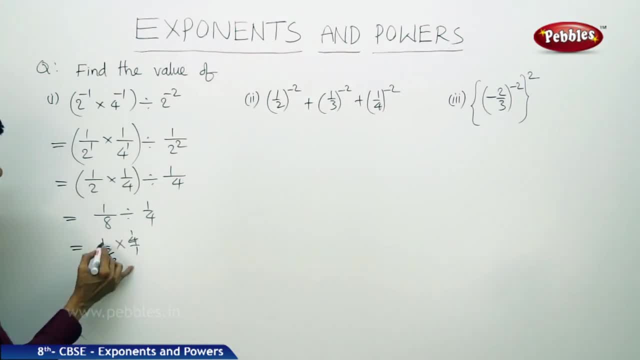 Now we can cancel 4. 1s are 4, 2s are. This equals to 1. 1s are 1 by 2, 1s are 2.. So here the law is: a to the power of minus n equals to 1 by a to the power of n. Next second question: 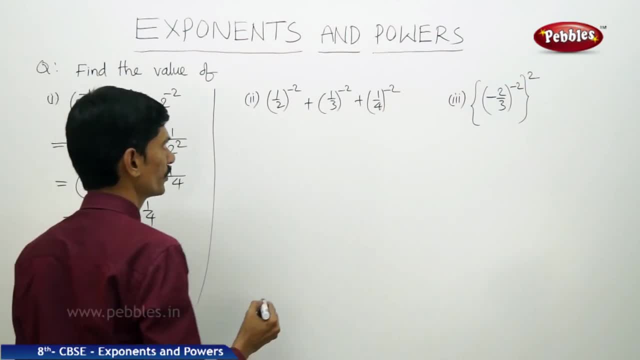 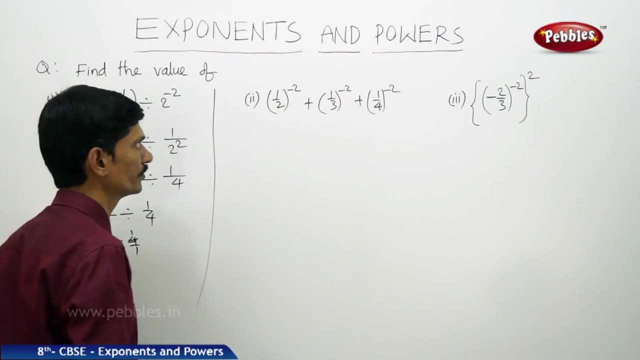 1 by 2 whole power minus 2 plus 1 by 3 whole power minus 2 plus 1 by 4 whole to the power of minus 2.. So a by b whole power minus m equals to b by a whole to the power of m. 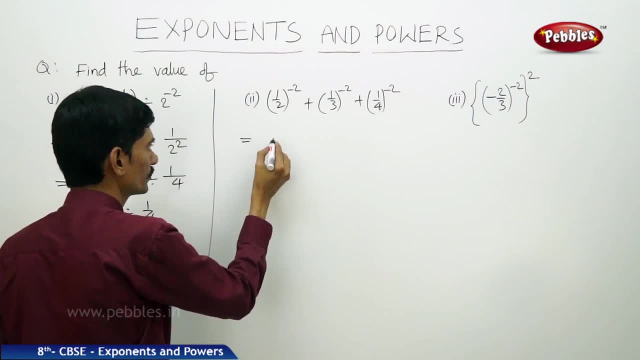 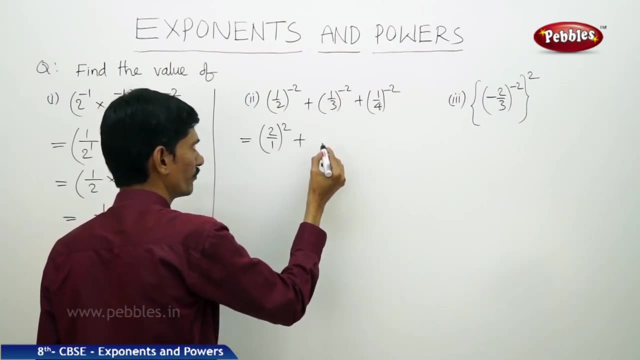 So this can be written as 1 by 2 whole power. minus 2 can be written as 2 by 1 whole to the power of 2 plus 1 by 3 whole to the power of minus 2 is 3 by 1 whole to the power of plus 2 plus 1 by 4 whole power. 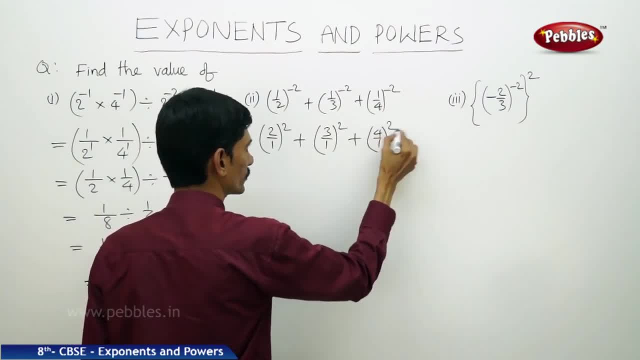 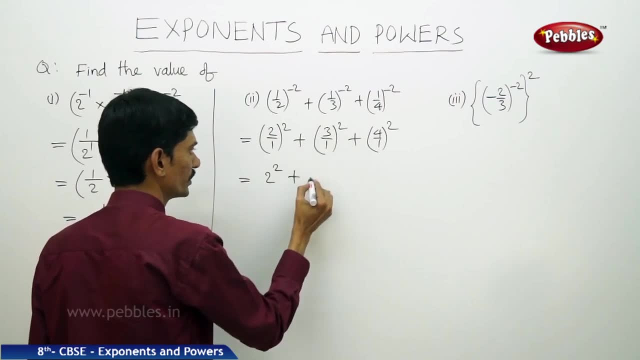 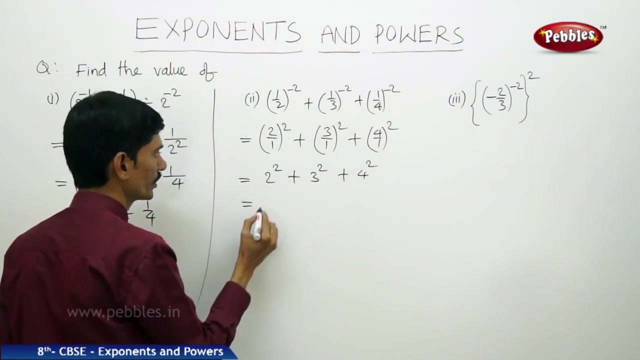 minus 2 is 4 by 1 whole to the power of plus 2.. Now 2 by 1 means 2 power. 2 plus 3 by 1 means 3 to the power of 2.. plus 4 by 1 means 4 to the power of 2.. Now 2 square is 4 plus 3 square is 9 plus 4 square. 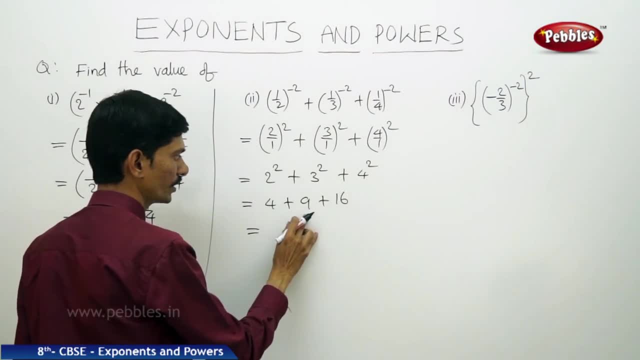 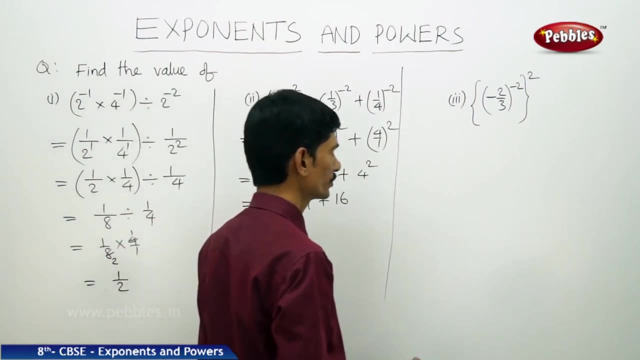 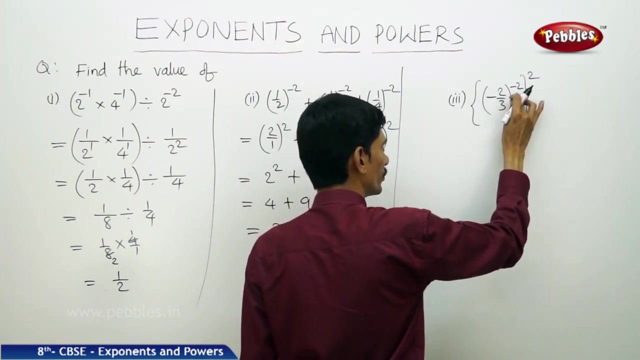 is 16.. Now 16 plus 9, 25,, 25 plus 4, 29.. Next, minus 2 by 3 whole power minus 2 whole to the power of plus 2.. So this is, according to the law, a power m whole to the power of. 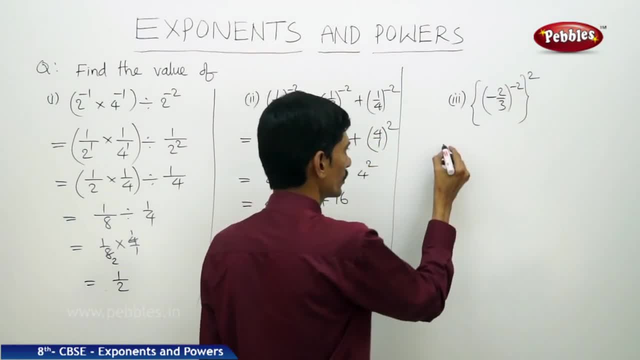 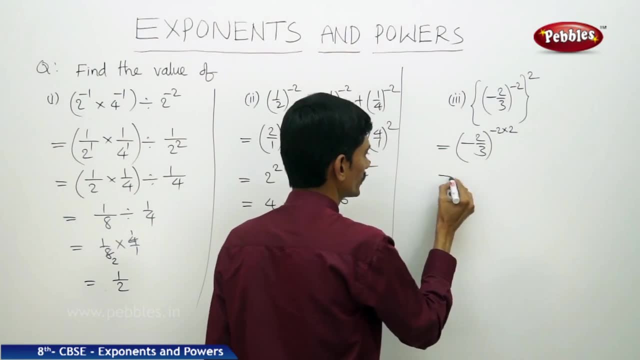 n. This equals to a to the power of m into n. Now this equals to minus 2 by 3 whole, to the power of minus 2 into 2.. This equals to minus 2 by 3 whole to the power of 2 twos. 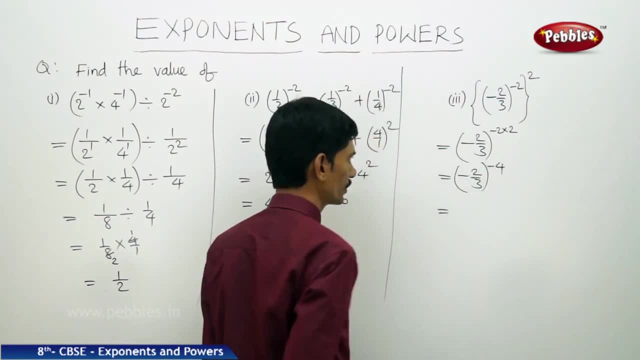 are 4.. So it is minus 4.. Now it is according to the law: a by b whole to the power of minus m equals to b by a whole to the power of m. Now this can be written as minus 3 by 2 whole. 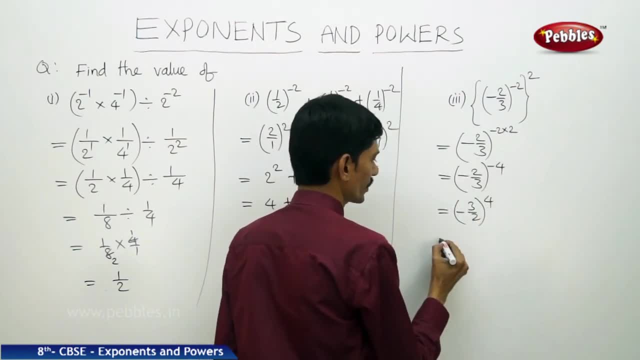 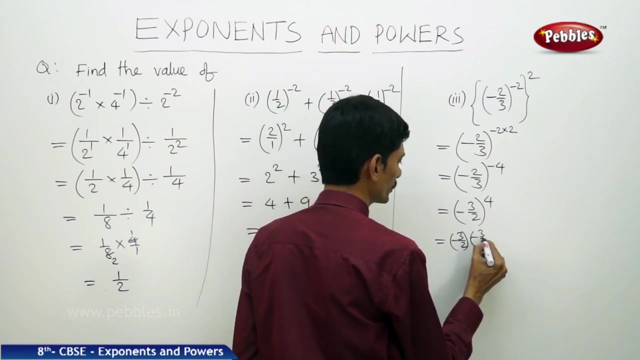 to the power of 12. of 4.. Now this equals to minus, to the power of even number is positive. So 3 power 4 by 2 power 4. or we can write that minus 3 by 2 into minus 3 by 2, into minus 3 by 2, into. 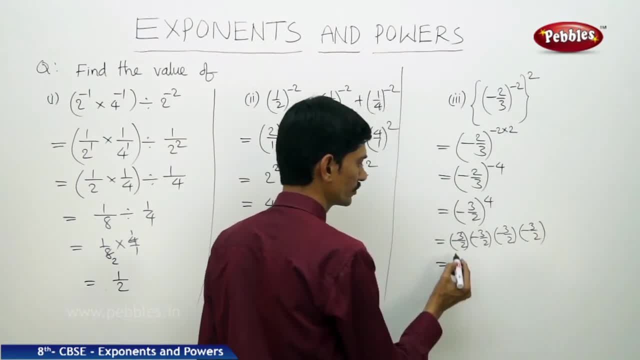 minus 3 by 2. This equals to minus into minus plus, plus, into minus, minus, minus into minus plus. So overall we will get the positive. Now, 3, 3 is 9,, 9, 3 is 27,, 27, 3 is 81 divided. 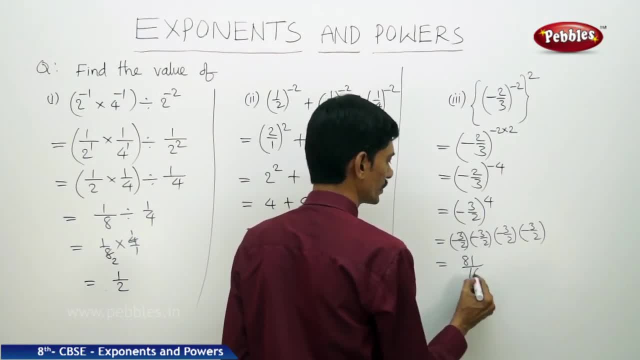 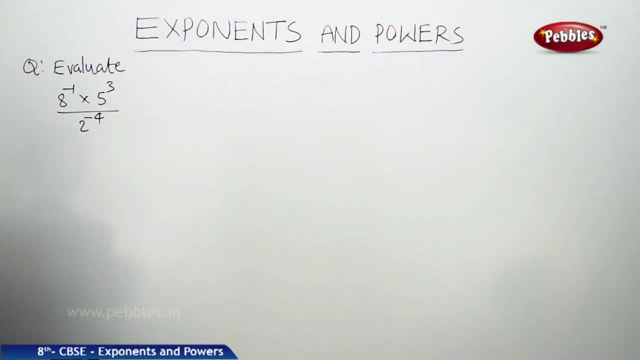 by 2, 2 is 4, 4, 2 is 8, 8, 2 is 16.. Now we will solve the next question. Evaluate 8 to the power of minus 1 into 5 to the power of 3, divided by 2 to the power of minus 4.. Now 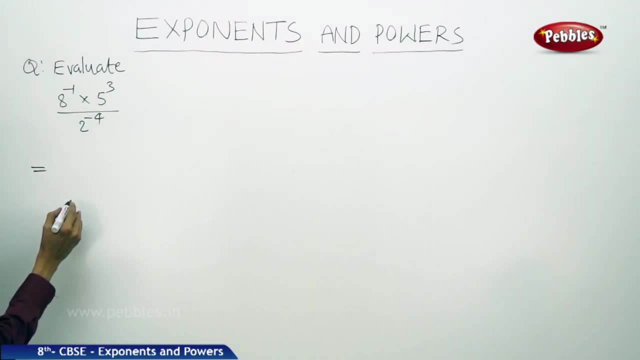 this equals to 8 to the power of minus 1. can be written as 1 by 8 to the power of 1.. So this is 1 by 8 to the power of minus 1 into 5 to the power of 3 into 2 power minus. 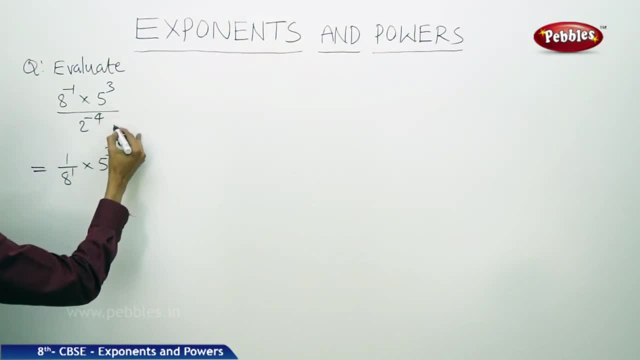 4 can be written as see. this is 1 by 2 to the power of minus 4.. When it comes to the numerator, it becomes 2 to the power of 4.. So here we are using the law 8 to the power. 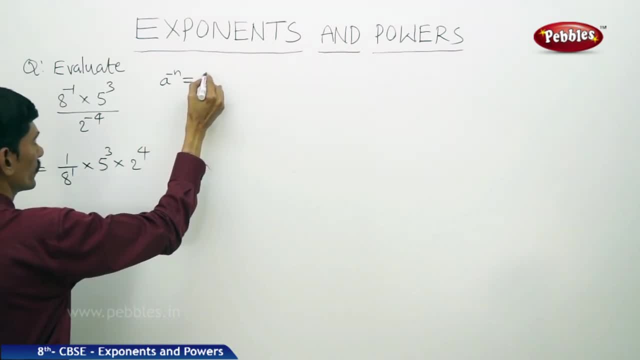 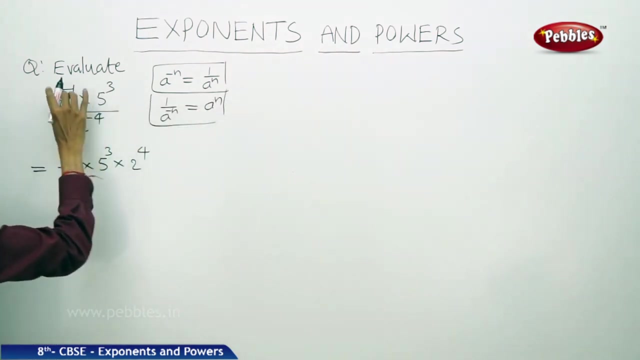 of minus n equals to 1 by 8 to the power of n, And 1 by 8 to the power of minus n equals to 8 to the power of n. So we have changed the negative exponents as the positive exponents. 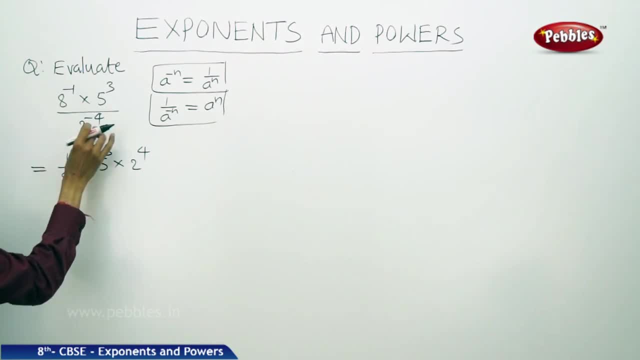 So we have sent this to the denominator and we have sent this to the numerator. Now this equals to 1 by 8, to the power of 1 means 8 into 5 cube. 5 is multiplied 3 times 5 into. 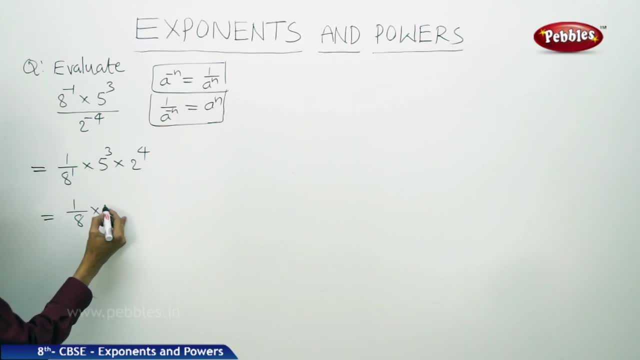 5 into 5.. So it is 5, 5 is 25, 25, 5 is 125,, 125 into 2 to the power of 4 is 16.. Means 2 is multiplied 4 times. So now you can cancel 8. 1s are 8,. 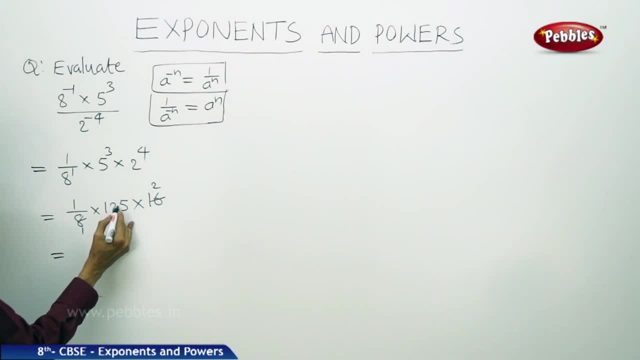 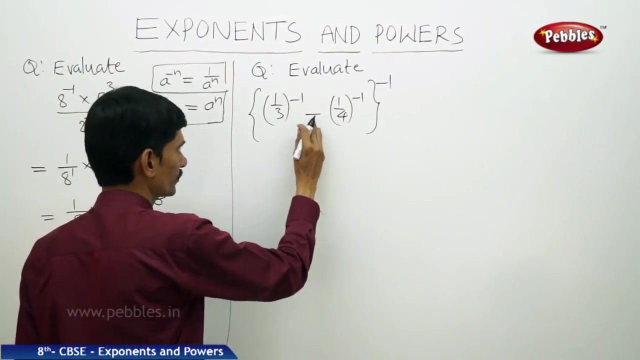 8 2s are 16.. Now this equals to 125. 1s are 125 into 2.. Now this equals to 250.. 125 2s are 250.. Now let us solve the next question. Evaluate 1 by 3, 1 to the power of minus 1. 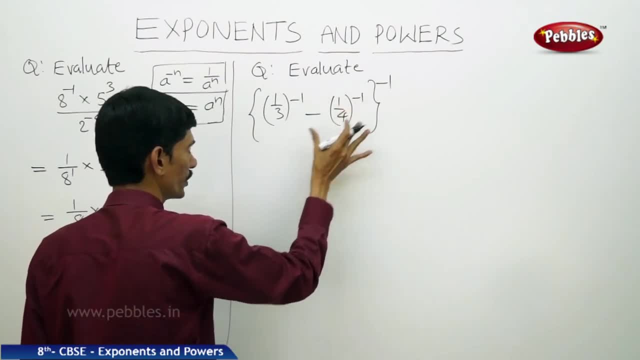 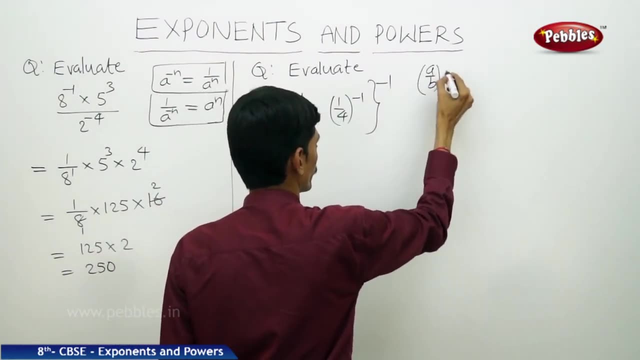 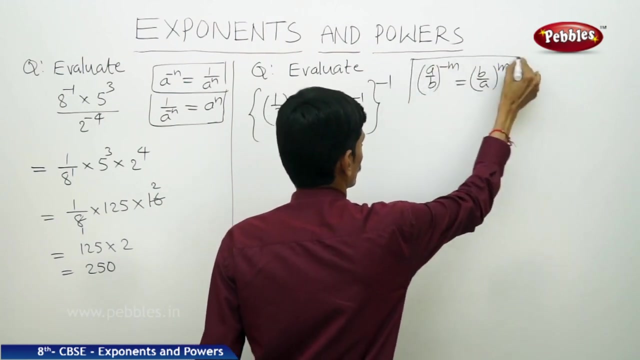 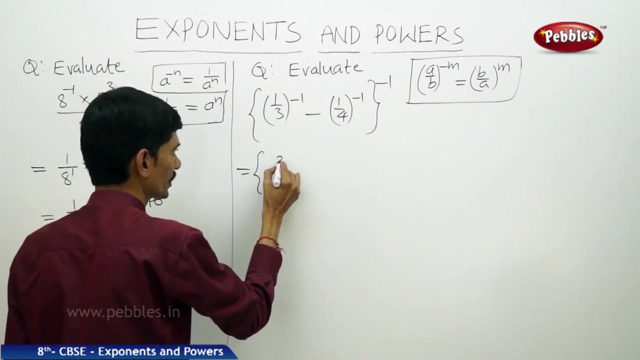 minus 1 by 4: 1 to the power of minus 1, whole to the power of minus 1.. So here we can use the law of exponents: a by b, whole to the power of minus m equals to b by a whole to the power of m. Now here, 1 by 3 whole to the power of minus 1 means: 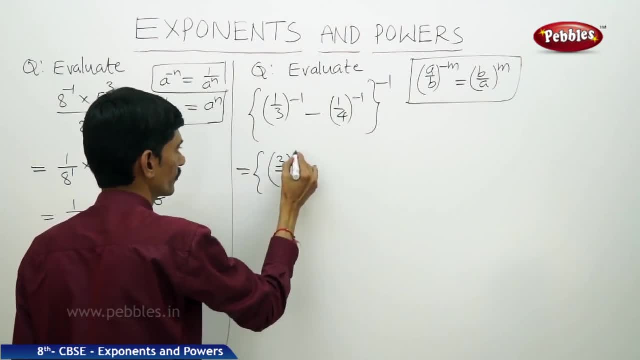 it can be written as: 3 by 1 whole to the power of 1 minus 1 by 4 whole to the power of minus 1 can be written as 4 by 1 whole to the power of minus 1.. So here we can use the law of: 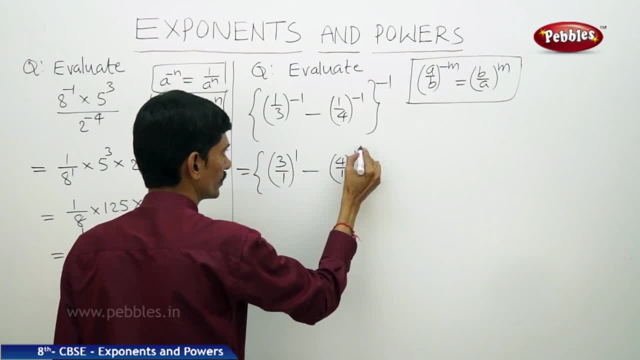 exponents: a by b whole to the power of minus m equals to b by a whole to the power of m by 1 whole to the power of plus 1.. Again, whole to the power of minus 1.. Now this equals: 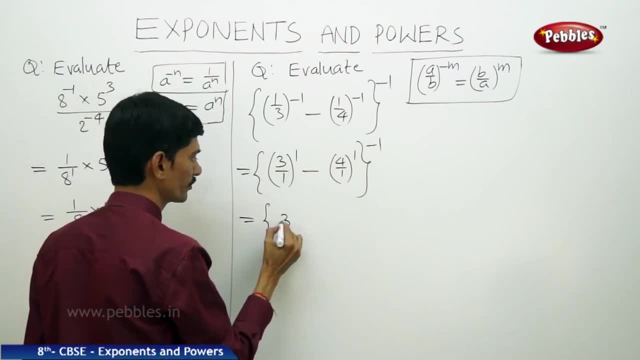 to 3 by 1 means 3 to the power of 1 minus 4. by 1 means 4 to the power of 1, whole to the power of minus 1.. This equals to 3 to the power of 1, means 3 minus 4 to the power. 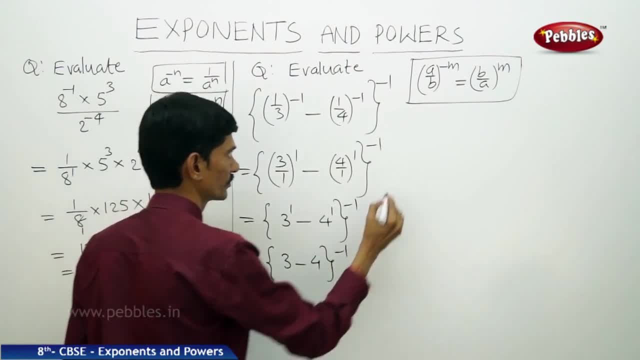 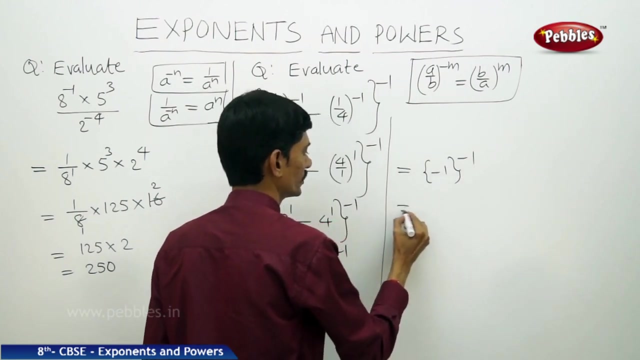 of 1 means 4, whole to the power of minus 1.. This equals to 3 power no 3 minus 4, it is minus 1, whole to the power of minus 1.. This equals to- here we can use a- to the. 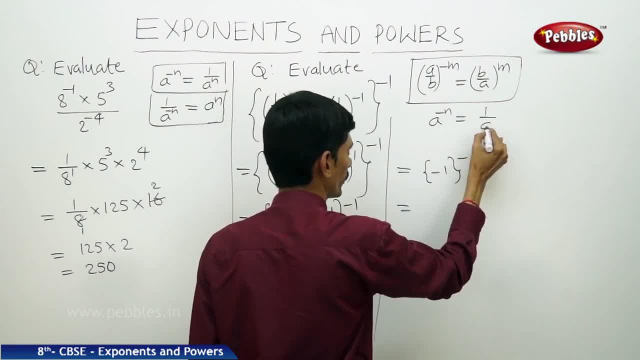 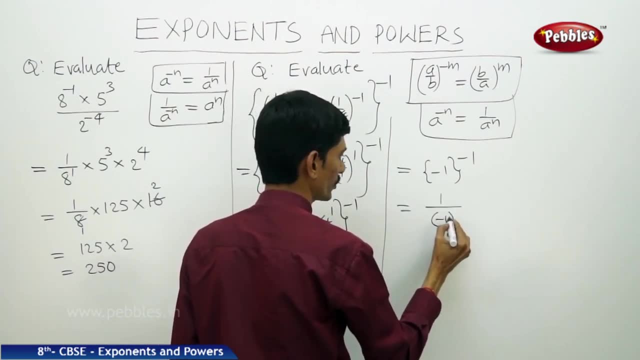 power of minus n equals to 1 by a to the power of n. So this equals to 1 by minus n. So minus 1 whole to the power of minus 1 is same as 1 by minus 1 whole to the power. 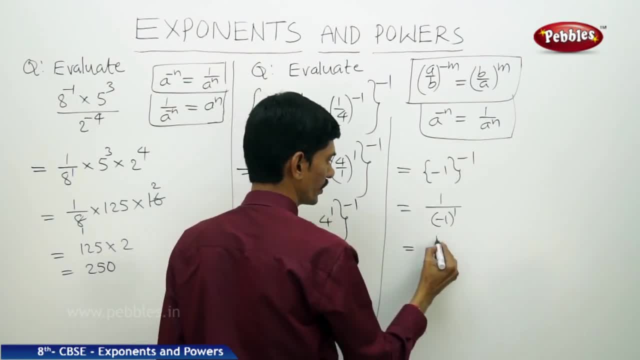 of 1 according to this law. Now this equals to 1 by minus 1 whole to the power of 1 means minus 1.. This equals to minus 1 by 1 means 1.. Now the next question is: simplify 3 to. 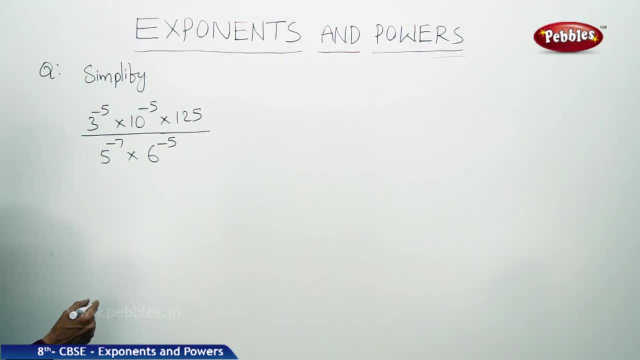 the power of minus 5 into 10 to the power of minus 5 into 125. divided by 5 to the power of minus 7 into 7.. In case 1 minus 1 equal to 100 into 10 to the power of minus 5 to the power of 1 minus. 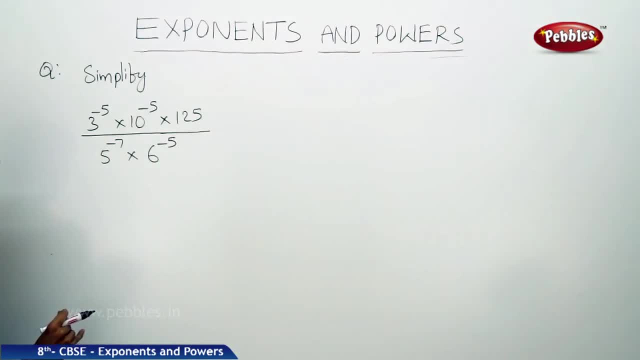 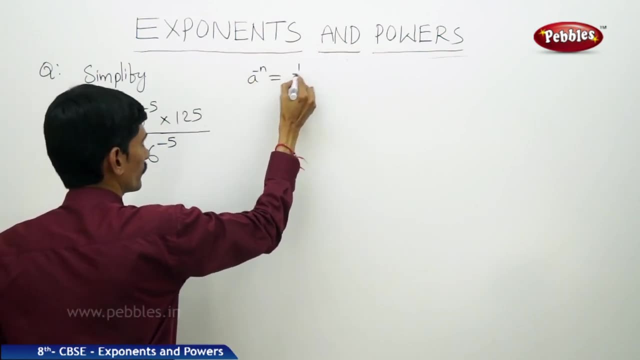 6 to the power of minus 5.. Now, first you will convert all the negative exponent as the positive exponent using this 2 laws: a to the power of minus n equals to 1 by a to the power of n, or 1 by a to the power of minus n equals to a to the power o n. Now this: 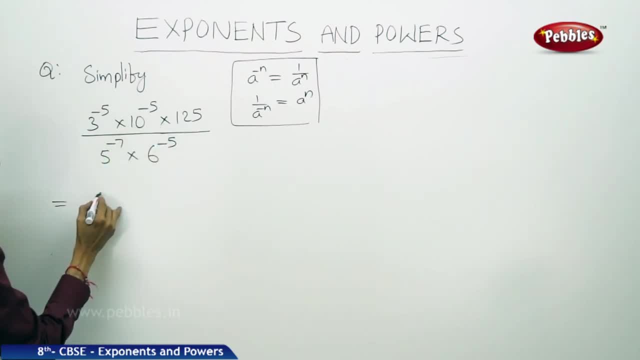 equals to 125 is same into 1 over 80 to the power of minus n. equals to 5 power over minus n. 2�, 2E, 2N, 4 minus 7, I am writing in the numerator. then it becomes 5 to the power of 7 into 6 to the. 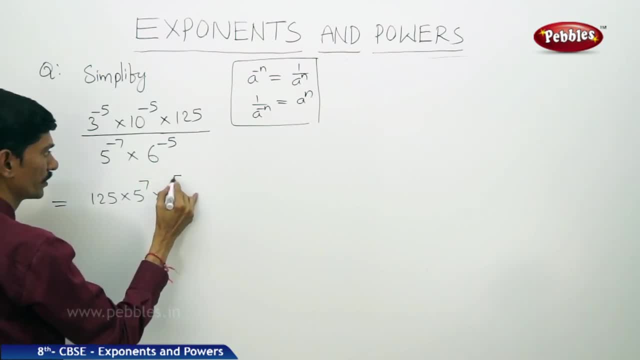 power of minus 5, I am writing in the numerator: it becomes 6 to the power of 5 divided by now 3 power minus 5, I am writing in the denominator: it becomes 3 to the power of 5 into 10 power. 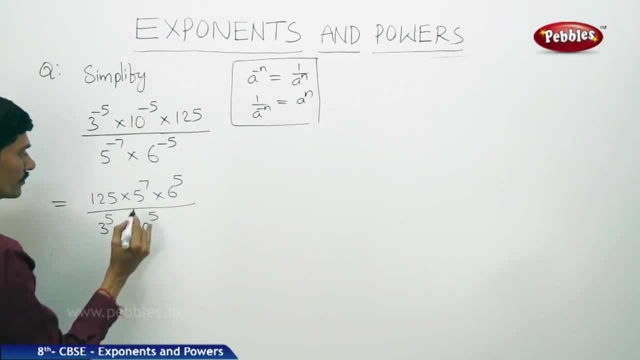 minus 5, in the denominator it becomes 10 to the power of 5, now this equals to now: 125 can be written as 5 to the power of 3 into 5 to the power of 7 into 6 can be written. 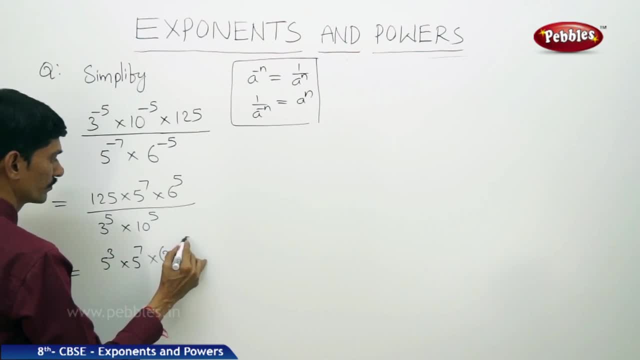 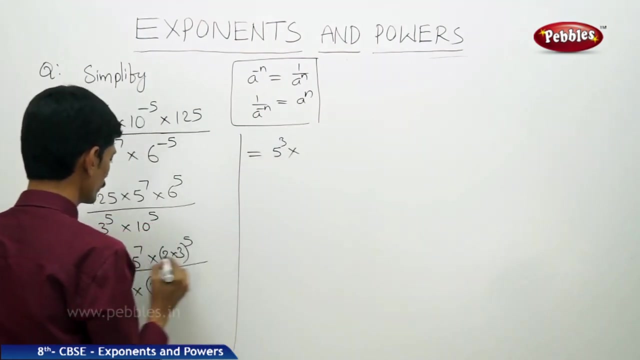 as 2 into 3. whole to the power of 5 divided by 3. power 5 into 10. power 5, 10 can be written as 2 into 5.. Now this equals to 5 power 3 into 5, power 7 into now. this is according to the law. 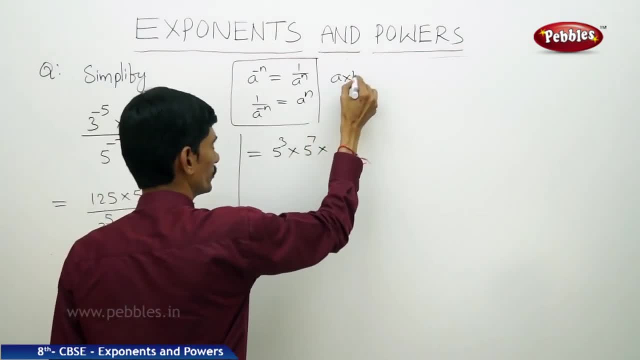 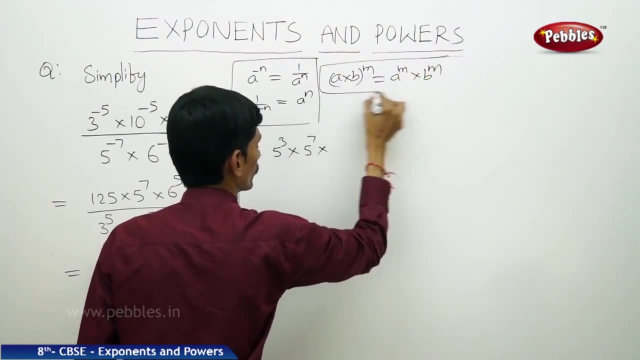 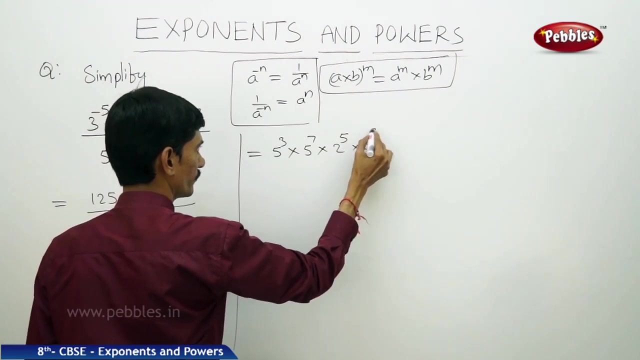 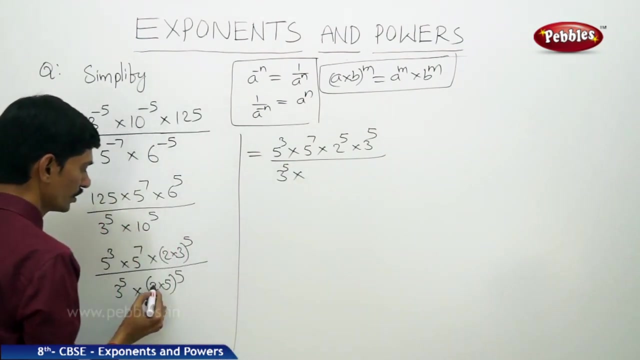 a into b whole power m, a into b whole power. m equals to a power m into b, to the power of m. Now this equals to 2 power 5 into 3, to the power of 5 divided by 3 power 5 into now here. 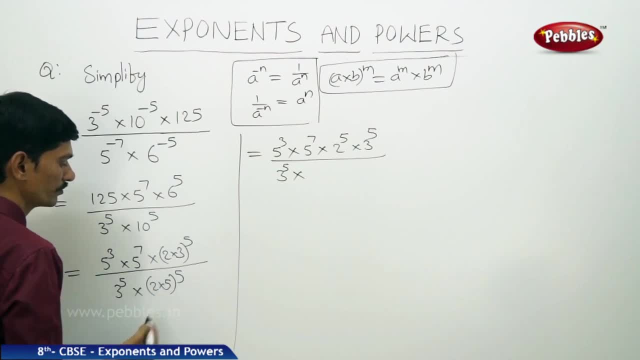 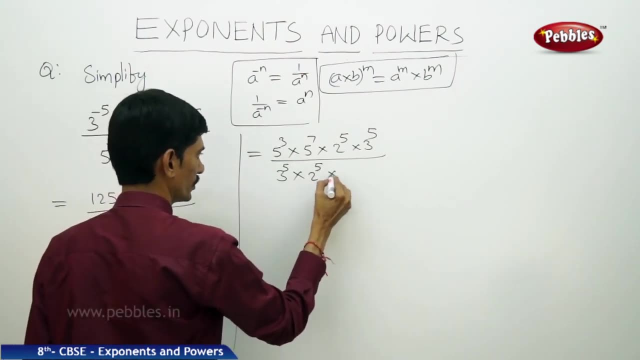 also we can use the same law a into b, whole to the power of m is equal to a to the power of m, into b to the power of m. so you can write 2 power 5 into 5 to the power of 5.. 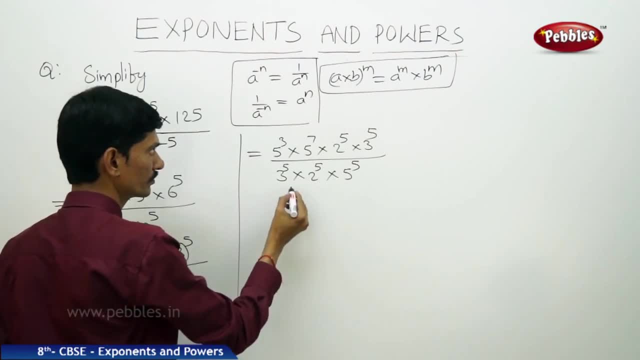 Now here we can cancel 3 power 5, 3 power 5, and we can cancel 2 power 5, 2 power 5, this equals to here: 5 power 3 into 5 power 7, so this equals to 5, to the power of 3 plus. 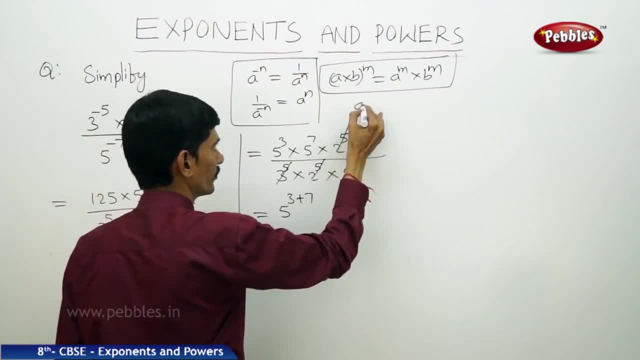 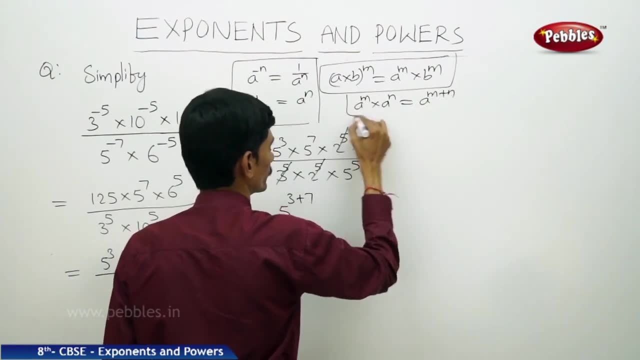 7, because a to the power of m into a to the power of n equals to a to the power of m plus n. Now this equals to 5 to the power of m, divided by 5 to the power of 5, now this equals to: 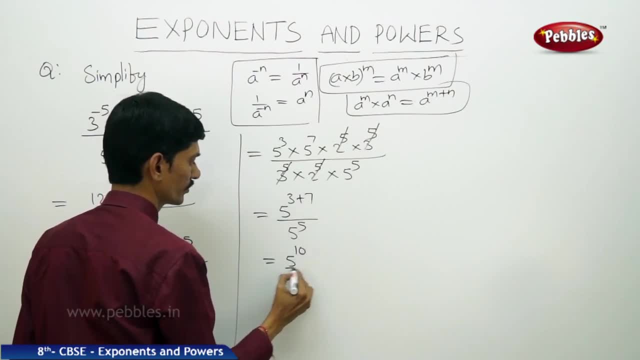 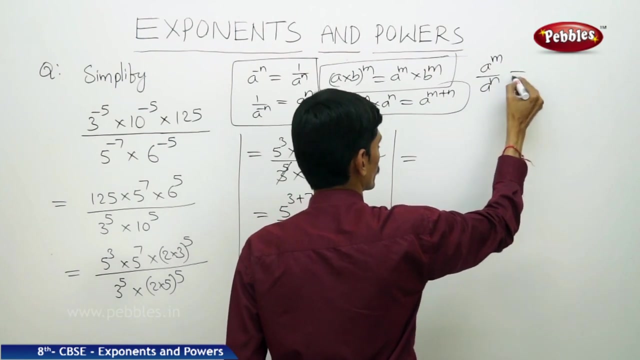 5 to the power of 3 plus 7 is 10 by 5 to the power of 5.. Now this equals to- again this is in the form: a power m by a power n. so a to the power of m minus n, a to the power of m divided by a to the power of n m minus n. now here: 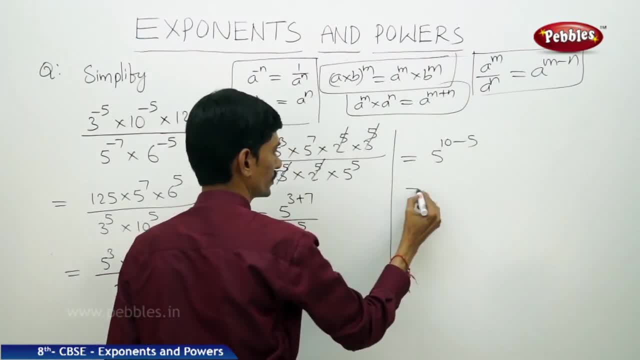 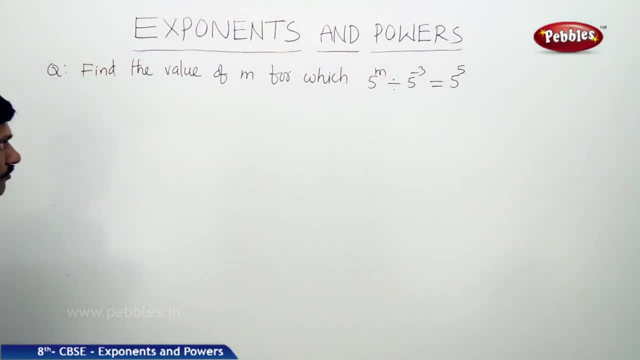 we can write 5 to the power of 10 minus 5.. This equals to 5 to the power of 5.. Now the next question: find the value of m, for which 5 to the power of m divided by 5 to the power of minus 3. 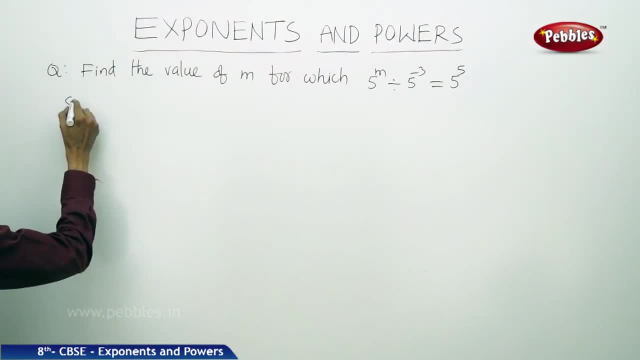 equals to 5 to the power of 5.. Now let us solve the equation and find the value of m Now: 5 to the power of m. divided by 5 to the power of minus 3 equals to 5 to the power. 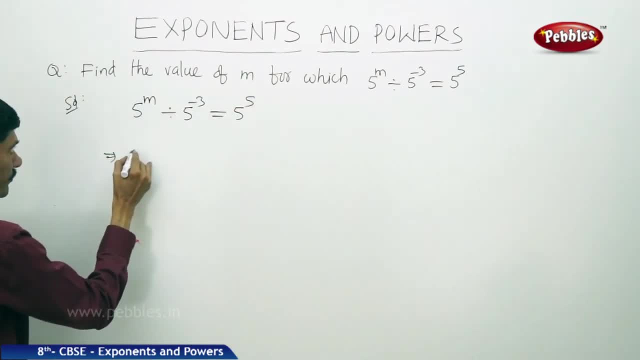 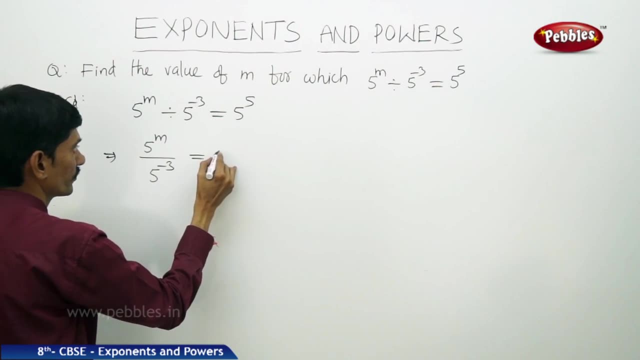 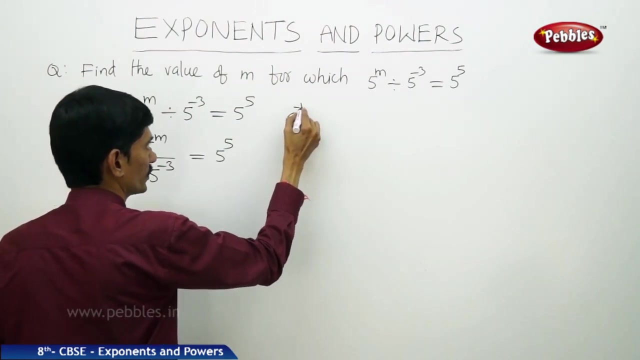 of 5.. Now this can be written as: 5 to the power of m by 5 to the power of minus 3 equals to 5 to the power of 5.. Now, as you know that 8 to the power of minus n equals to 1 by 8. 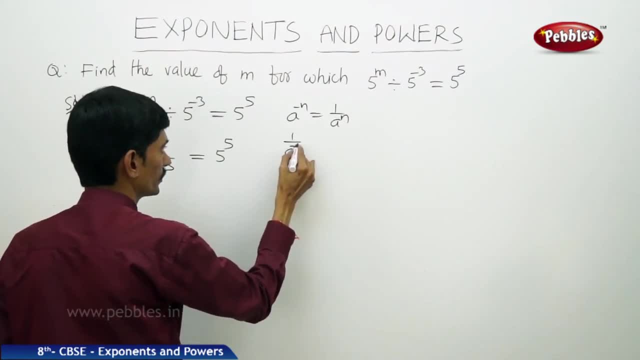 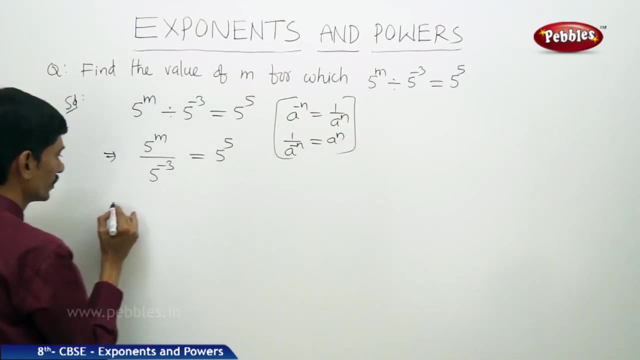 to the power of n, or 1 by 8 to the power of minus. n equals to 8 to the power of n. Now we can apply the second law here. Now this can be written as 5 to the power of m by 5. 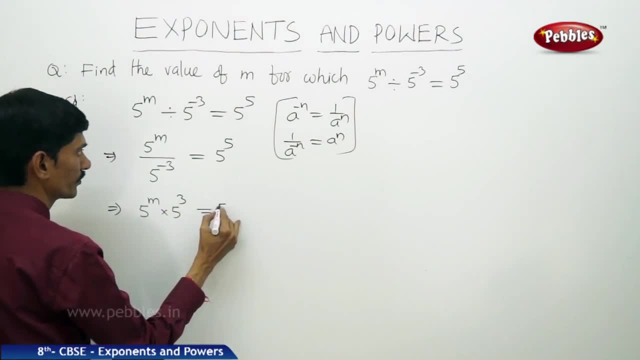 to the power of 3. This equals to 5 to the power of 5.. Now, which implies 5 to the power of m by 3 equals to 5 to the power of 5.. Here we can use this formula: 8 to the power of. 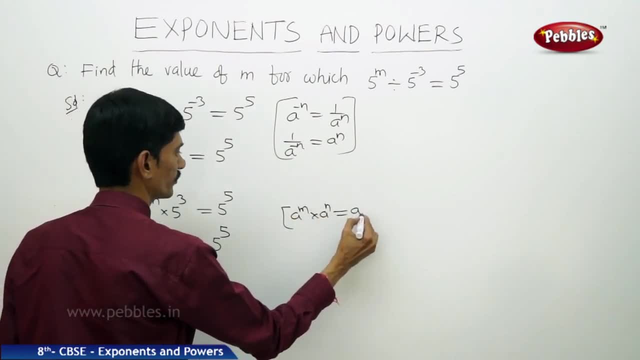 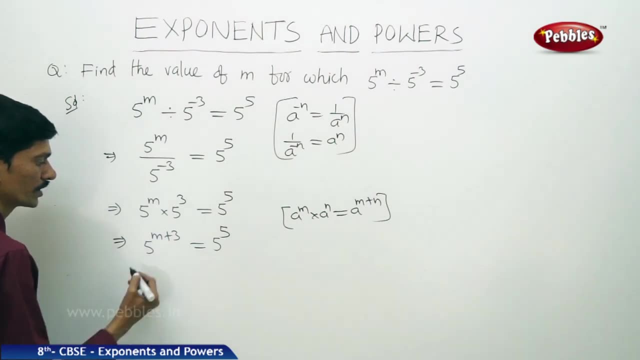 m by 8 to the power of n equals to 8 to the power of m by n. Now, when the bases are equal on both sides, then we can equate the exponents. So then m plus 3 equals to 5.. So when bases are equal on both sides of the equation, then exponents 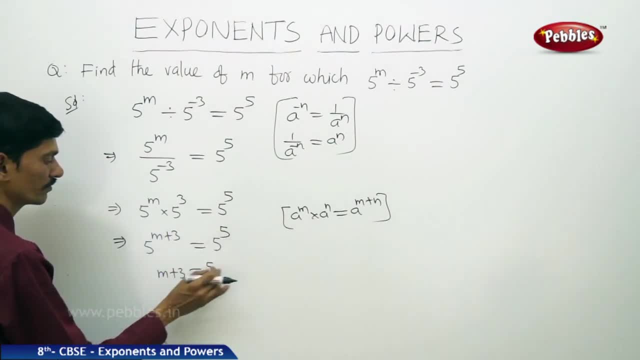 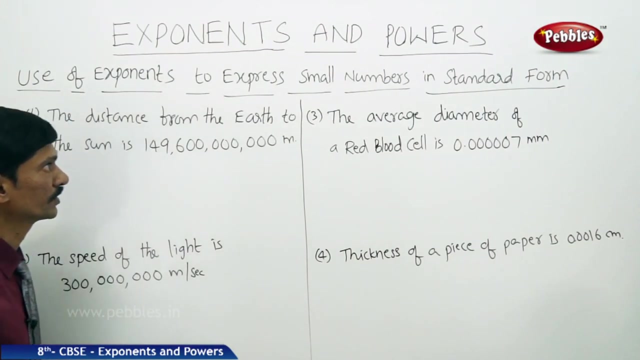 must be equal. Then m plus 3 equals to 5.. So then m equals to 5 minus 3.. So m equals to 5 minus 3.. 5 minus 3 is 2.. In the present chapter, exponents and powers, so far we have discussed about the 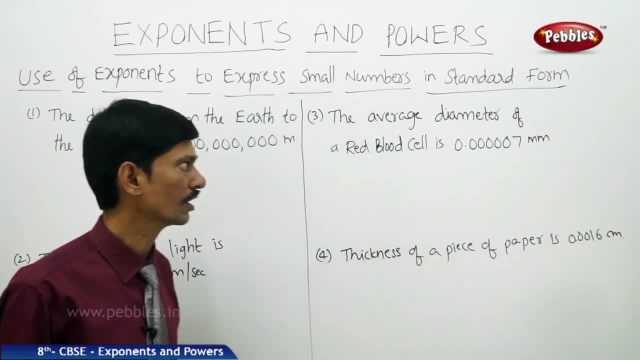 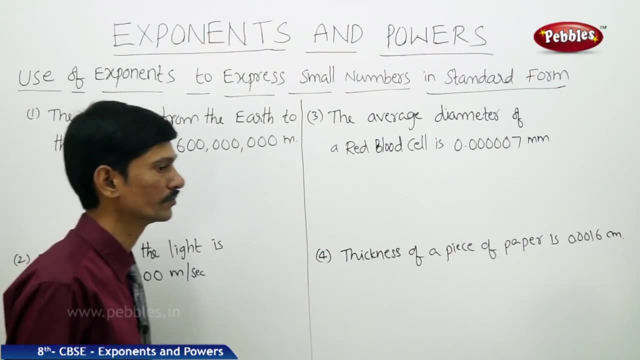 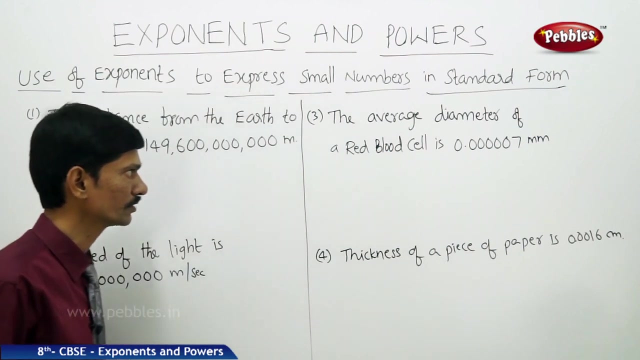 loss of exponents and we have done some problems using the loss of exponents. Now we will move to use of exponents to express small numbers in standard form. So while writing small numbers or very large numbers in the standard form, we can use the loss of exponents. Now let us see. 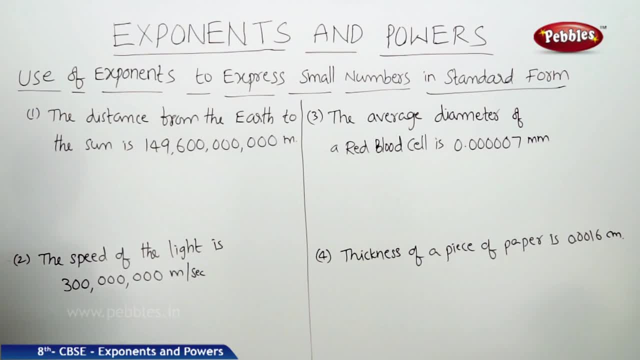 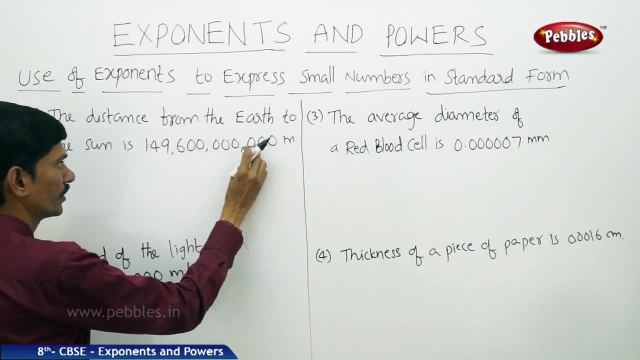 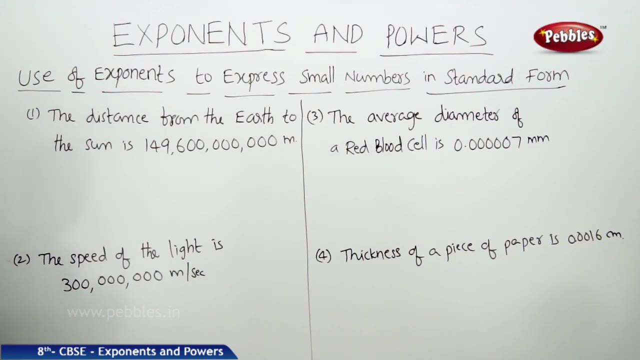 some facts. The distance from the earth to the sun is 1496 after 1496, 1,, 2,, 3,, 4,, 5,, 6,, 7, 8 zeros, So this is very large value. Then how to represent this larger value in the standard form? 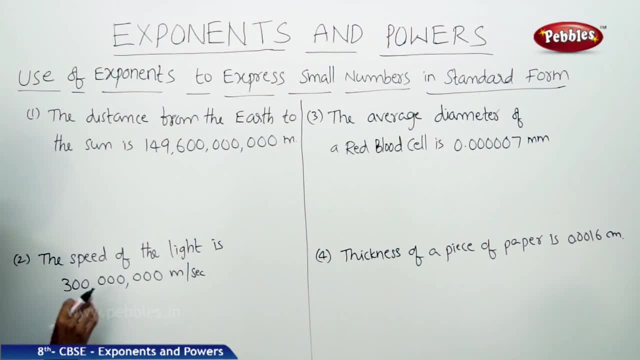 And the speed of the light is after 3,. how many zeros are there? 1,, 2,, 3,, 4,, 5,, 6,, 7,, 8.. So there are 8 zeros after 3.. So this is also very large. 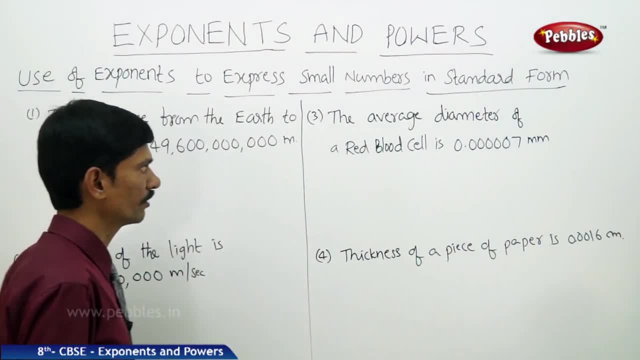 And the next one. the average diameter of a red blood cell is 0.00007 millimeters, So this is very smaller value, And the thickness of a piece of paper is 0.0016 centimeters, So these two are. 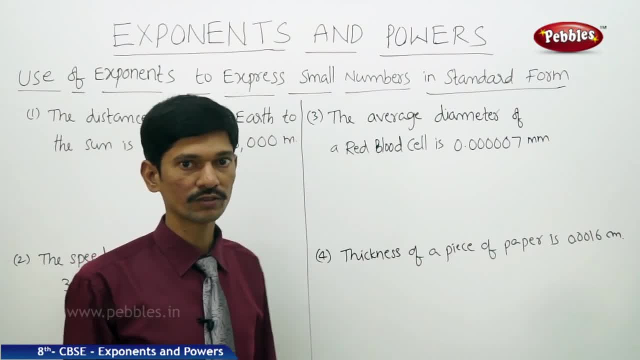 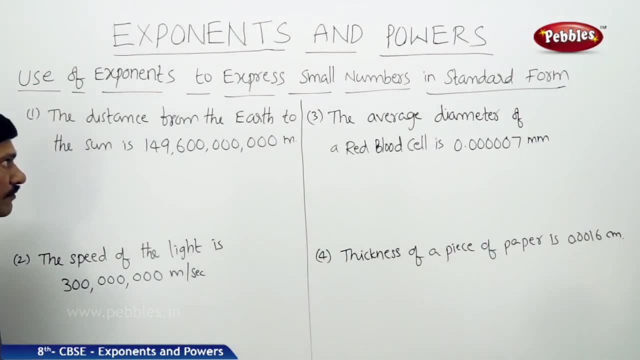 very smaller values. So how to represent the large values and the small values in the standard form By using exponents means the loss of exponents. Now the distance from the earth to the sun is. So let us see the first question, That is: 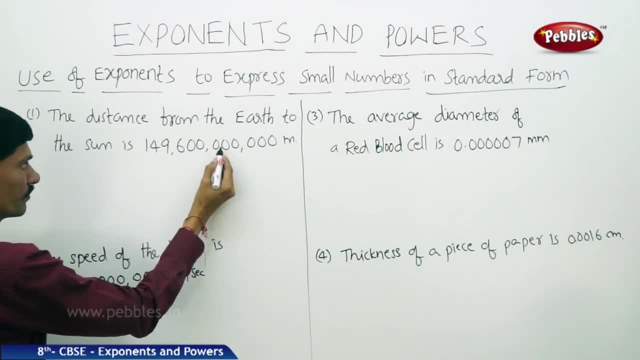 after 1496, there are 2 plus 3, 5 plus 3, 8 zeros. Now this can be written as into 10 to the power of 8 meters. Now this equals to: Now we will. 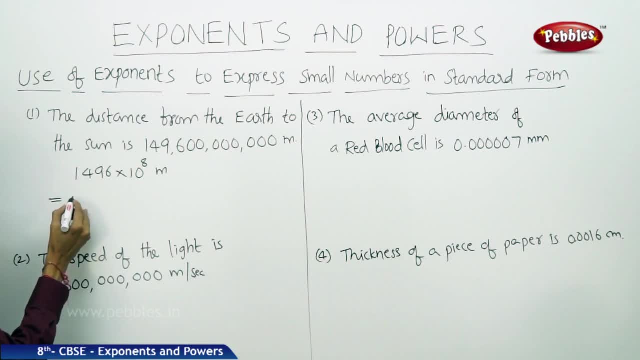 take the decimal point before 3 digits from right. So we will write 1.496 into 10 to the power of 8 plus 3.. Because the decimal point is shifted from units place to 3 digits left side. So we have taken 10 to the power of 3 here Now. 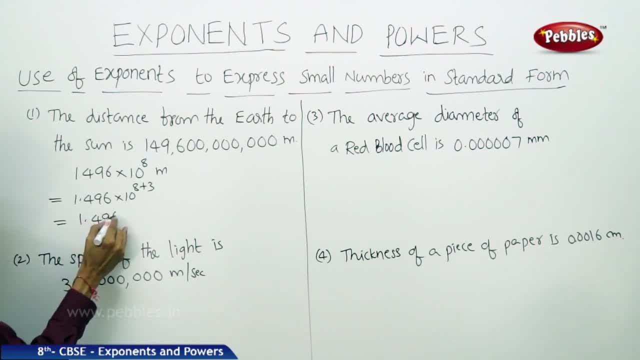 this equals to 1.496 into 10, to the power of 8 plus 3 is 11 meters. Next, the speed of the light is. Now see how many zeros are there after 3 here: 3 plus 3,, 6,, 6 plus 2,, 8.. 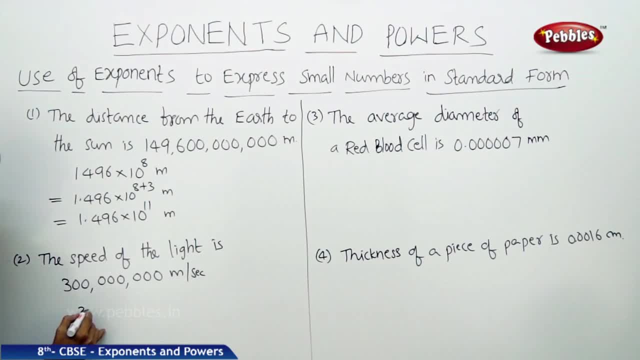 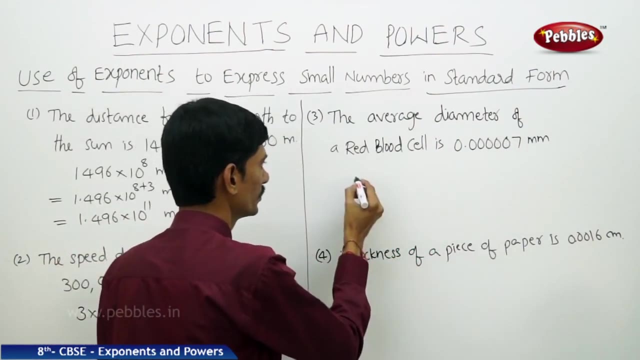 So there are 8 zeros. Now this can be written as 3 into 10, to the power of 8 meter per seconds. Now we will see the small values like 0.00007 millimeters. Now this equals to. This can be: 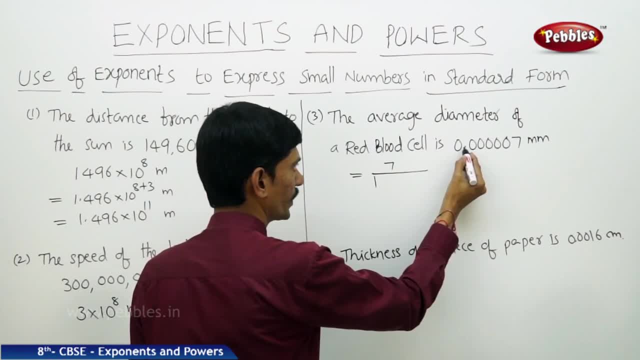 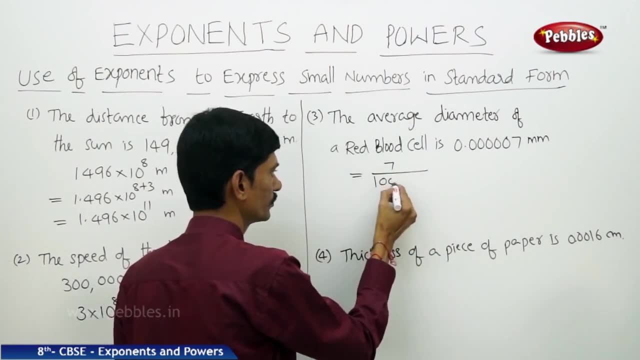 written as 7 by 1.. Now, after decimal point, how many digits are there? So 1,, 2,, 3,, 4,, 5,, 6.. So we can write 1,, 2,, 3,, 4,, 5,, 6 zeros. Now this equals to 7 by 10, to the power of 6 millimeters. Now this can. 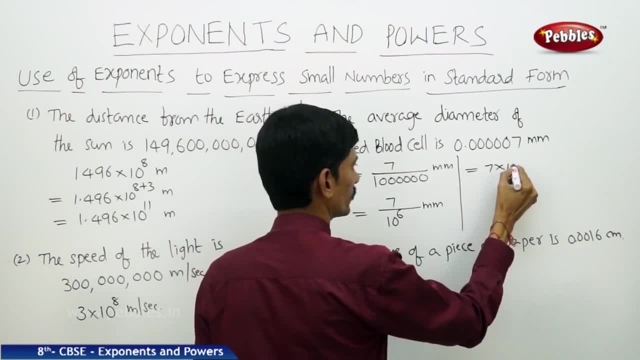 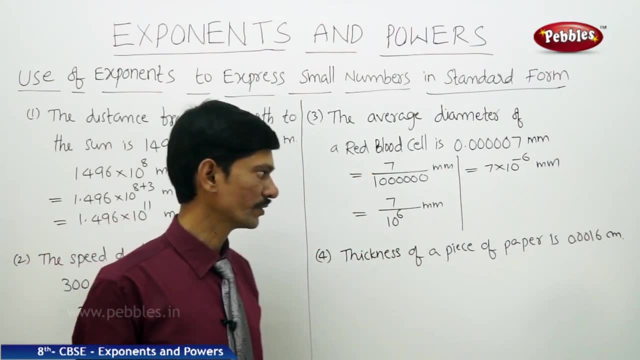 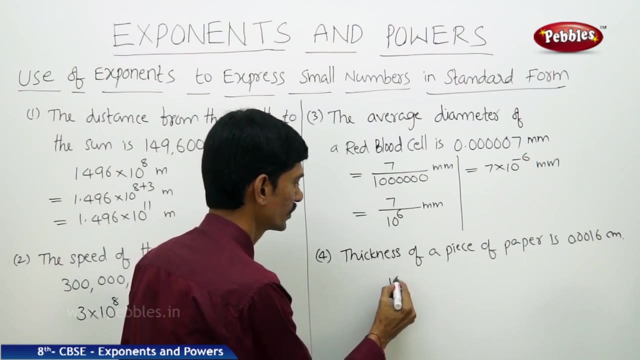 be written as 10 into 10, to the power of minus 6 millimeters. Now the next one. the thickness of a piece of paper is 0.0016 centimeters. Now this can be written as 16 by 1.. Now, after the decimal point: 1,, 2,, 3,, 4.. There are 48. So we can take 4 zeros here. 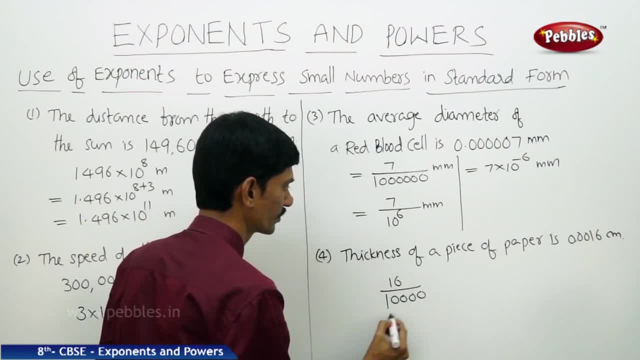 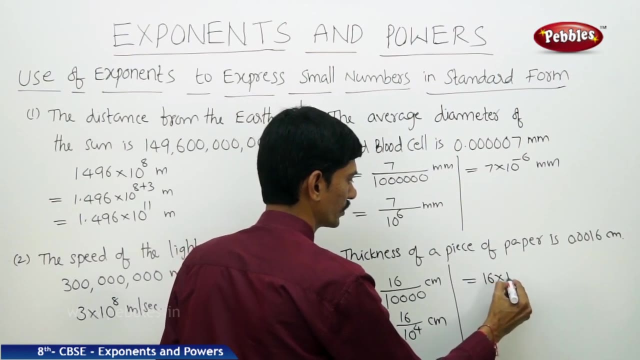 in the denominator 1,, 2,, 3,, 4 centimeters. Now this equals to 16 by 10, to the power of 4 centimeters. Now this equals to 16 into 10, to the power of minus 4 centimeters. Now we can take the. 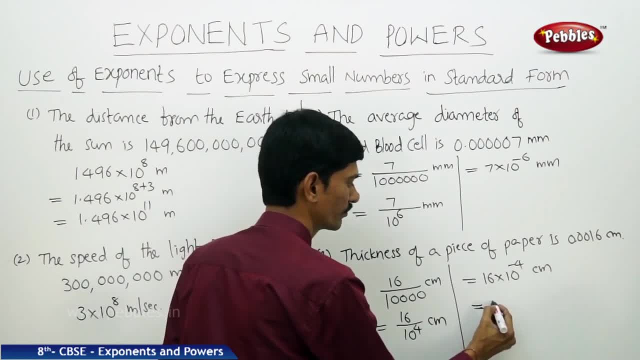 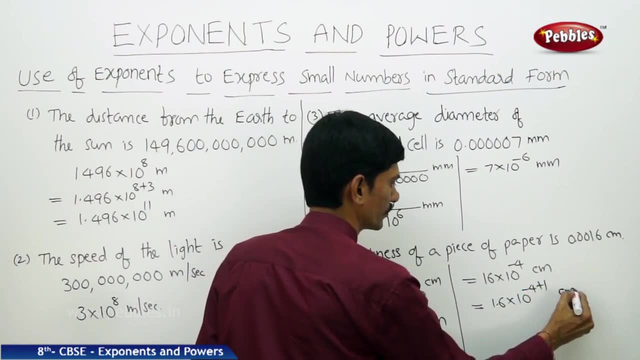 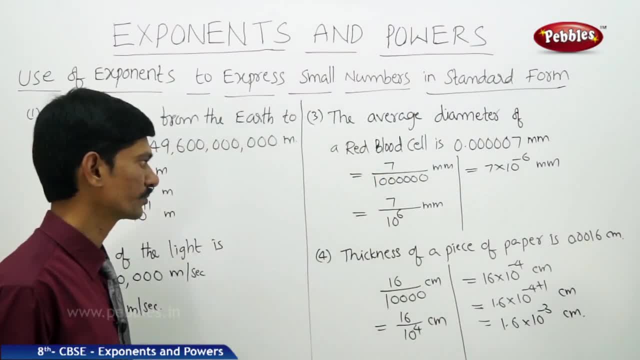 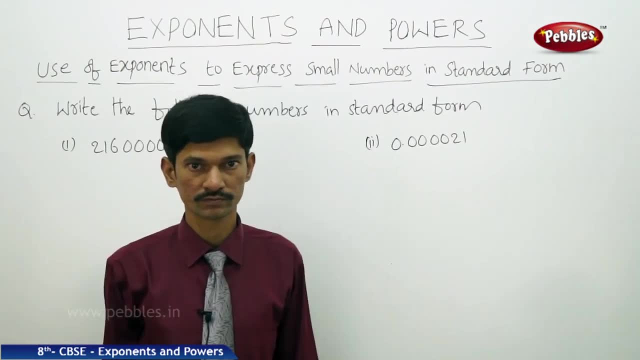 of minus 3 centimeters Now. this equals to 1.6 into 10, to the power of minus 3 centimeters Now. So we can use the exponents while expressing the large values or small values in the standard form. 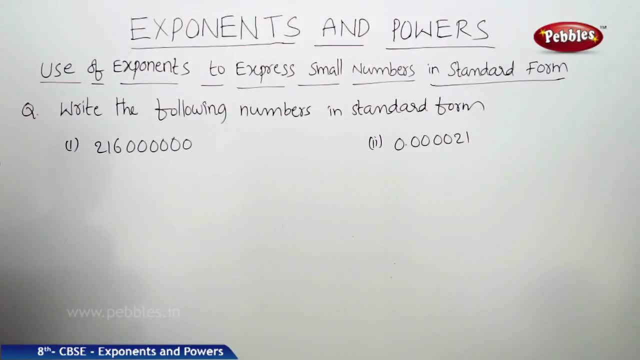 Now let us solve a problem. Write the following numbers in standard form. The first question is: see after 2,, 1,, 6, how many 0s are there? 1,, 2,, 3,, 4,, 5, 6, so? 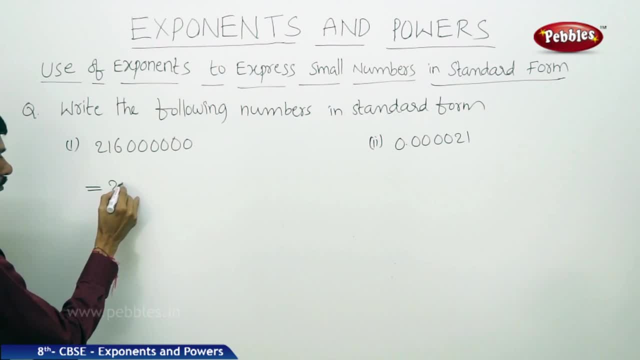 there are 6 0s now. this can be written as 2, 1, 6 into 10 to the power of 6.. Now we have to place a decimal point before 2 deeds, so this can be written as 2.16 into. 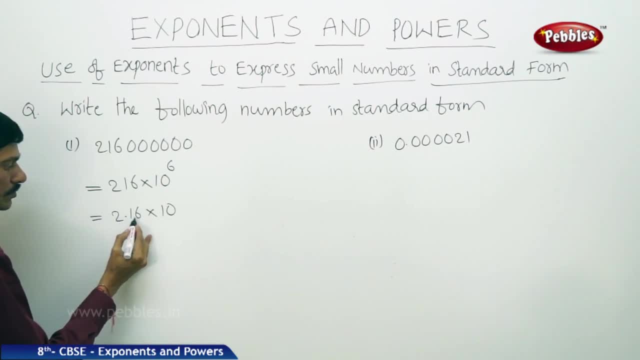 10 to the power of. here, after the decimal point, there are 2 deeds, so we should increase the exponent by 2, so 6 plus 2, now this equals to 2.16 into 10 to the power of 8.. 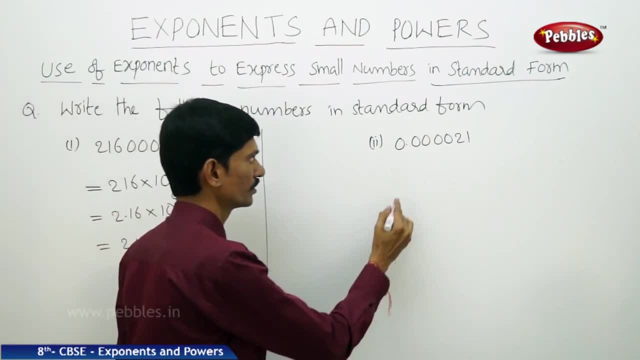 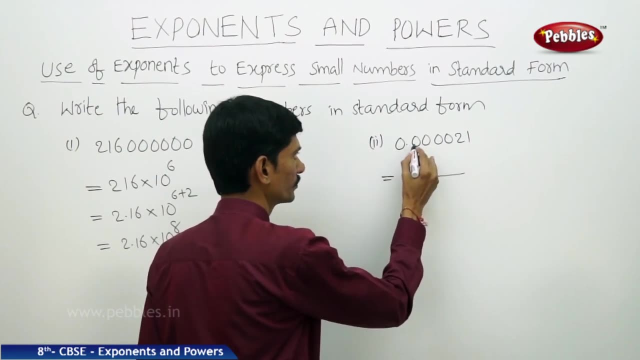 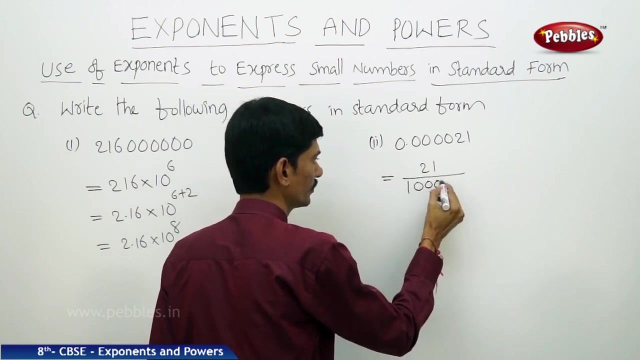 Now the second question: 0.000021, now 21 by 1, and after decimal point 1,, 2,, 3,, 4,, 5,, 6, there are 6 deeds, so we will take 6 0s here: 1, 2,, 3,, 4,, 5, 6, now this equals to: 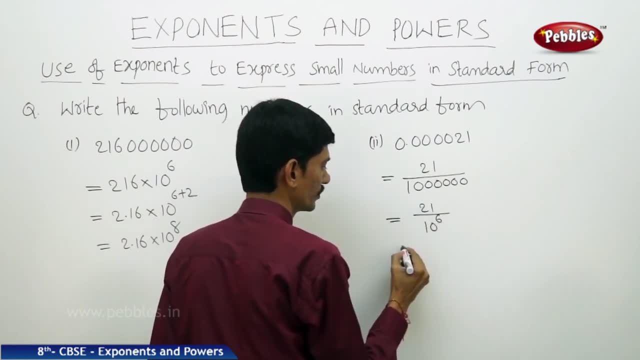 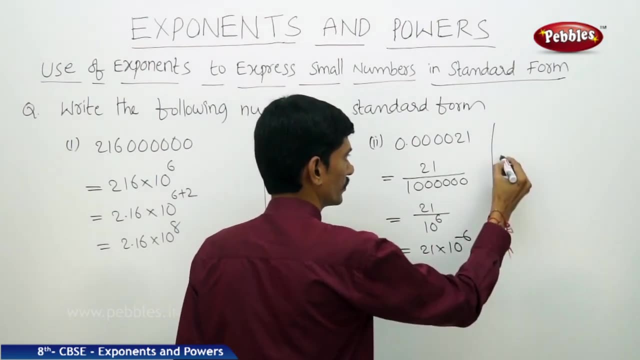 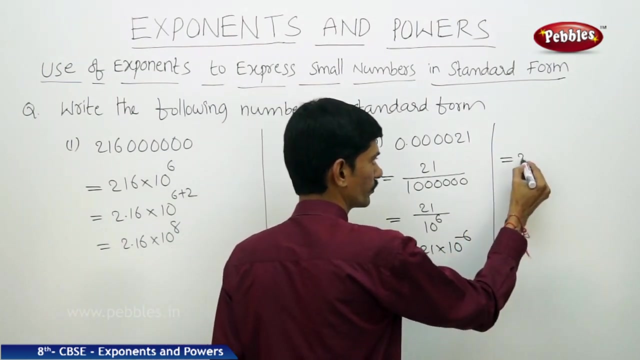 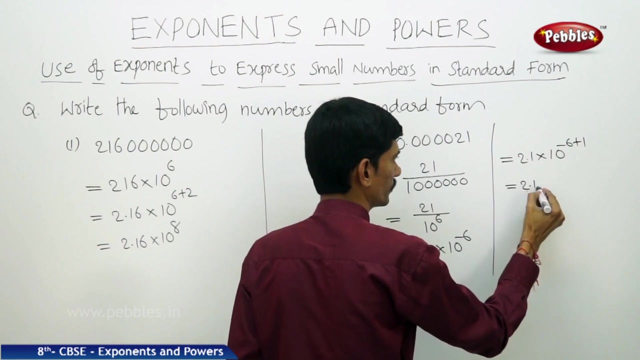 21 by 10 to the power of 6,. now this equals to 21 into 10 to the power of minus 6.. Now this equals to: now we can place decimal point before 1 digit from units. place now 2.1 into 10 to the power of minus 6 plus 1, this equals to 2.1 into 10 to the power of. 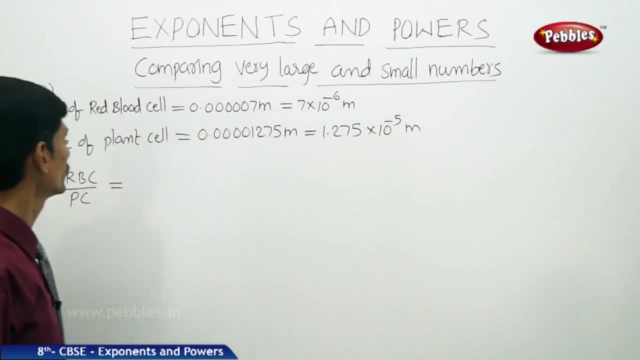 minus 5.. Now the next topic: comparing very large and small numbers. now let us take an example now. the size of red blood cell is given by 0.00001.. 0.00007 meters and the size of plant cell is given by 0.00001275 meters. 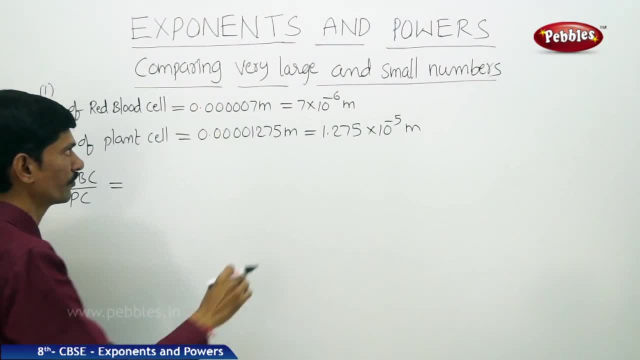 Now these 2 values can be written in the standard form as so: the size of red blood cell is written as 7 into 10, to the power of minus 6 meters, and the size of the plant cell can be written in the standard form as 1.275 into 10 to the power of minus 5 meters. 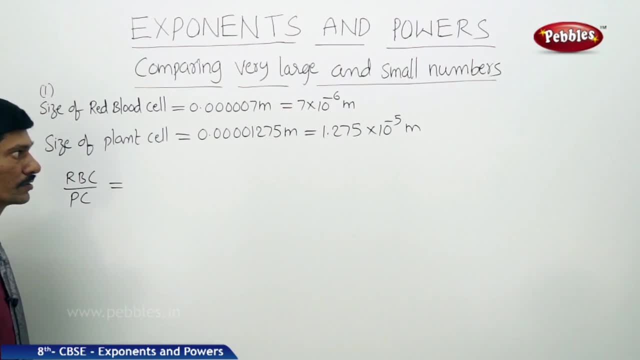 Now we will compare these 2 values. So we will take the quotient of the size of red blood cell and the size of plant cell. Now the size of red blood cell is 7 into 10 to the power of minus 6 divided by the size. 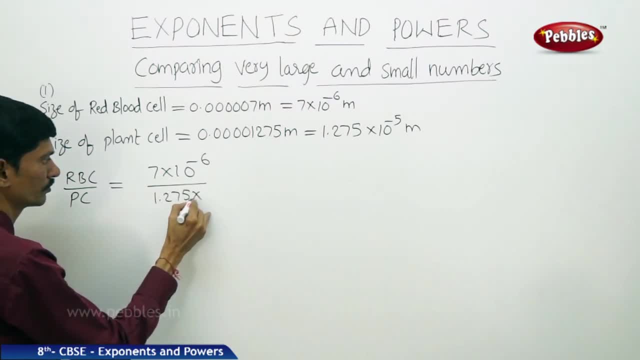 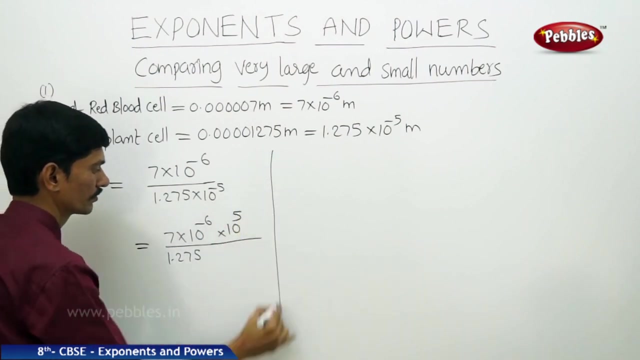 of plant cell is 1.275 into 10 to the power of minus 5.. Now this equals to 7 into 10, to the power of minus 6.. Here we are taking 2 of x and we will write it as 10 to the power of minus 6 divided by 1.275. divided by 1.275. 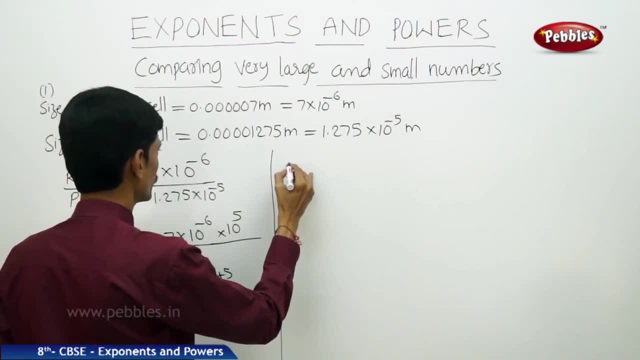 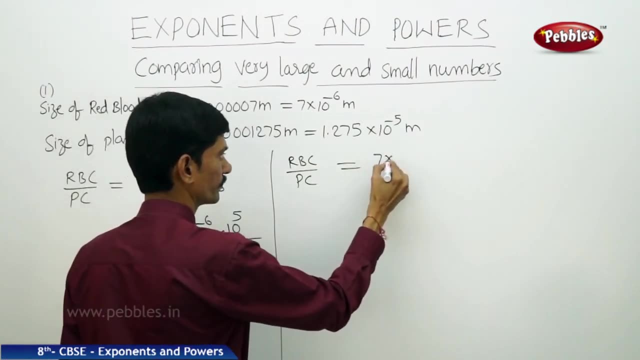 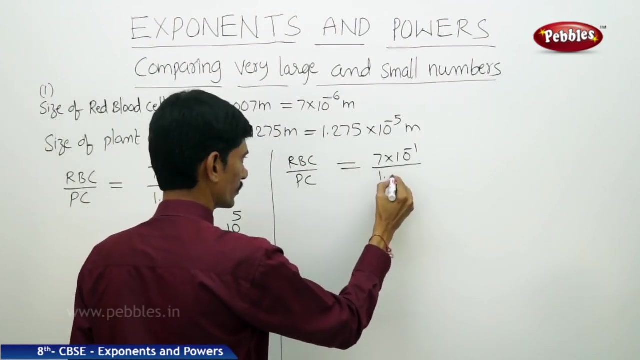 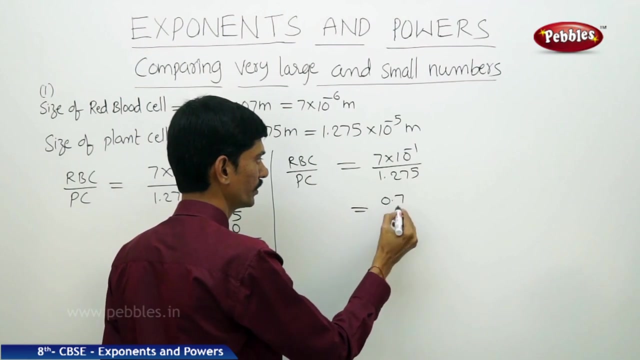 Now this equals to 7 into 10 to the power of minus 1. minus 6 plus 5 is minus 1 divided by 1.275.. So 7 into 10 to the power of minus 1 means this can be written as 0.7 divided. 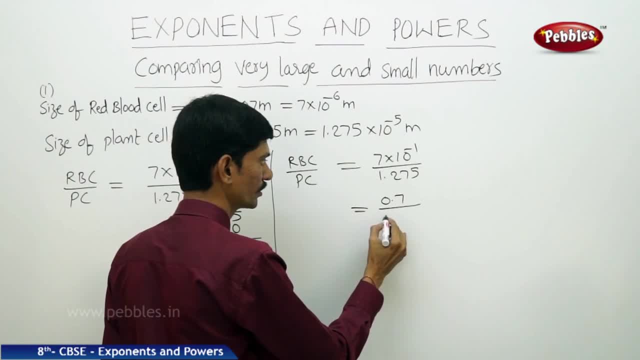 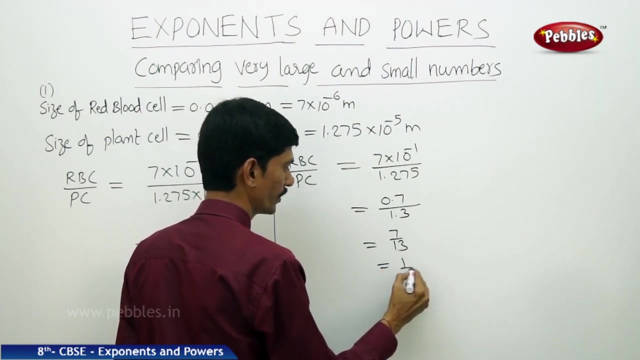 by so 1.275 is approximately equal to 1.3.. Now this equals to approximately equals to. now. here we can cancel decimal point to decimal point, and this can be written as 7 by 13.. Now this is approximately equals to 1 by 2.. Now, therefore, the size of red. 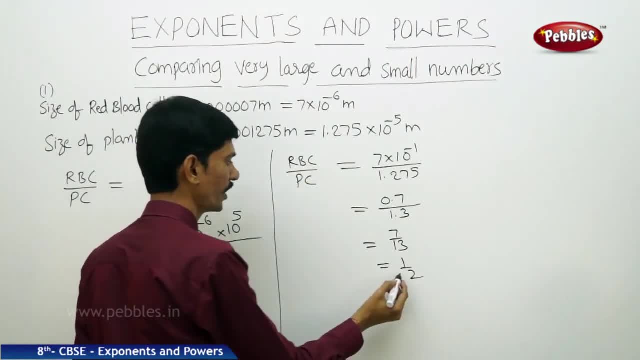 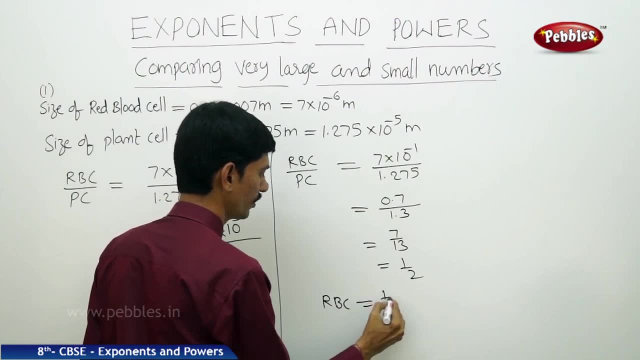 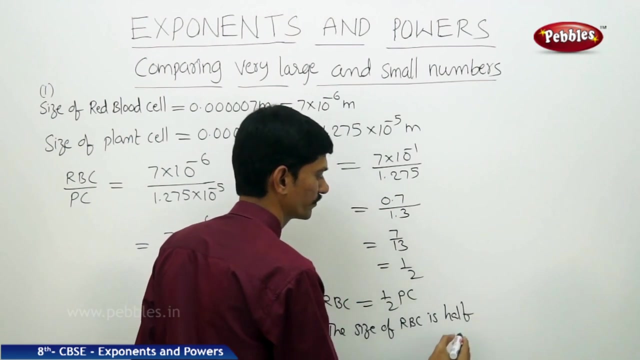 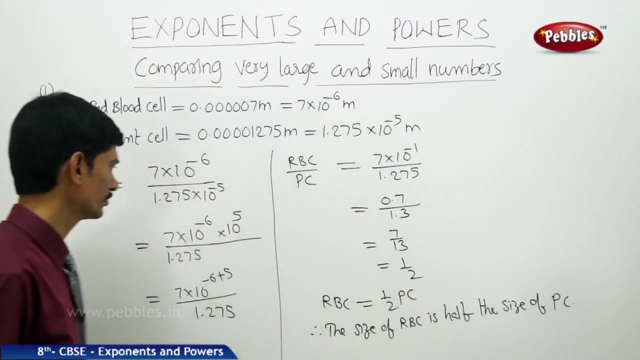 blood cell is half the size of plant cell. So here we can write that red blood cell equals to 1 by 2. So the size of plant cell equals to half plant cell. Therefore you can write that the size of red blood cell is half the size of plant cell. So by finding the ratio of 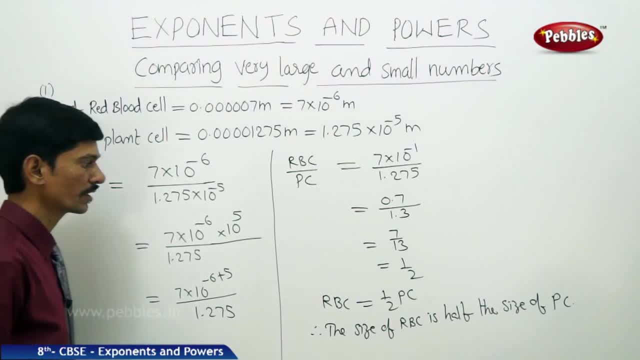 the size of the red blood cell and the plant cell. so we can compare these two. Now, here we can observe that approximately the size of plant cell is equal to 1 by 2.. Now from here we can write that the size of the red blood cell is equal to 1 by 2.. Now here we. 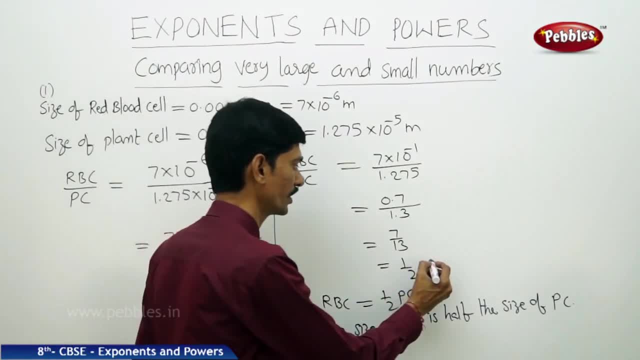 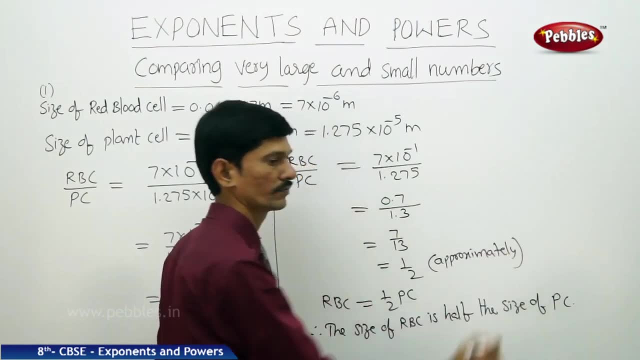 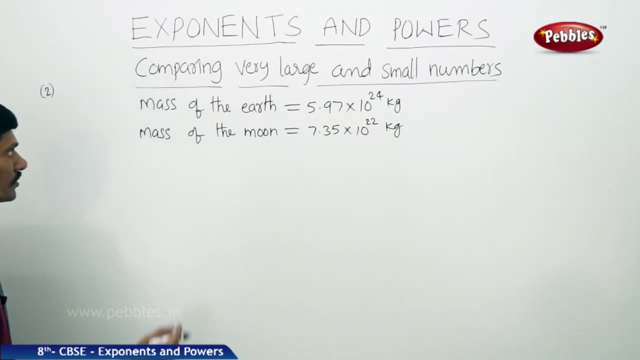 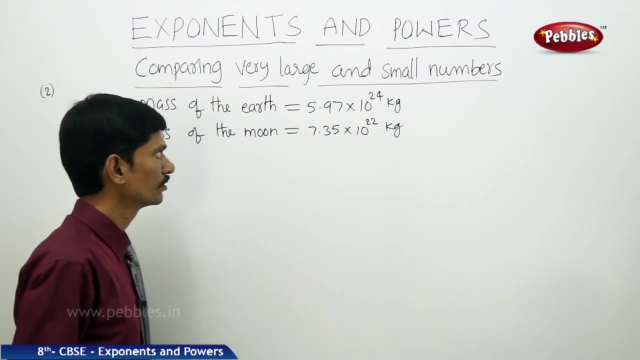 of red blood cell is half the size of plant cell, so this is approximately equal value. Now let us take another example to compare the larger numbers, using exponents. now, given that mass of the earth is 5.97 into 10, to the power of 24 kilograms, so this is a larger. 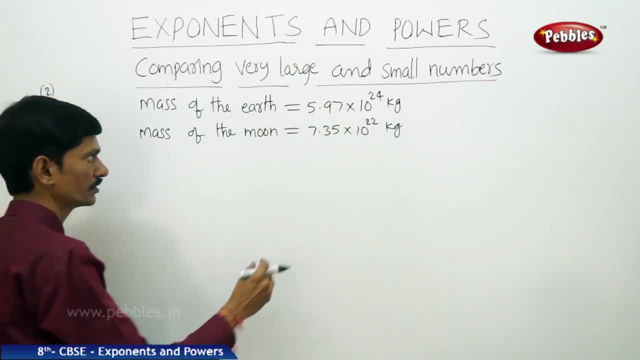 value and mass of the moon is 7.35 into 10 to the power of 22 kilograms. If you want to find the total mass- means the mass of the earth plus the mass of the moon, then you will find there is some total mass equals to mass of the earth plus mass of the. 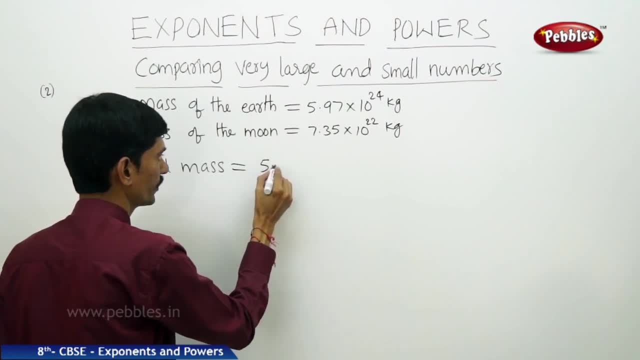 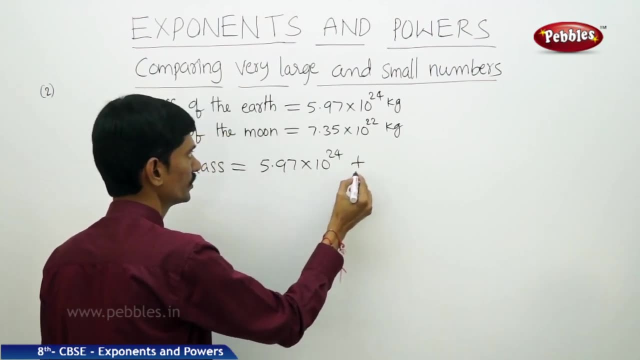 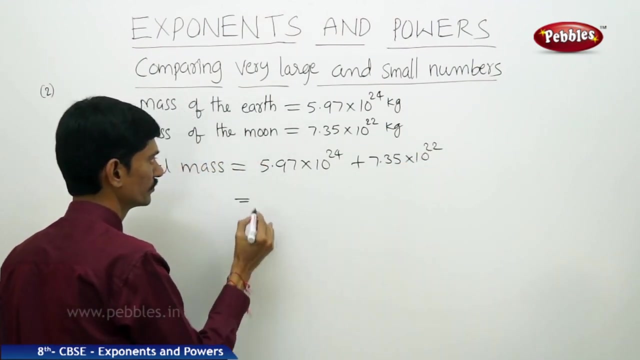 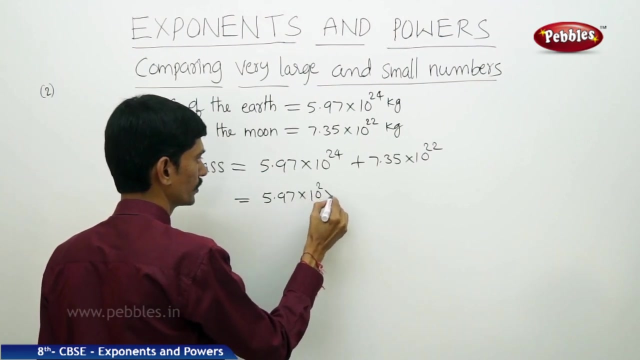 moon. so mass of the earth is given that 5.97 into 10 to the power of 24 kilograms. The mass of the moon is 7.35 into 10 to the power of 22 kilograms. Now this equals to 5.97 into 10 to the power of 24 kilograms. can be written as 10 square. 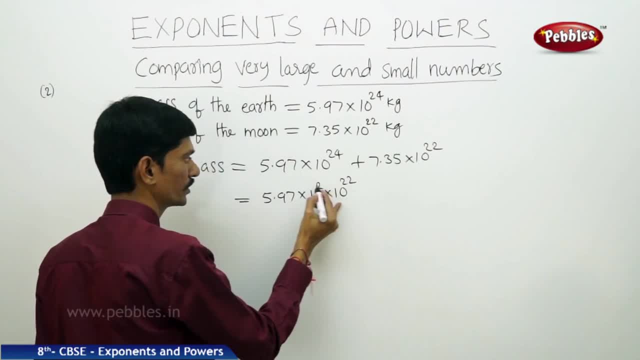 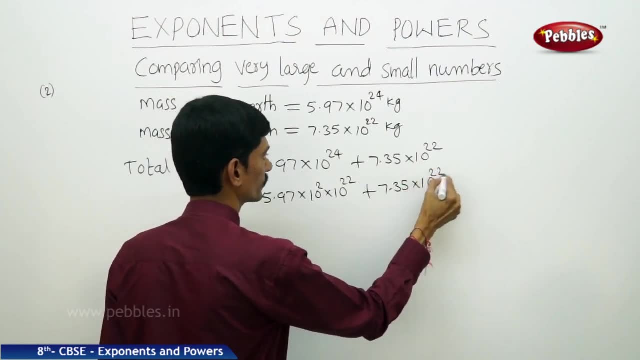 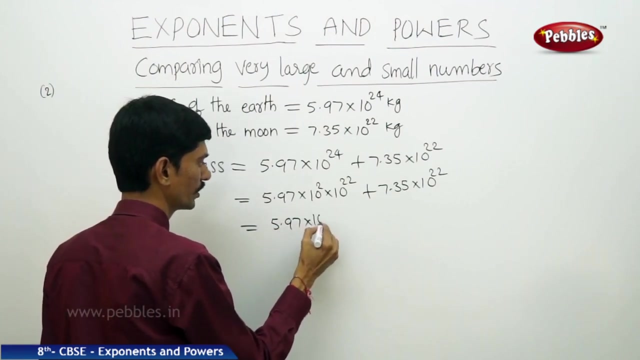 into 10 to the power of 22 kilograms. so here, 22 plus 2 is 24 plus 7.35 into 10 to the power of 22 kilograms. This equals to 5.97 into 10. square means 100 into 10 to the power of 22 plus 7.35 into. 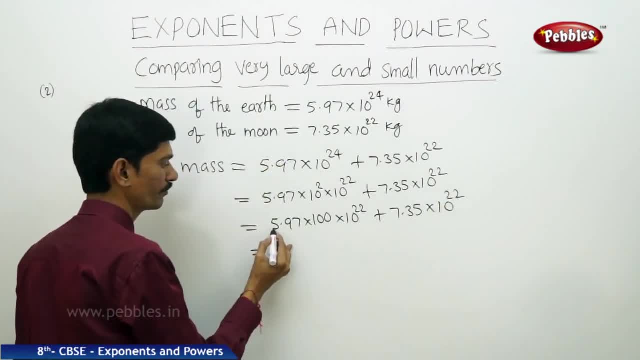 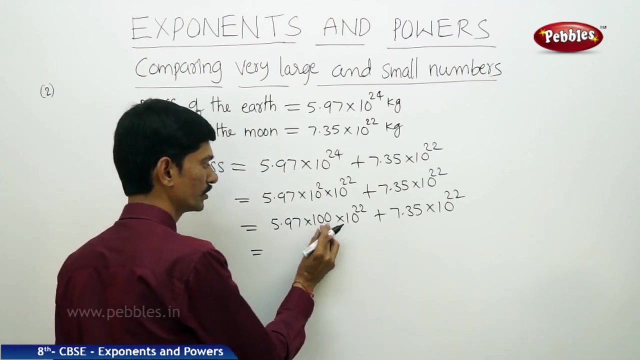 10 to the power of 22.. Now 5.97 into 100. so when you multiply a decimal number by 10,, 100 or 1000, then decimal point will move 2 digits if it is multiplied by 100. Because there are two zeros in the number. 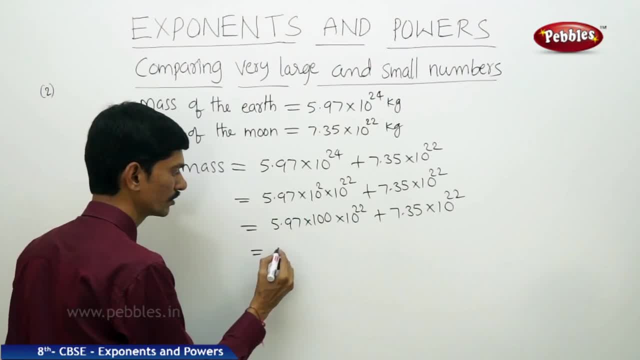 It will move 2 digits right. so here Meth is equal to 5. 90, 7. shared with 2, here give the 1.. Now, if you are interested in tens of Pang, so this means that we had taken packet 7 of. 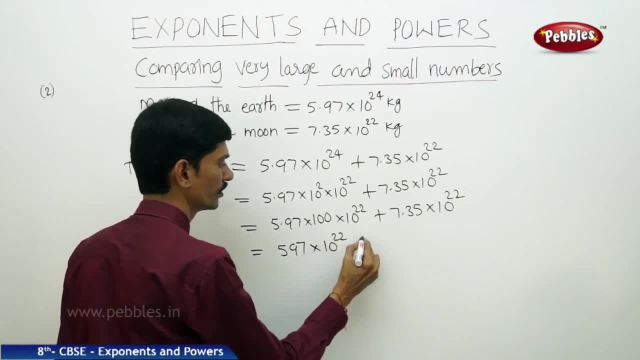 7 kahla of사� Francis for zero, that is 9.. How a number. so it will move 2 days. right now this becomes 5.. 97 point zero means 597 into 10 to the power of 22, plus 7.35 into 10 to the power of 22.. 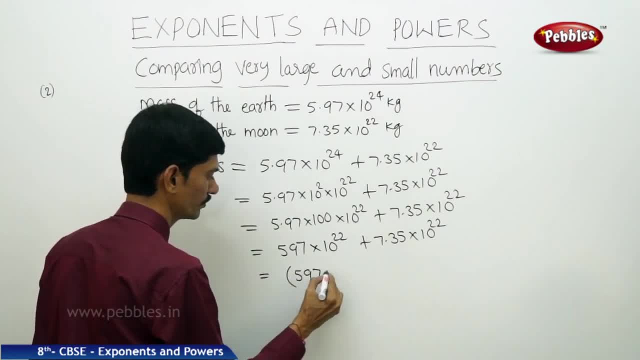 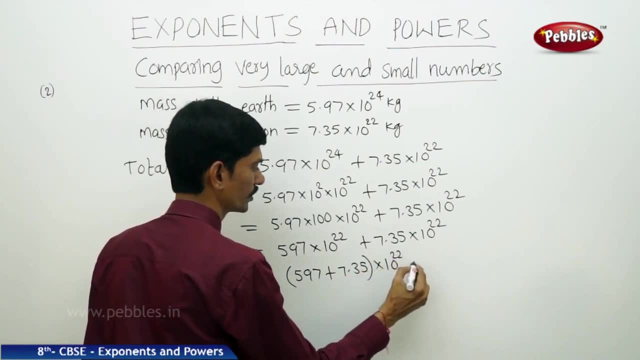 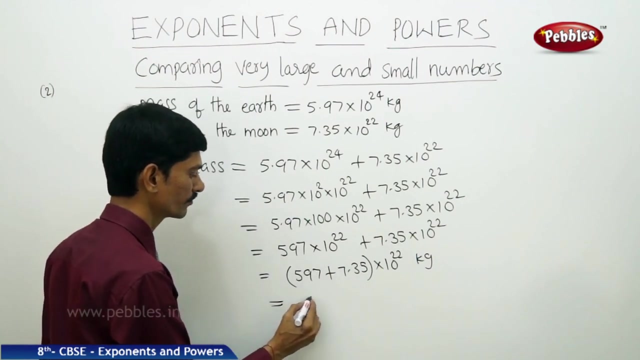 Now here we can take 10 to the power of 22 come in, So then we get 597 plus 7, .3, and All 10 to the power of 22 kilograms. Now this equals to 597 plus 7, 604.35, into 10 to the power of 22 kilograms. 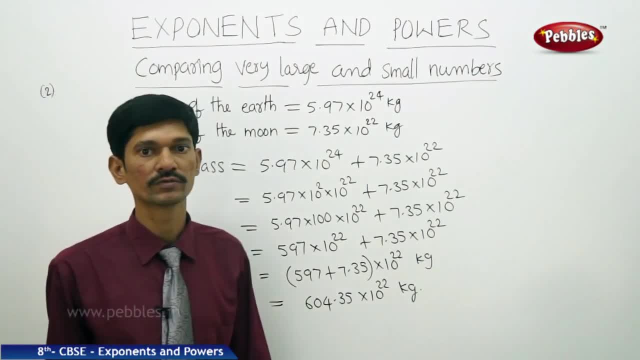 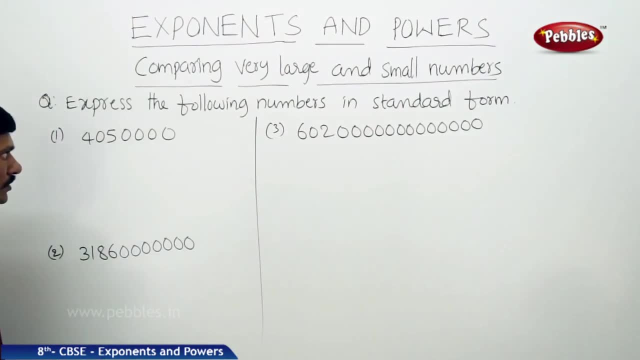 So this is the total mass of the earth and the moon. Now let us solve few problems. Express the following numbers in standard form. So here the larger numbers are given, So very large numbers. we have to write So these numbers in the standard form. 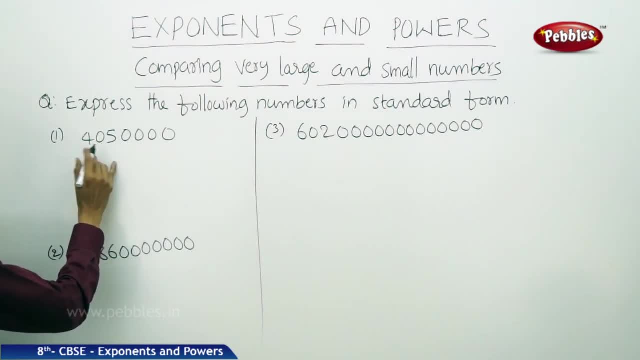 Now the first question is 405.. After 405, there are 4 zeros. Now this can be written as 405 into 10, to the power of. So here 1,, 2,, 3, 4 zeros are there. 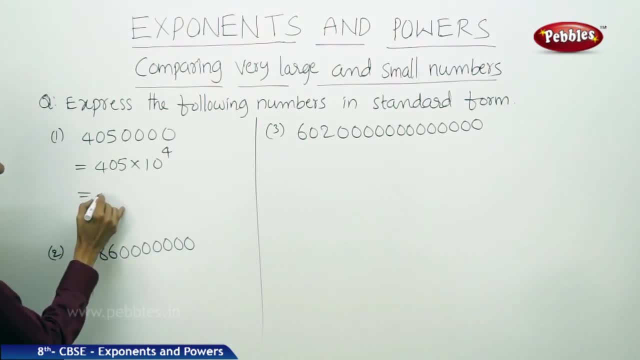 So we can write 10 to the power of 4.. Now this equals to: Now we have to put the decimal point before 2 digits from units, place So 1, 2.. So this can be written as 4.05 into 10 to the power of 4.. 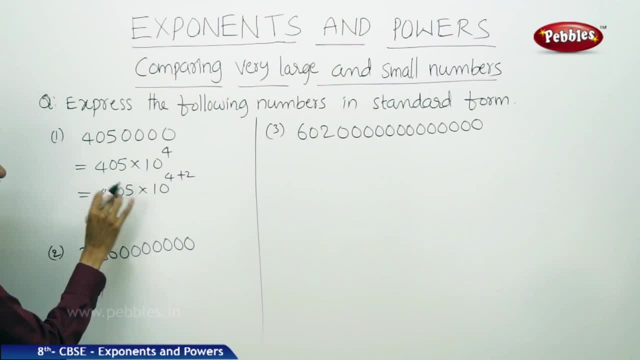 So plus 2, because there are 2 digits after decimal point, So we have to write plus 2 in the exponent. Now this equals to 4.05 into 10, to the power of 4 plus 2 is 6.. 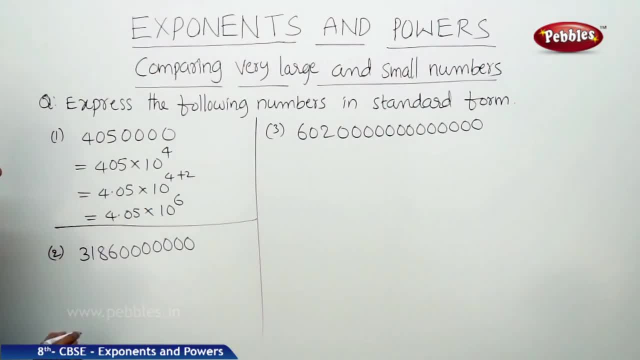 Now, this is the standard form of the given number. Next, 3186.. So after 3186, let us count how many zeros are there: 1, 2,, 3,, 4,, 5, 6, 7.. 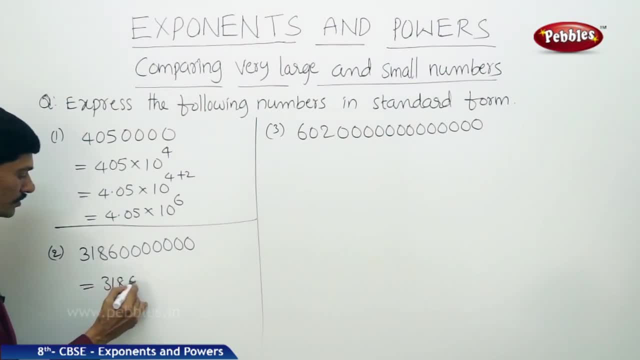 Now this equals to 3186.. Now this equals to 3186 into 10, to the power of 7.. Now this equals to: So 1,, 2,, 3.. Before 3 digits we have to take the decimal point. 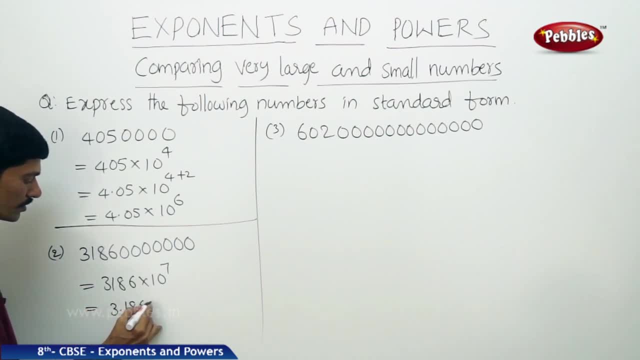 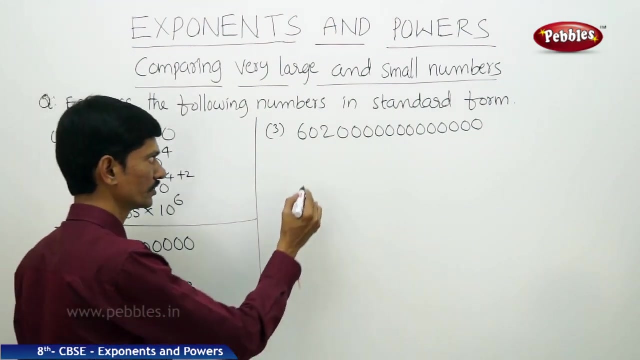 Now this can be written as 3.186 into 10 to the power of 7 plus 3.. This equals to 3.186 into 10 to the power of 7 plus 3 is 10.. Now next question. 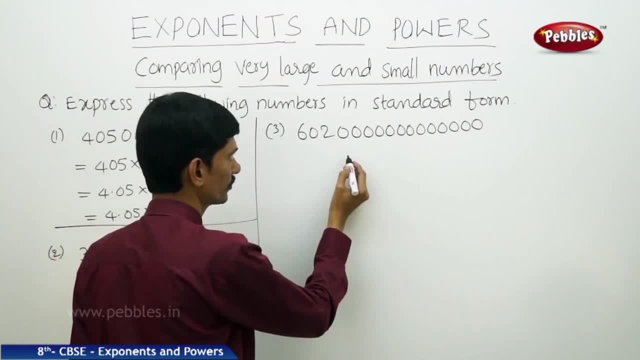 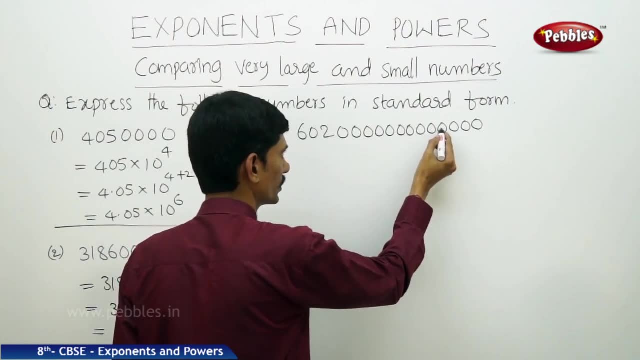 602.. After 602, how many zeros are there? So let us count the number of zeros Now: 1, 2, 3, 4,, 5,, 6,, 7,, 8,, 9,, 10,, 11,, 12,, 13.. 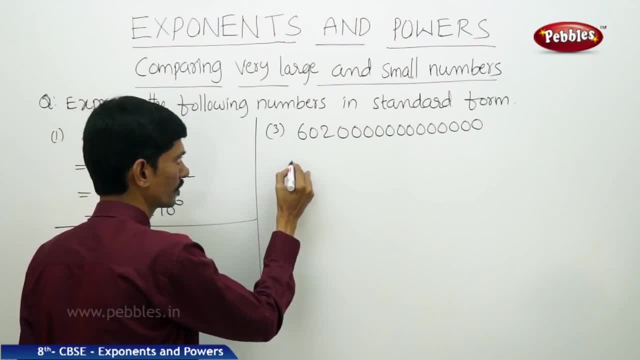 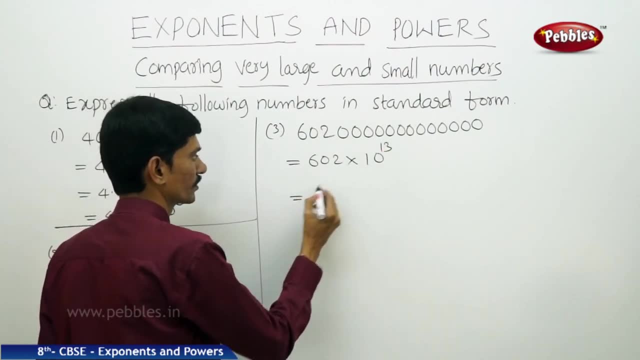 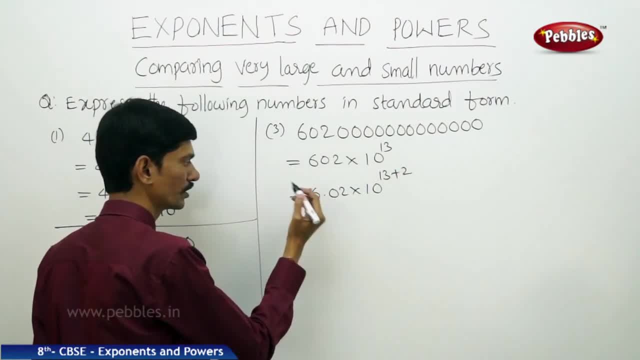 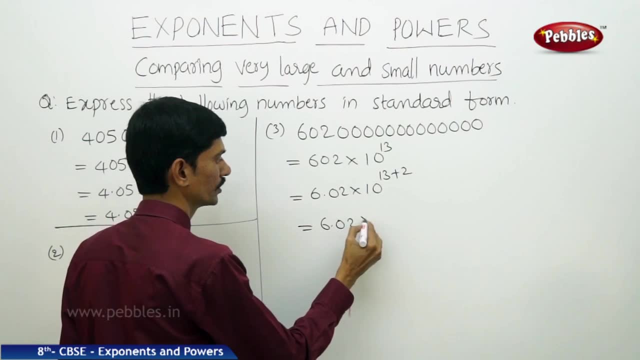 Now this equals to 6.02 into 10, to the power of 13 plus 3.. So as there are 2 digits after the decimal point, So we have to take plus 2 in the exponent. Now this equals to 6.02 into 10, to the power of 13, plus 2 is 15.. 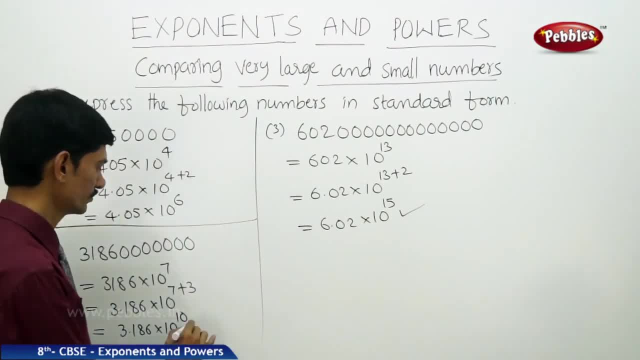 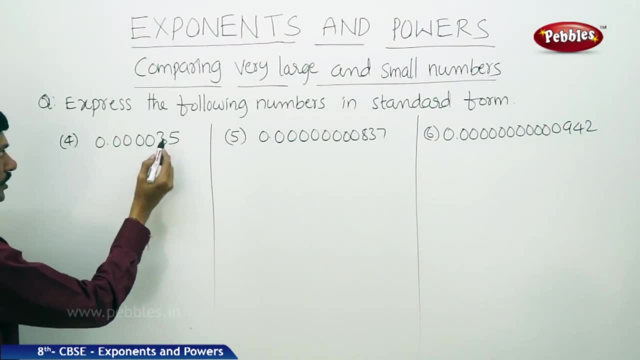 Now, this is the standard form of the given large value. Now we will take fourth question: 0.000035.. So we have to express this in the standard form. But this is very small value, because So it is in the decimal form. 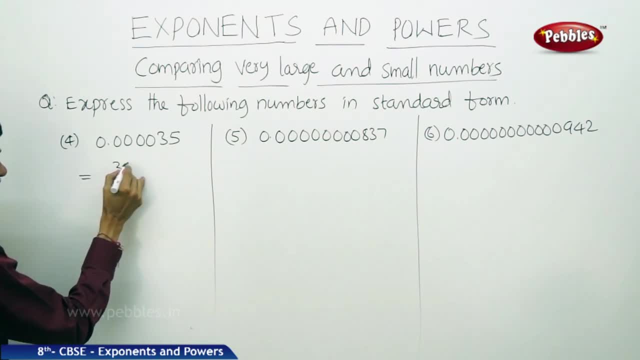 Now this equals to- We can write this in the fraction form: 35 by So, 1 after decimal point. How many digits are there? 1,, 2,, 3, 4, 5, 6.. So we can write 10 to the power of 6.. 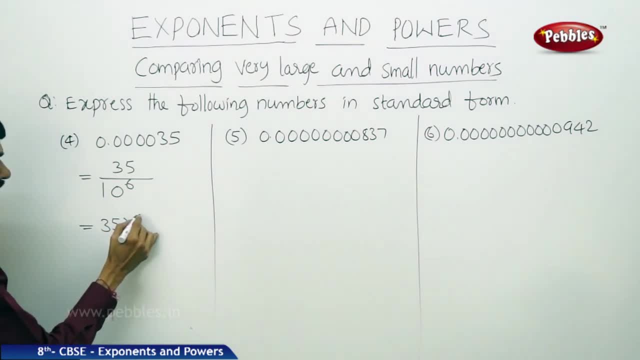 Now this can be written as 35 into 10 to the power of minus 6.. So this can be written using the loss of exponents. Now this equals to: Now we have to place the decimal point before 1 digit. 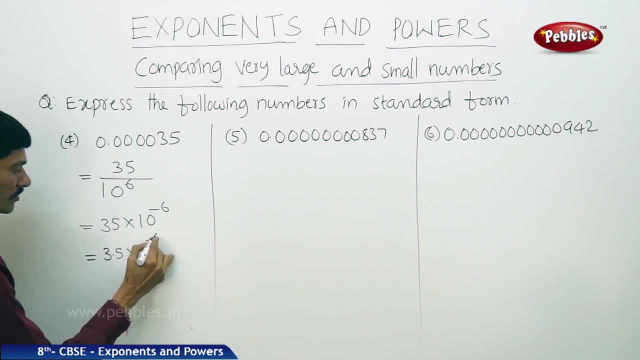 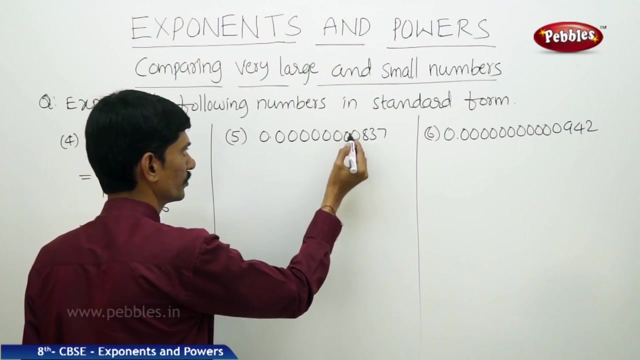 Now 3.5 into 10 to the power of minus 6 plus 1. This equals to 3.5 into 10 to the power of minus 5.. Now fifth question: 0.00000000837.. 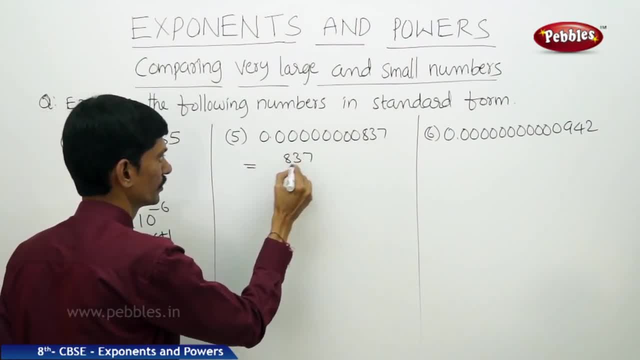 Now this equals to 837 by. So we write in the fraction. Now, after decimal point, how many digits are there? So 1, 2, 3, 4,, 5, 6, 7, 8,, 9,, 10,, 11.. 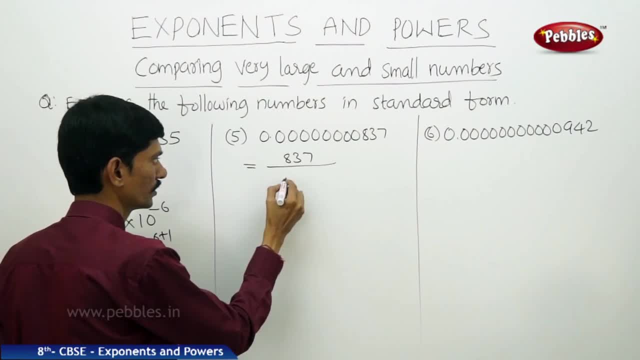 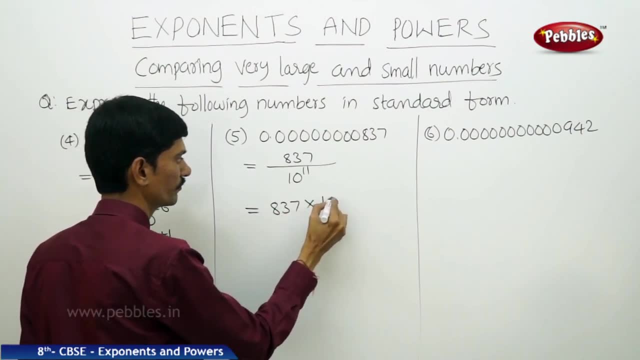 So there are 11 digits after decimal point, So we can write 10 to the power of 11.. Now this can be written as 837 into 10 to the power of minus 11.. Now this equals to 8.37 into 10 to the power of minus 11.. 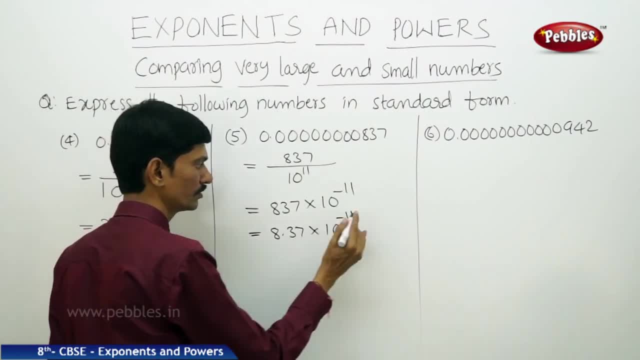 1. So after decimal point there are 2 deeds. So we have to take plus 2 in the exponent. Now this equals to 8.37 into 10, to the power of minus 11. plus 2 is minus 9.. Now this is: 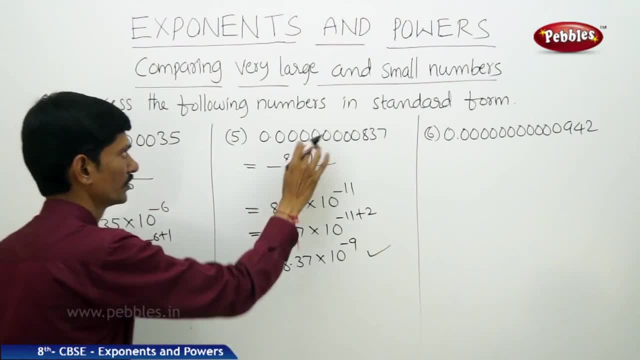 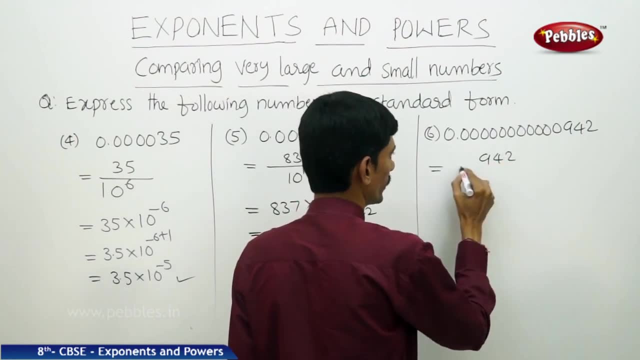 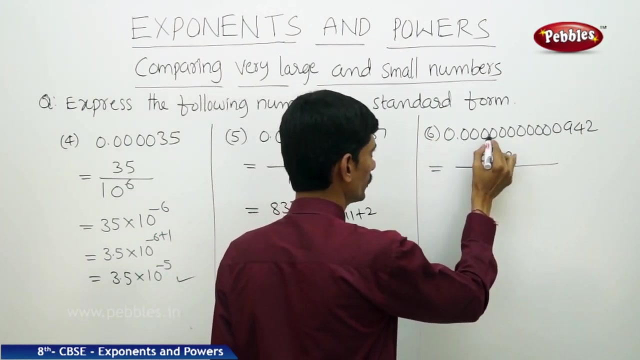 the standard form of the given decimal number. Next sixth question: Now, this equals to 942 divided by Now, how many deeds are there after decimal point 1,, 2,, 3,, 4,, 5,, 6,, 7,, 8,? 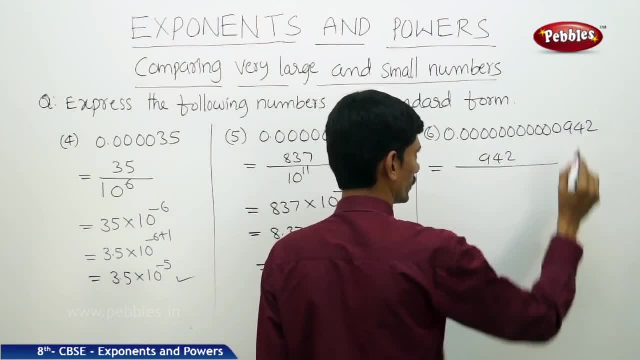 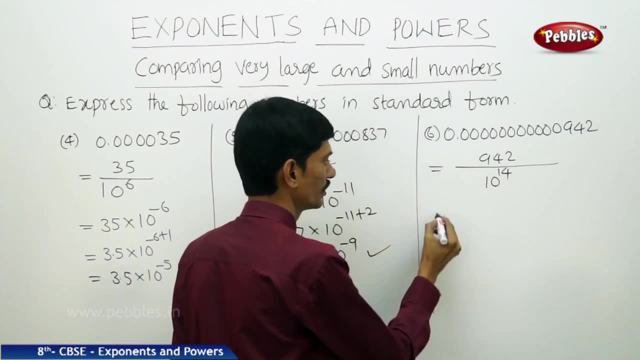 9,, 10,, 11,, 12,, 13,, 14.. So there are 14 deeds after decimal point. So we will take 10 to the power of 14 in the denominator. Now this equals to 942 into 10 to the power of minus. 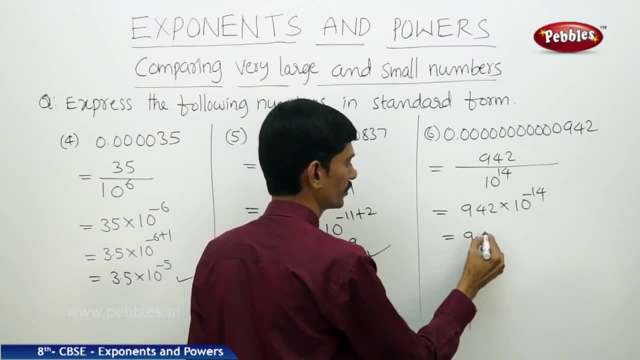 14. Now this equals to 9.42 into 10, to the power of minus 14 plus 2, because after decimal point there are 2 deeds, So we have to take here plus 2 in the exponent. Now this equals to: 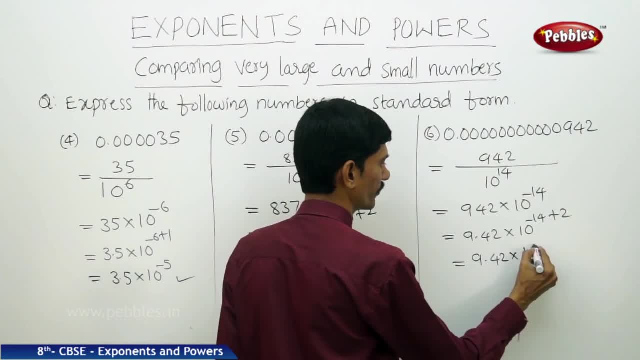 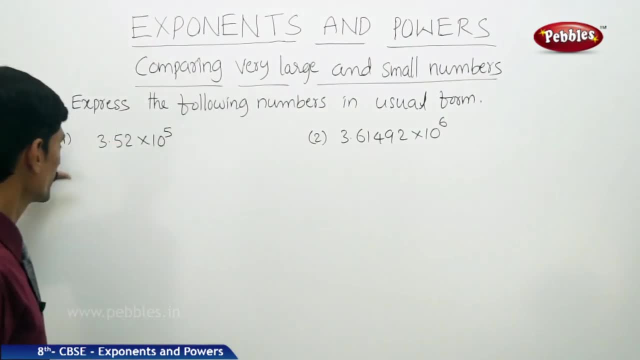 9.42 into 10 to the power of minus 12.. Now, this is the standard form of given decimal number. Now let us solve the next question. Express the following numbers in usual form. Now, just before you have expressed, 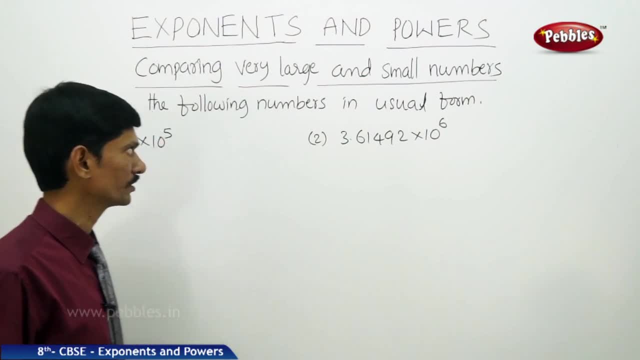 Now the given numbers in the standard form. Now we have to express. Now the standard forms are given, We have to express these standard forms in our usual form. Now, the first question is: 3.52 into 10 to the power of 5.. So, as we know that this is larger value, 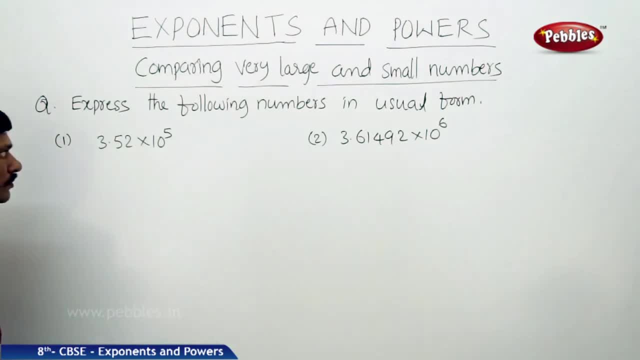 because the exponent of the 10 is positive number, So it is a larger value. We should express this in our usual form. Now this equals to: Now we should remove the decimal point, So 352.. So 352.. 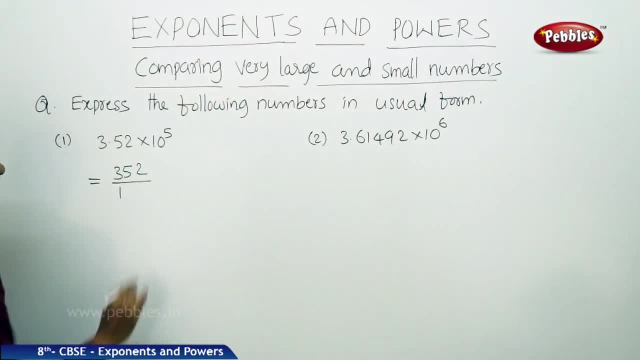 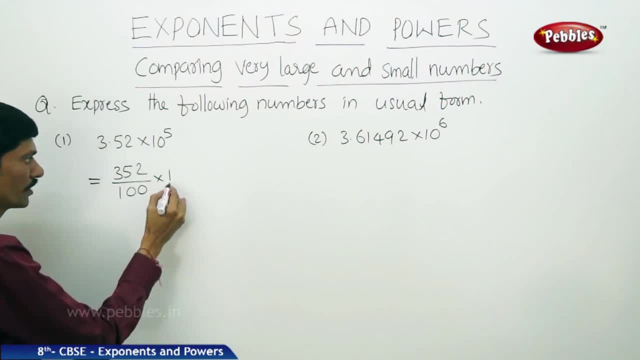 into 10 to the power of 5 means after 1, you should take 1,, 2,, 3,, 4, 5 zeros. Now here we can cancel 2 zeros Here. 2 zeros Now this equals to 352 into 1000.. Now this equals. 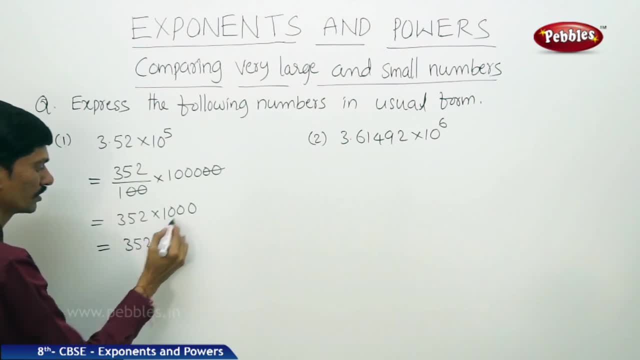 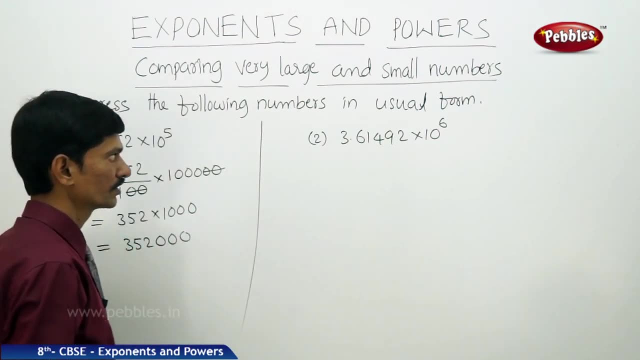 to 352 ones are 352.. And there are 3 zeros. Now this equals to 352 into 1000.. Now this three zeros, Now this is 3,52,000.. Now the second question: 3.61492 into 10 to the power. 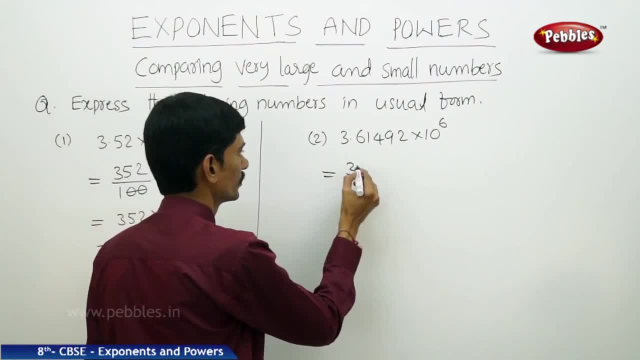 of 6.. Now this equals to 361492 divided by. so write 1 here. Then how many deeds are there after decimal point? 1,, 2,, 3,, 4, 5.. So we take 5 zeros- 1,, 2,, 3,, 4, 5- into 10. 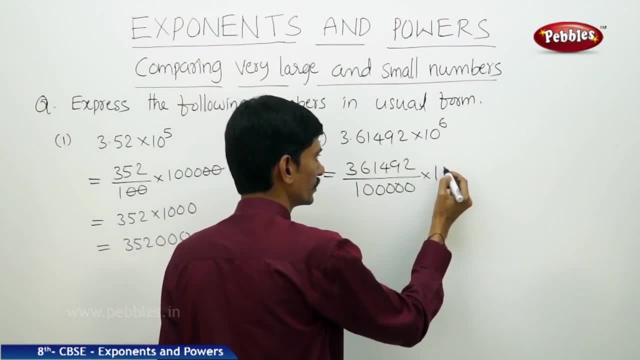 to the power of 6 means after 1, we should take 6 zeros: 1,, 2,, 3,, 4,, 5, 6.. So we can cancel 5 zeros and here 5 zeros and 1 zero is left in the numerator. Now this equals: 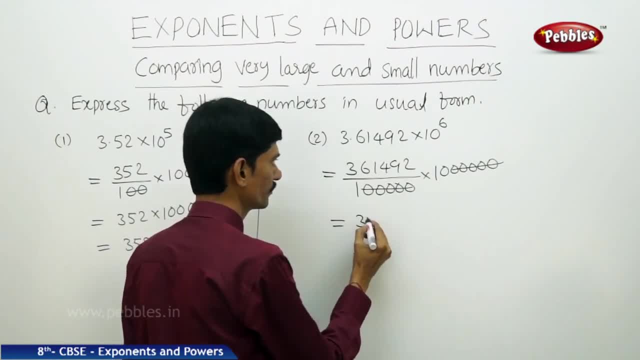 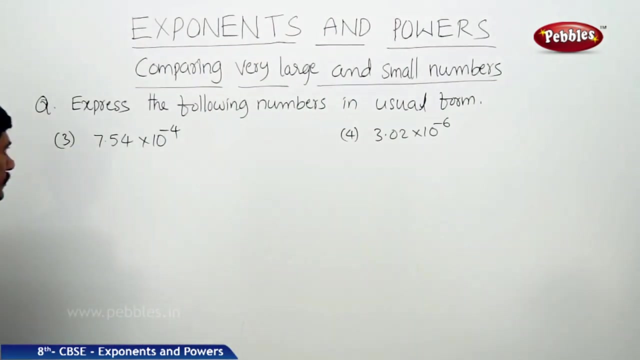 to 361492.. Now this equals to 361492.. Now let us solve third problem: 7.54 into 10, to the power of minus 4.. So when you observe the exponent of 10, it is negative number. So we can understand. 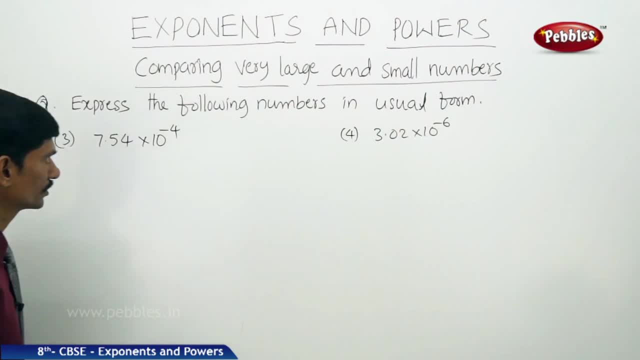 that it is very small value. Now we should express in our usual form. Now the standard form is given. Now this equals to 7.54. into 10 to the power of 6.. Now this equals to 7.54.. So when the power 10 to the power of minus 4 comes to the denominator, it becomes: 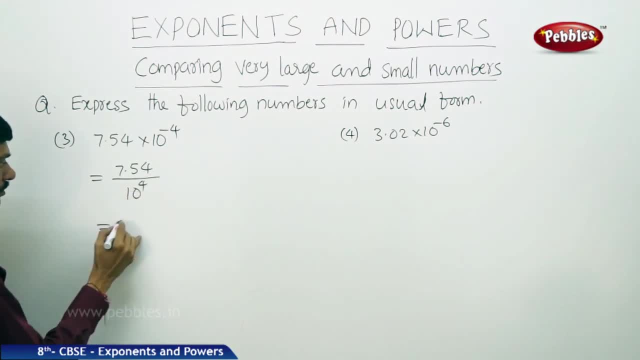 10 to the power of 4.. Now this equals to 7.54 divided by so. 10 to the power of 4 means, after 1, we should take 4 zeros: 1,, 2,, 3, 4.. So this is 10000.. So when you divide a, 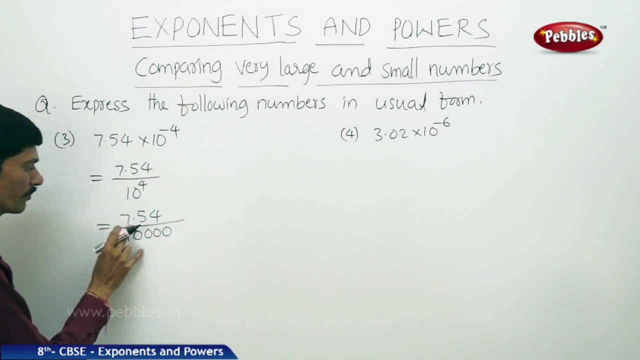 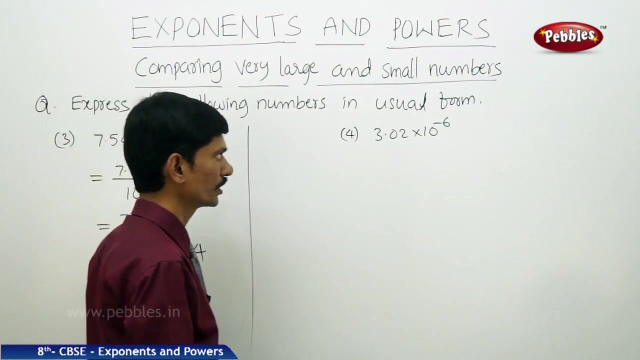 decimal number by 10000, then decimal point will move 4 digits left, then 0 point, So only 1 digit is there, 7.. So then we need to take more three zeros-1,, 2, 3 zeros, then 7,, 5,, 4.. Next 3.02 into 10, to the power of minus 6.. Now 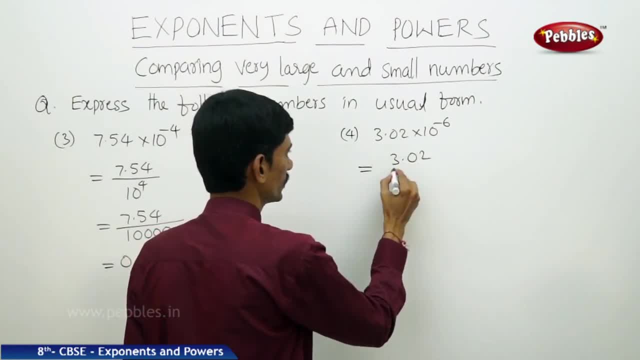 this can be written as: 3.02 divided by 10 to the power of 6.. Now this equals to 33.7, 13.3.. So this is 10 to the power of 6.. Now this equals to 34.33.. Now this equals to 32.3 into. 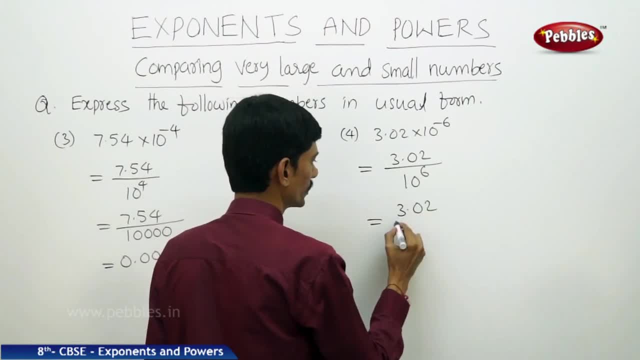 10 to the power of 6.. This is actually not equal to 0.. No, that is. So. the formula is: 3.02 divided by 10 to the power of 6 means after 1,. how many 0s we have to take here? 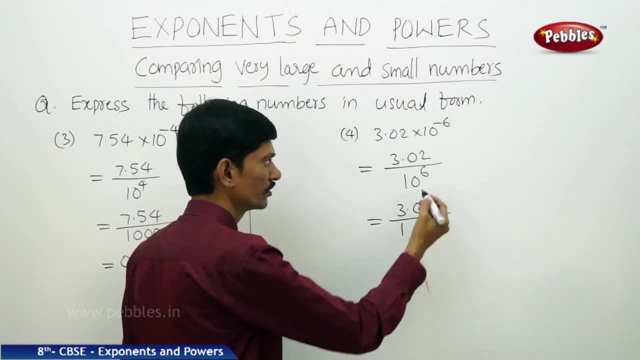 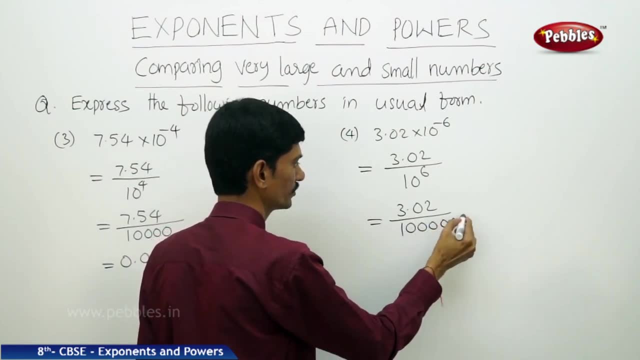 So that is based on the exponent of 10.. So exponent of 10 is 6.. So you should take 6 0s after 1.. 1,, 2,, 3,, 4,, 5,, 6.. 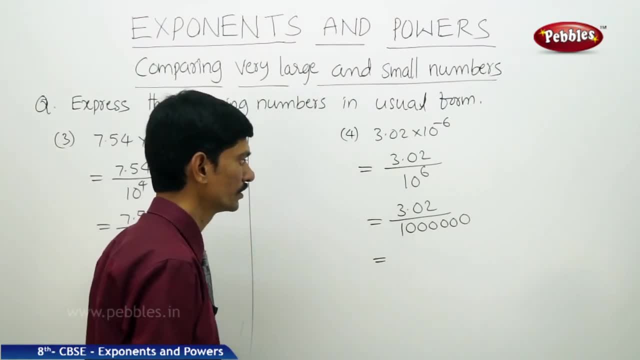 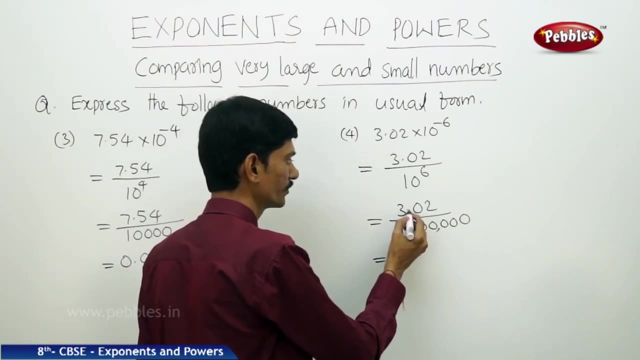 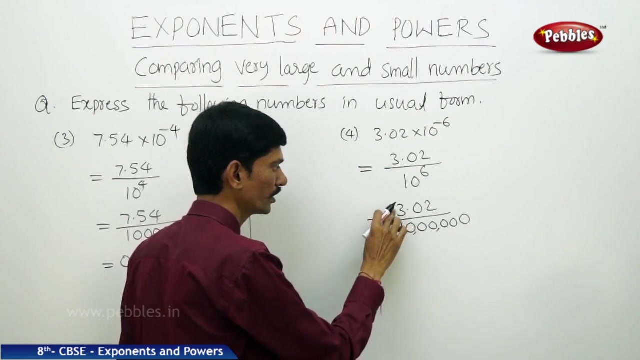 Now, when you divide 3.02 by 10 lakh, then the decimal point will be shifted to 1,, 2,, 3,, 4,, 5, 6 digits left side. So only 1 digit, 3, is there. 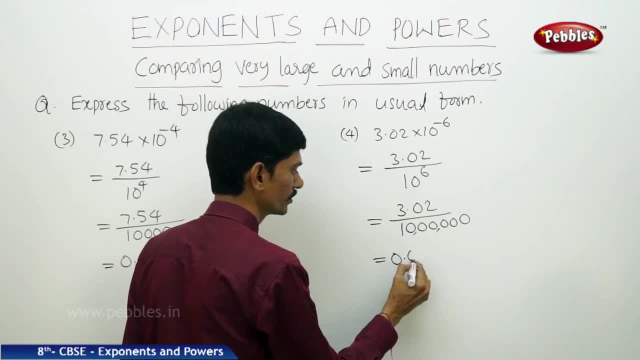 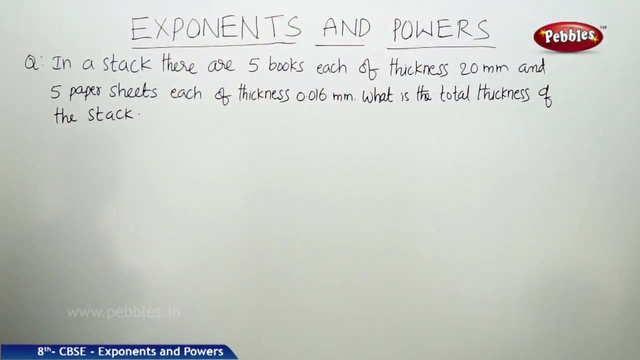 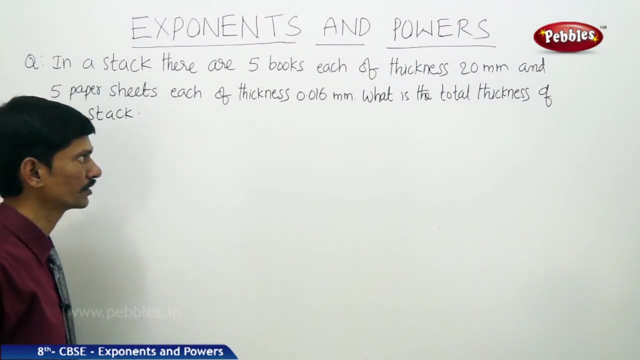 So we should take 5: 0s, 0.00000302.. Now, this is the usual form, And this is the standard form. Now let us solve a problem. In a stack, there are 5 books, each of thickness 20 millimeters, and 5 paper sheets each of thickness 0.016 millimeters. 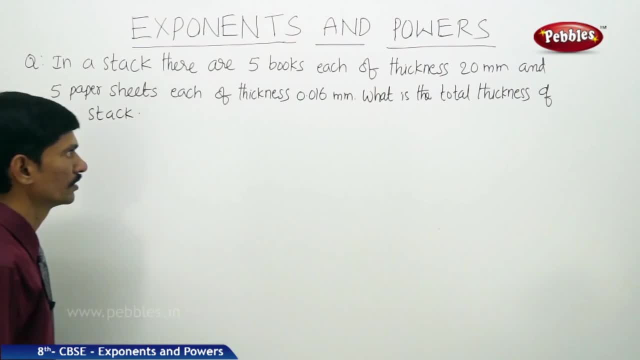 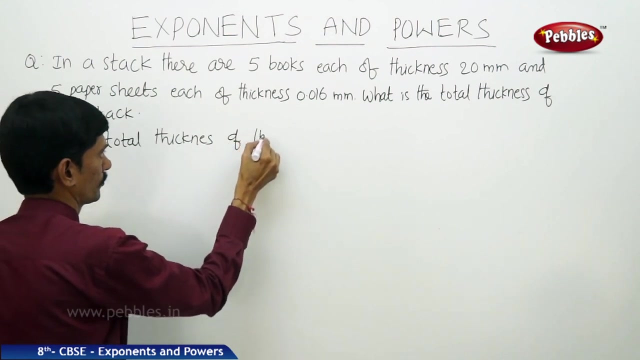 Then what is the total thickness of the stack? So this can be done using the exponents and using the standard forms. Now let us solve the total thickness of the stack: 2,, 3,, 4,, 5,, 6,, 6, and so on. 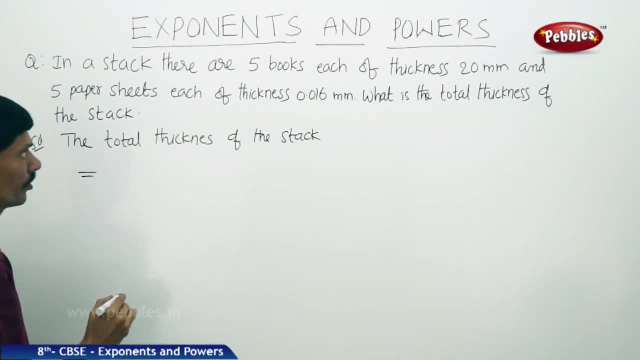 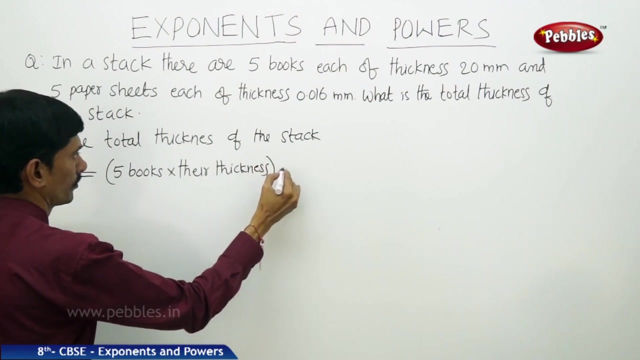 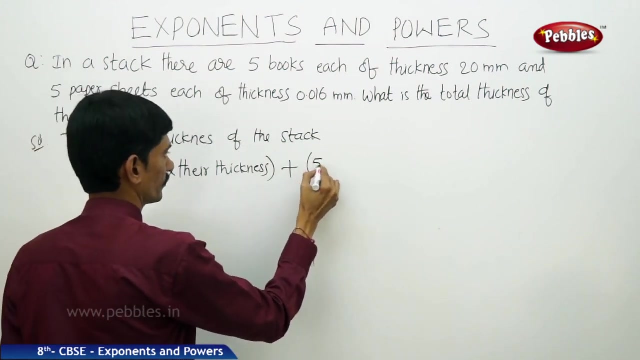 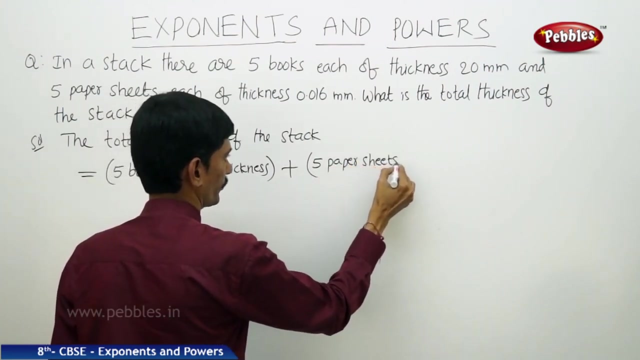 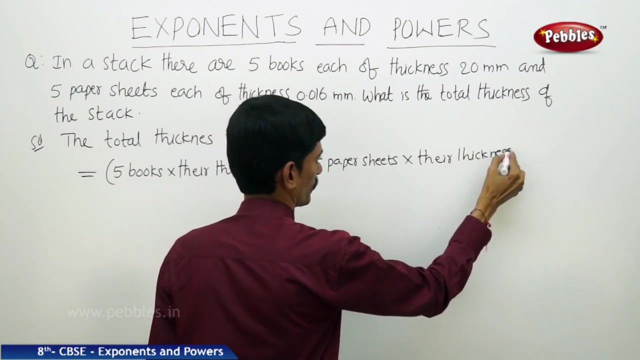 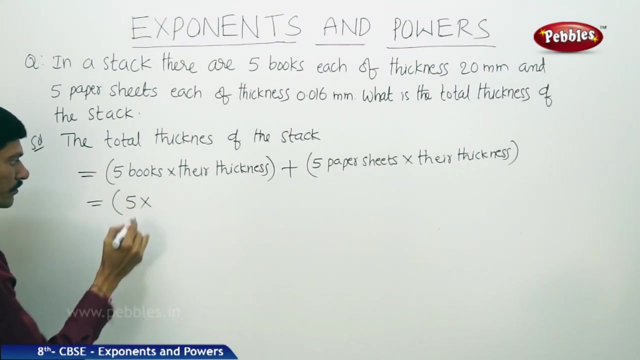 Equals to: Now how many books are there? So 5 books into their thickness plus five paper sheets and their thickness, five paper sheets into their thickness. now this equals to: so there are five books of five. the number of books: 5 into what is the thickness of each book. so that is 20 millimeters. so